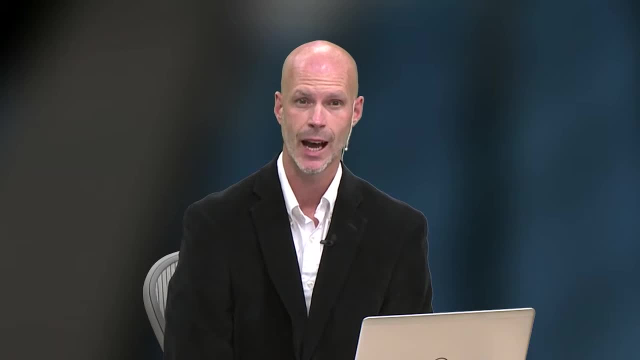 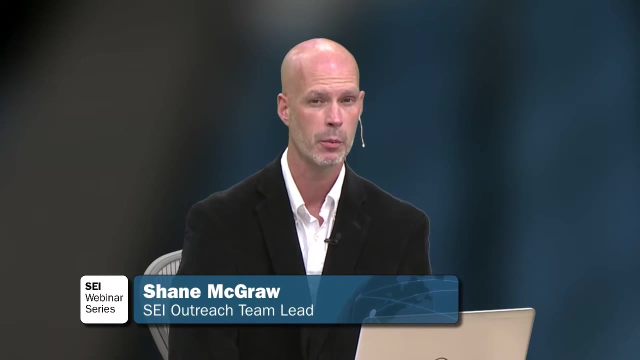 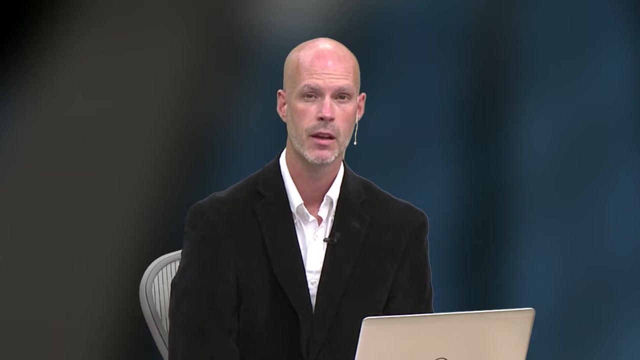 My name is Shane McGraw, your moderator for the presentation, and I'd like to thank you for attending. We want to make today as interactive as possible, so we will address questions throughout the presentation and again at the end of the presentation. You can submit those questions to our event staff at any time by using the Ask a Question tab or the Chat tab on your control panel. 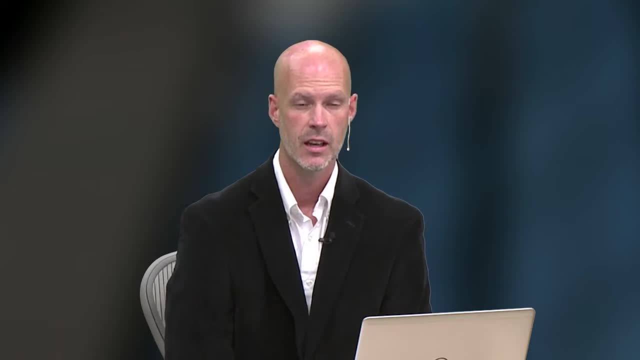 We will also ask a few polling questions throughout the presentation and they will appear as a pop-up window on your screen. The first question I'd like to ask- and it will appear now- is: how did you hear of today's event? Another three tabs I'd like to point out are the Download Materials, Twitter and Survey tabs. 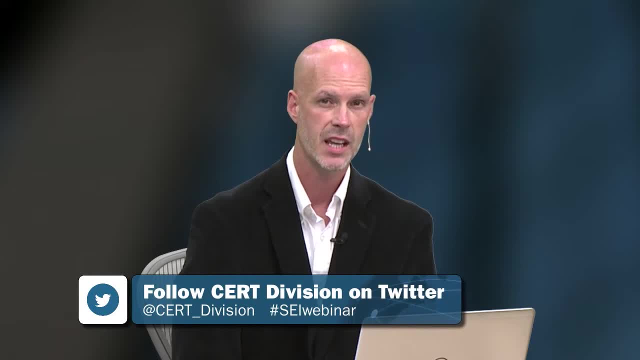 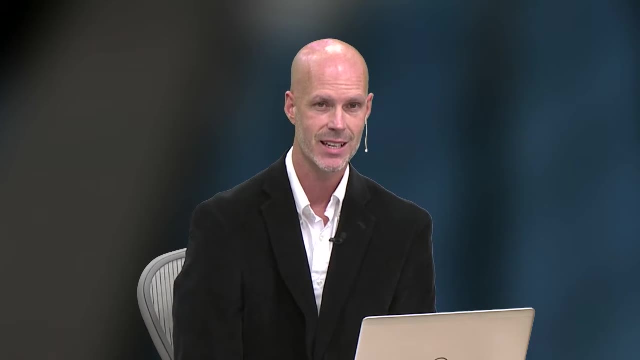 The Download Materials tab is the most important one. The Download Materials tab is the most important one. The Download Materials tab has a PDF copy of the presentation slides there now, along with other secure coding-related work and resources from the SEI. For those of you using Twitter, be sure to follow at CERT underscore division and use the hashtag SEIwebinar. 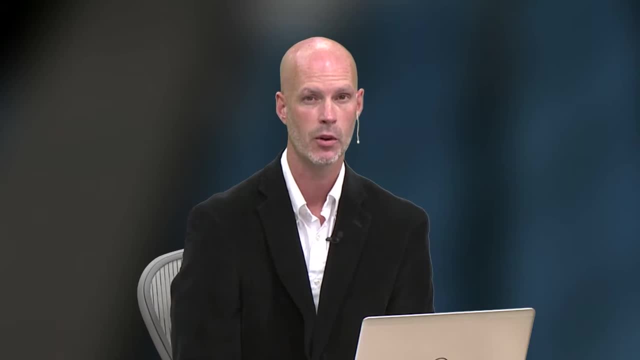 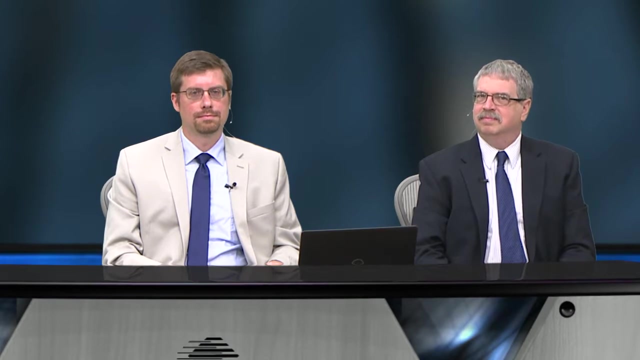 The survey we ask that you fill out upon the completion of today's webinar, as your feedback is always greatly appreciated. Now I'd like to introduce our presenters for today. Bob Shiela is the Technical Manager leading the Secure Coding Team in the Cyber Security Foundations Directorate in the CERT Division. 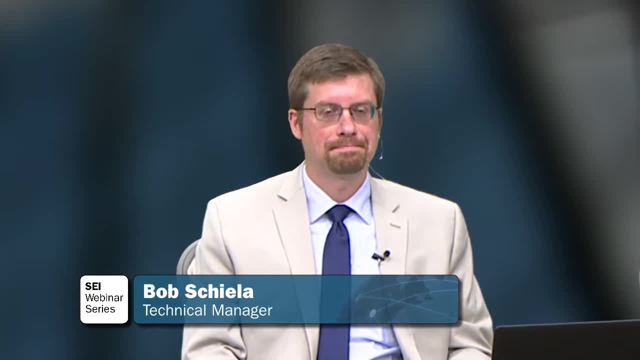 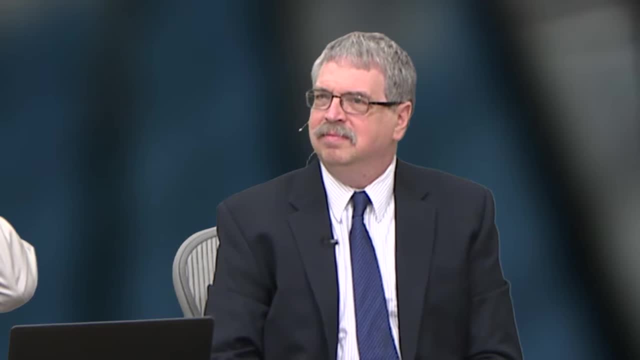 Dr Mark Sherman is the Technical Director for the Cyber Security Foundations Group and, before coming to CERT, Dr Sherman was at IBM and various startups. Welcome, Bob Mark, all yours. Thank you very much, Shane. It's a pleasure to be here and hello to everyone out in the web. 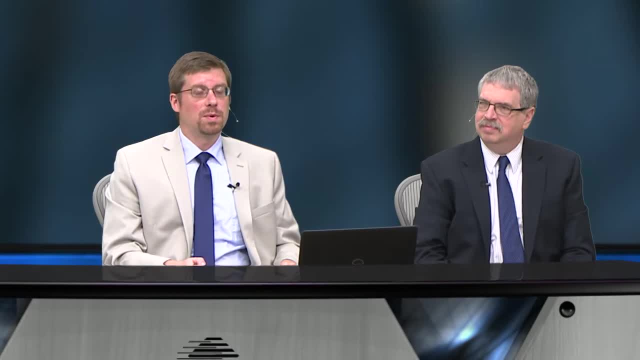 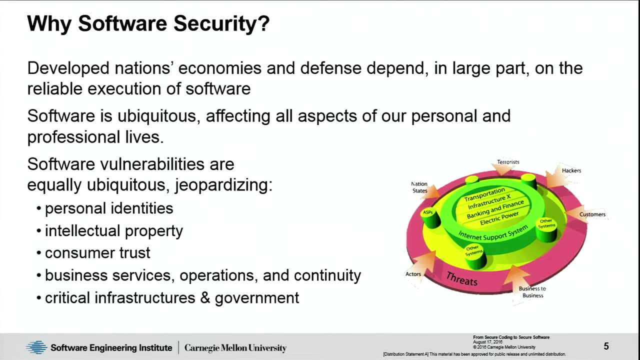 We're here today to talk about the Cyber Security Foundation. We're here today to talk about the Cyber Security Foundation. We're here today to talk about secure software and, in particular, developing secure software through secure coding practices. So I want to start off with: why is that important? 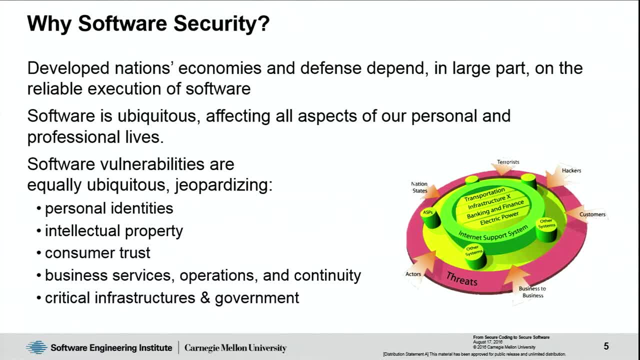 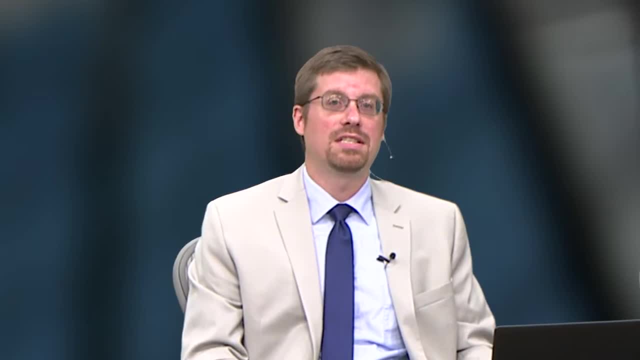 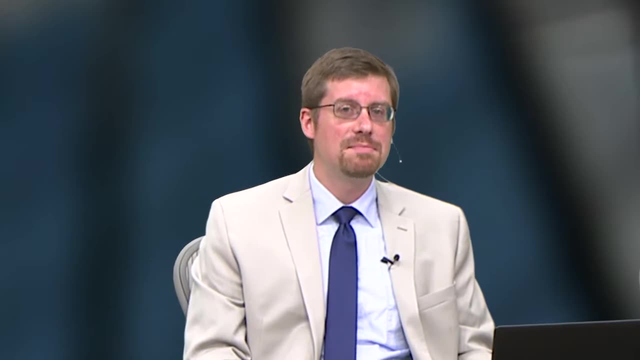 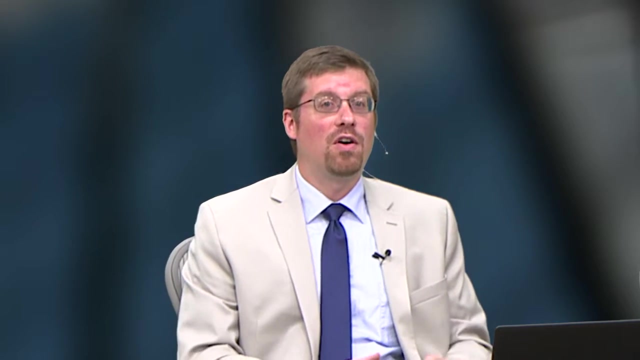 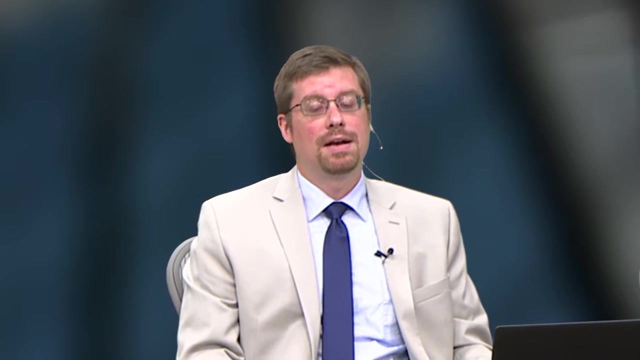 And they're more connected than ever to other systems. Also, a lot of these systems are connected in ways that they were never originally designed to be connected, So it's created other avenues for attack. A great example of all of these conditions was just announced: a couple of researchers at DEF CON that created a proof-of-concept ransomware on a thermostat. 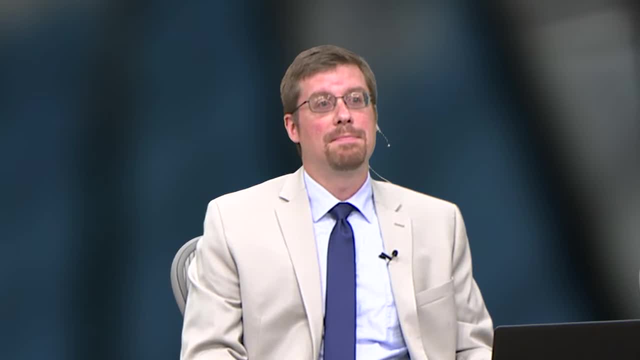 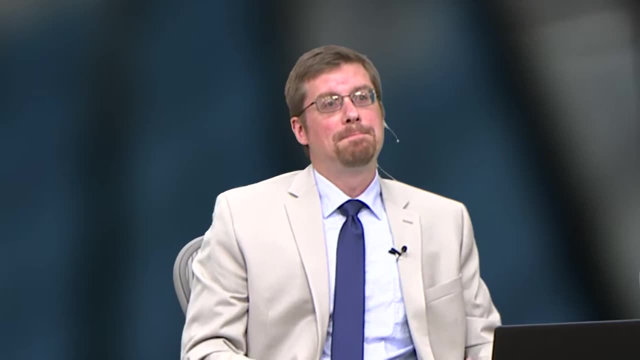 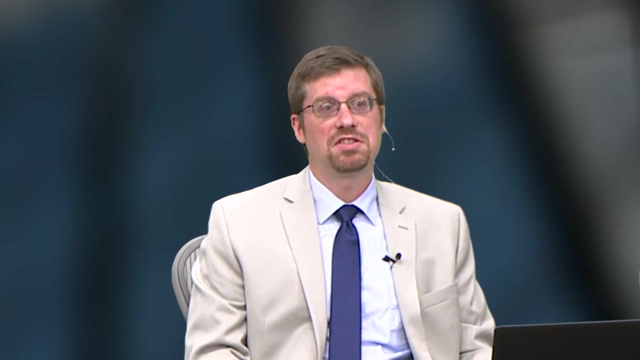 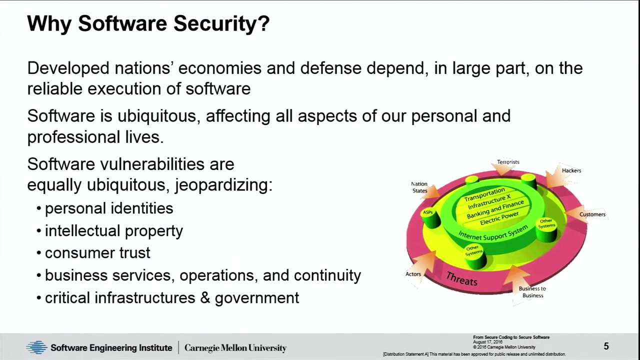 So IoT devices are definitely vectors for attack and we're starting to rely on them more and more, So there's a lot of different important ways that it's affecting our lives, through our personal information, intellectual property of organizations being lost, consumer trust and just general continuity of services. 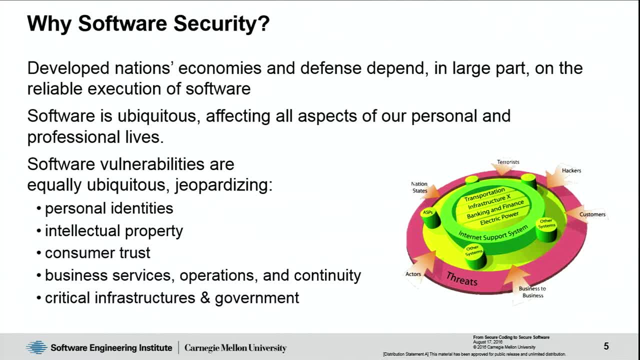 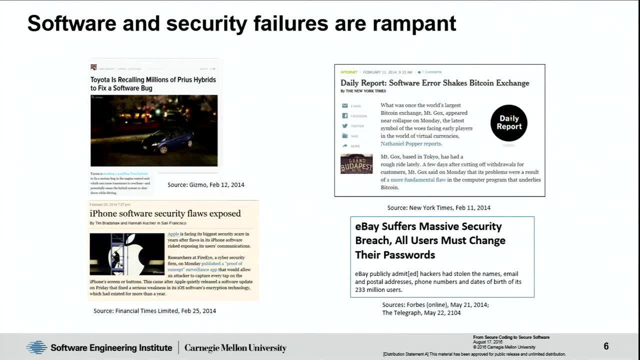 Our economies, today more than ever, And also our nation's defenses, are relying on software. So, as we also know, these vulnerabilities are affecting us and we're hearing about them constantly. It seems like every day, or at least every week, there's a new announcement of somebody or some system being affected by a hacker or an attack. 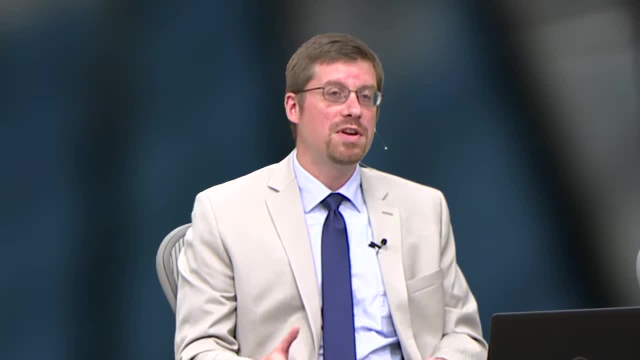 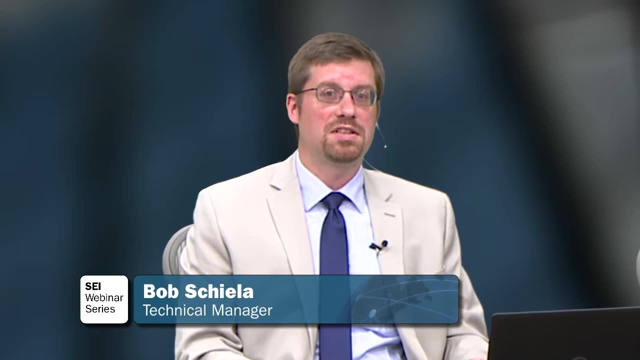 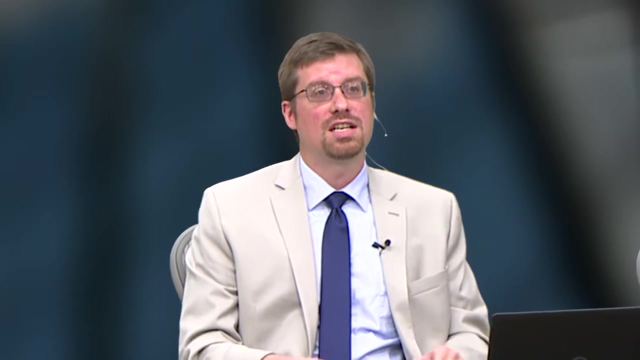 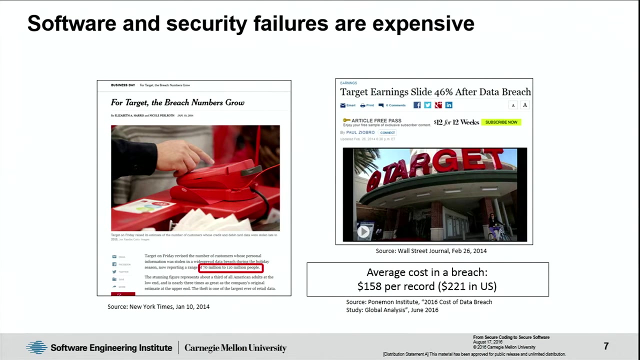 We learn a lot more about the specific coding issues In open-source software, but there's definitely issues with the security of software, whether it's open-source or proprietary. Additionally, the cost of securing the software or, in particular, dealing with the aftermath of a failure. has increased in price because of the amount of data that's being collected and the importance of that data. A recent report, 2016,, a couple months ago, the 2016 cost of data breach report estimates that the cost is $158 per record across the globe. 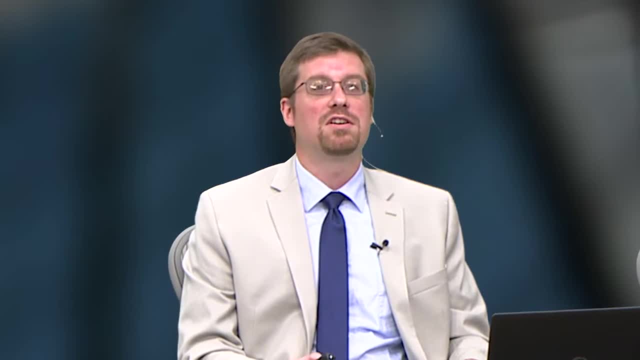 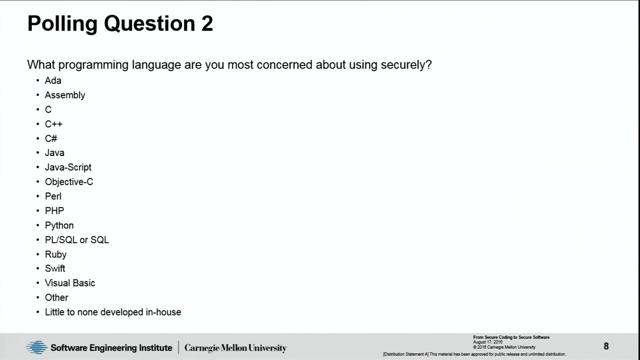 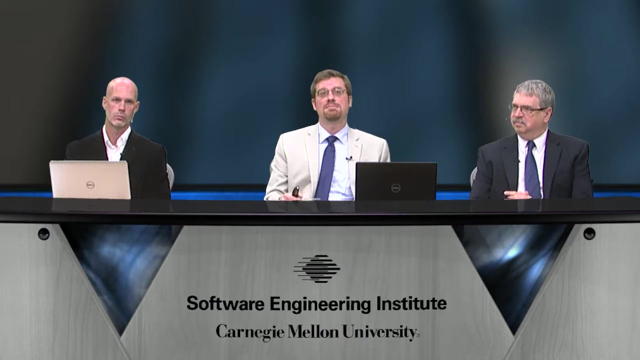 And in particular, the data of the US is about $221 per record that's lost. So we're going to talk a little more in detail about secure coding, which means we're going to be talking about software development and, in particular, developing particular languages. 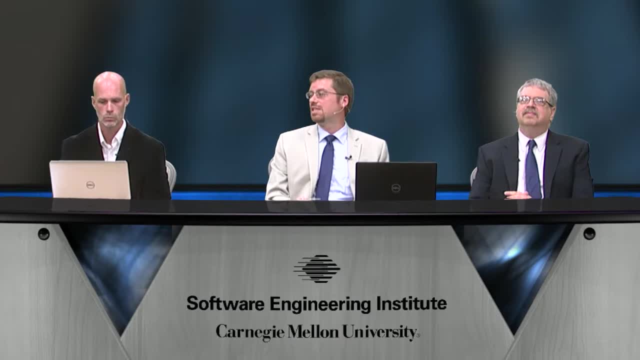 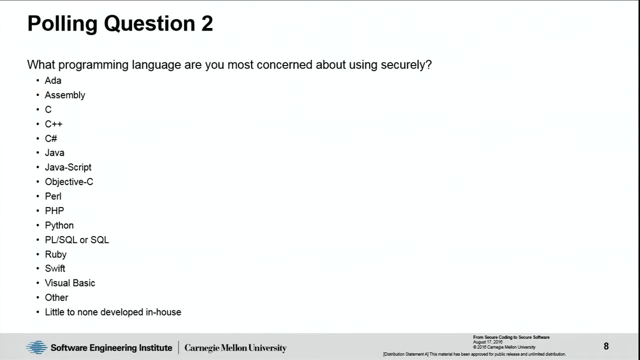 Before we get started in the details, I'm interested in finding out about what languages you're most interested in out there with regard to what you're trying to secure. So the question is posed, so we can see the results in about another minute or so. 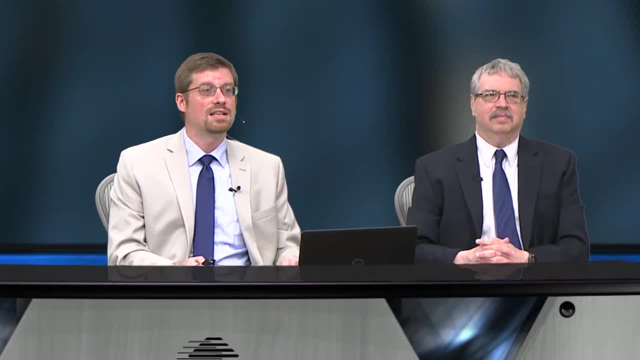 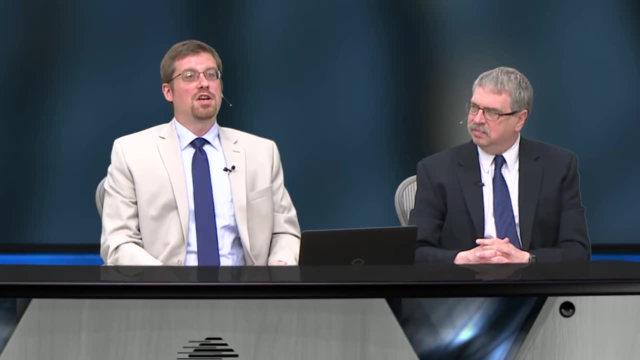 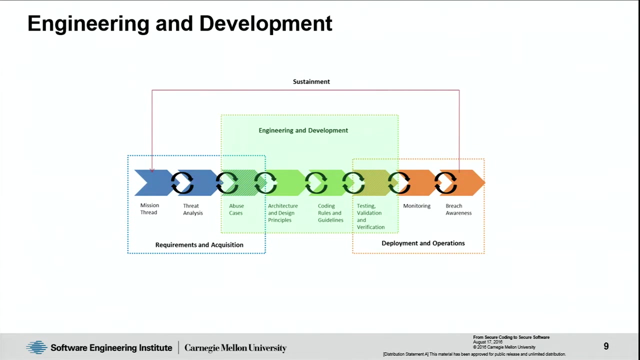 Yeah, so please go ahead and answer and submit your answer to that question. So, as I mentioned, we're going to talk about secure coding in particular, and here's, you know, a standard model of the development life cycle and to us, we kind of focus on the security aspects of this development life cycle. 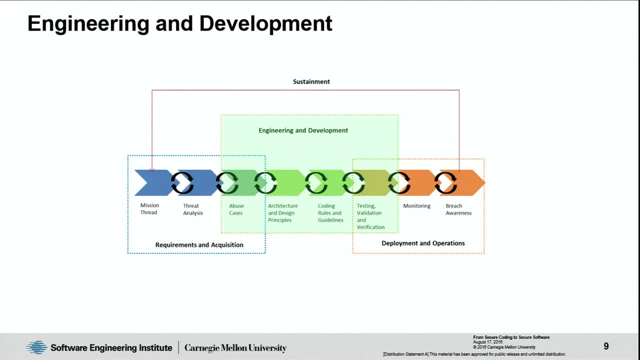 The secure coding group and what we're trying to impact really starts in the green chevron in the center and the one to its immediate right, coding rules and guidelines and testing, validation and verification. That's really what we're trying to focus on improving. 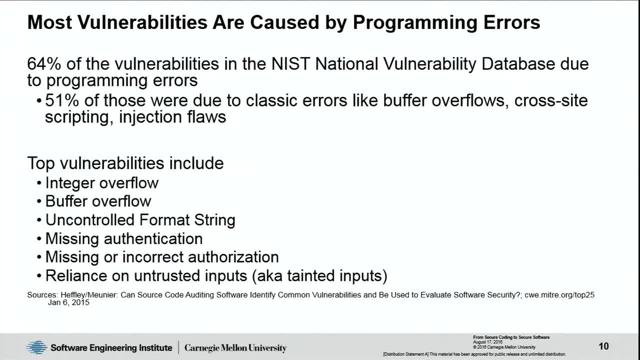 Why are we doing that? We're doing that because the A majority of vulnerabilities, according to NIST reports, have been found to be related to programming errors. In particular, a strong majority, if not A strong majority, if not even more, has been found to be classic errors that are fairly well-known. 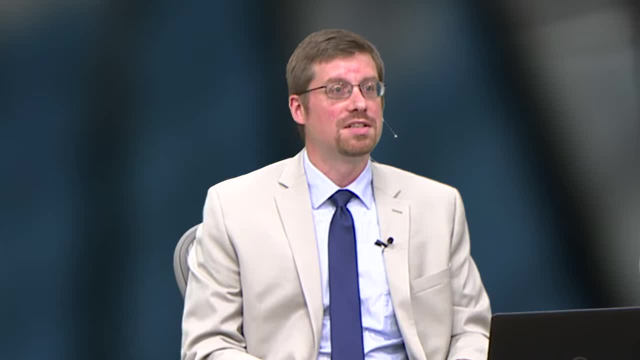 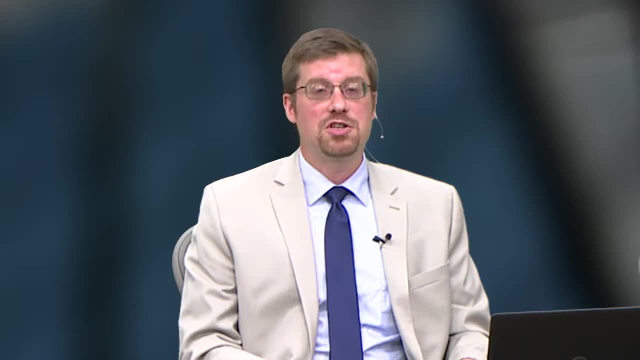 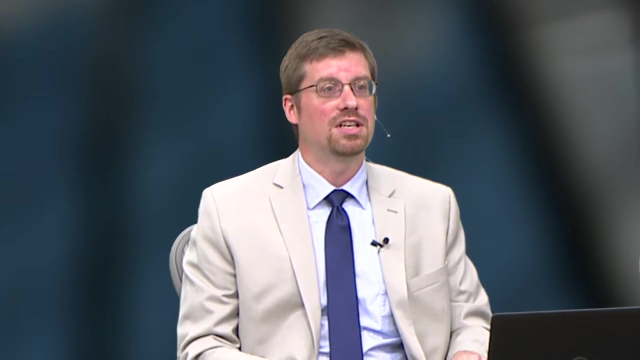 like buffer overflows, cross-state scripting and injection flaws. In particular, top vulnerabilities include integer overflow, buffer overflow, format strings that are not controlled, and then there's also issues with regard to authentication and authorization, And so these are well-known and yet they keep occurring. 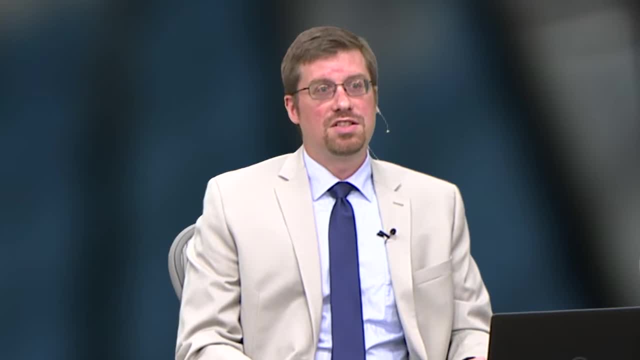 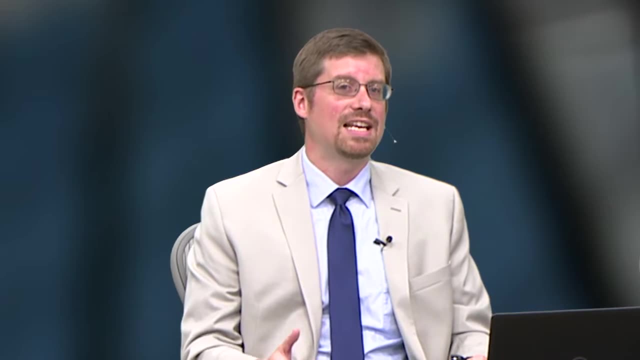 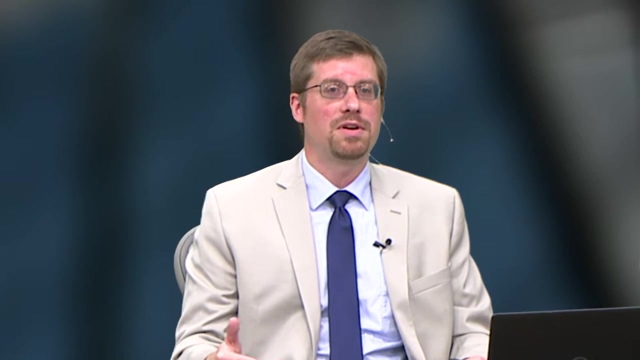 When you're trying to develop software that is secure, it really starts from the beginning, And so we don't lose sight of that, that you need to design it securely. If there are flaws in the design, then It doesn't matter if you use proper coding practices. 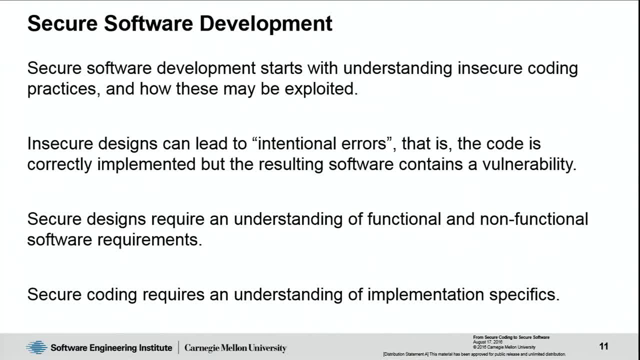 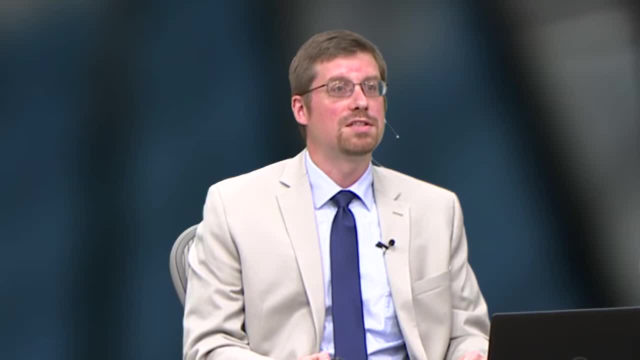 You're likely to have flaws in the software, And so we keep that in sight as well- that the software has to be designed securely. But then even a strong design can be undone by poor secure coding practices, And we'll talk about that in a few minutes. 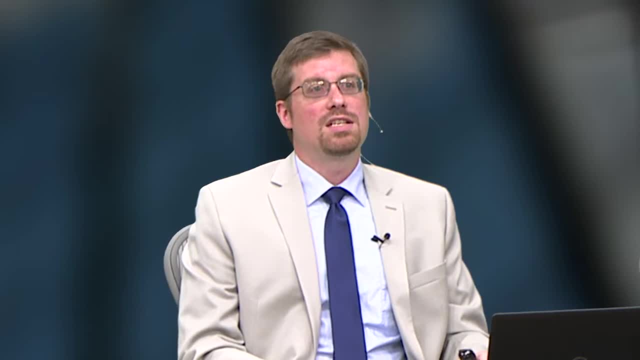 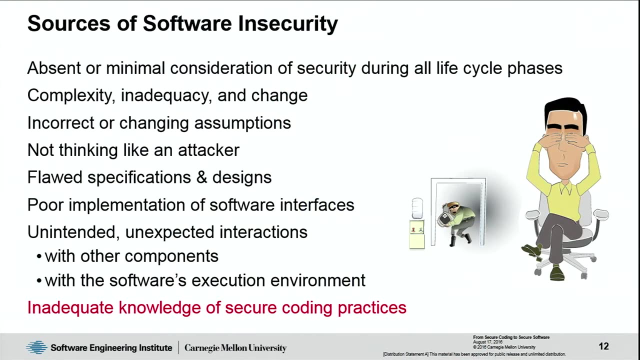 So here's a few of common sources of software. insecurity Again, kind of across the lifecycle, Looking at design all the way through In particular, just to mention a few of them. the complexity of the systems has grown, The inadequacy of a particular system in the context that it's placed. 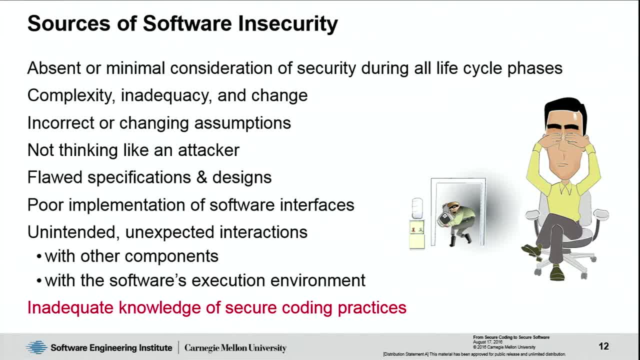 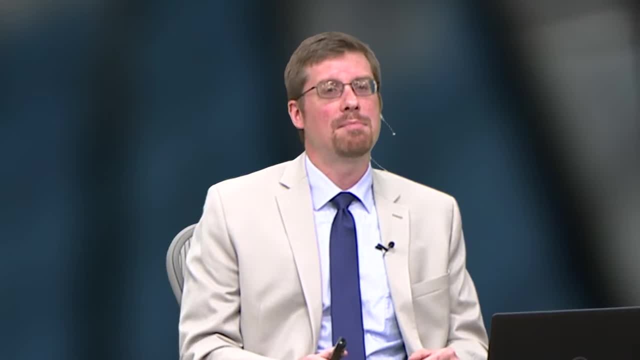 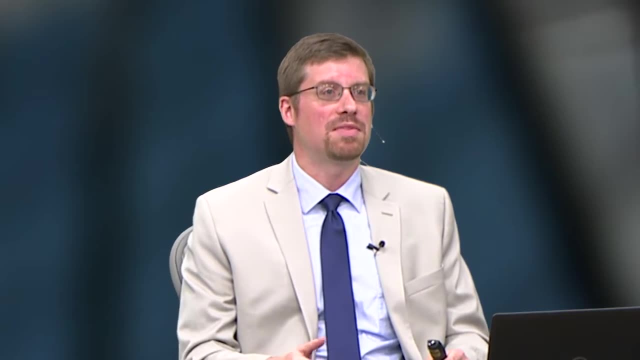 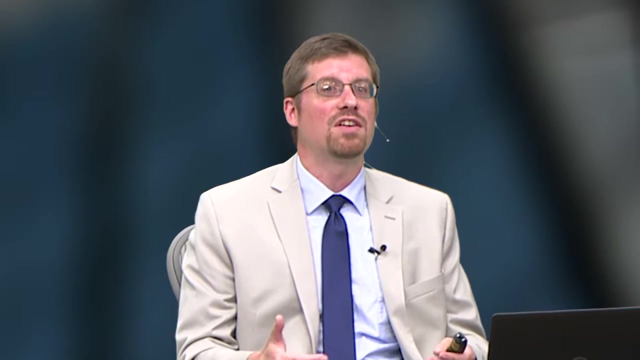 And change and managing that change across the system, across developers and development teams, is difficult to manage, Not during the design, not thinking like an attacker, Just thinking of use cases, of how a user will use it, As opposed to thinking about abuse cases and how attackers might misuse the software to get it to do something the original designers didn't intend is another aspect that can allow you to create software that's not secure. 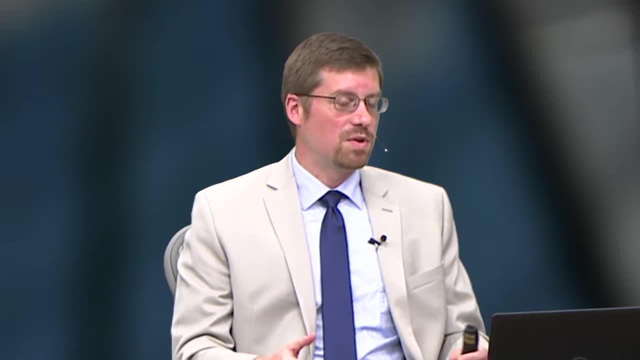 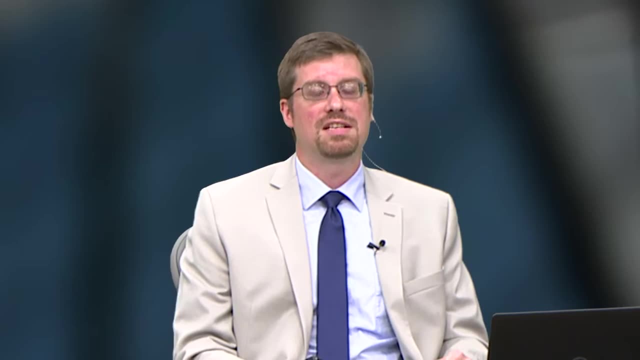 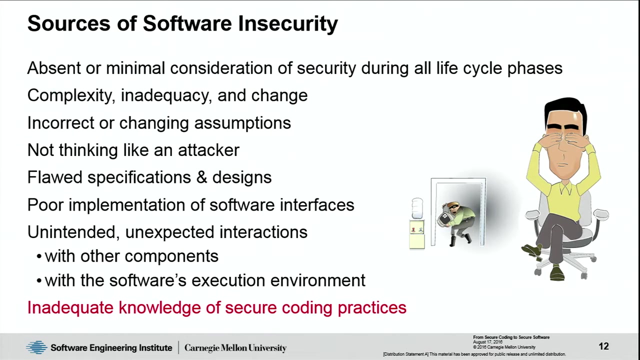 Let's see another one here. Well, a major one that we'll talk a little bit more about with our rules is unintended and unexpected. generically, interactions, But also unexpected, So, for instance, unintended and unexpected behaviors. this is, as I was mentioning, systems that have been designed for a particular context or environment or to be used in a particular way. 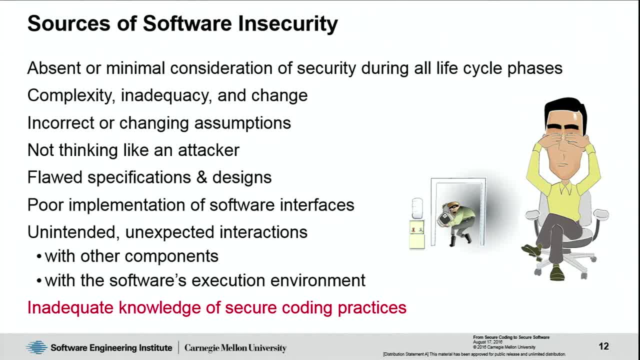 And then later, after it's been developed, is put in a different environment, Or for unintended and unexpected interaction. I'm sorry, behaviors. it is writing the software using language constructs that were never intended by the language itself. So you start violating rules of the language, whether you know it or not, and then the software 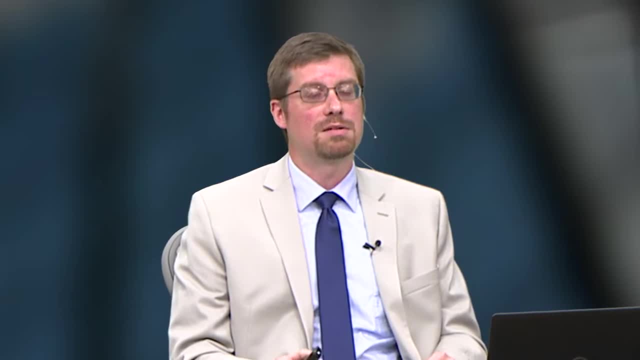 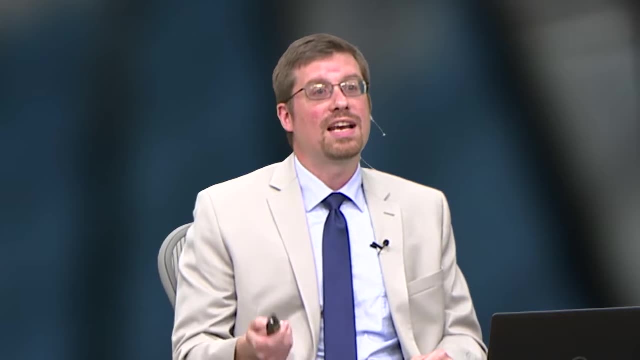 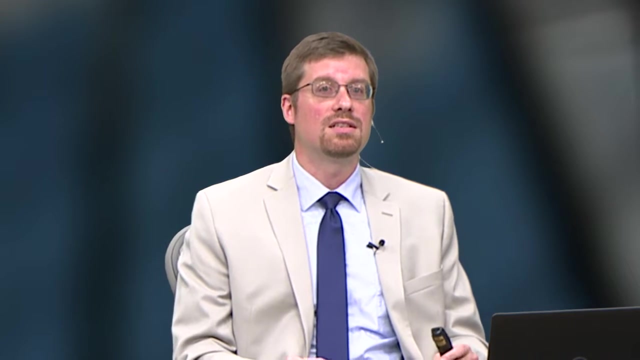 may do things, after it's compiled and installed on a particular platform, that you didn't intend. that leads to security issues. And, finally, one of the things we'll talk about later is inadequate knowledge of secure coding practices, And we'll discuss a little bit today about what some of that knowledge is and what secure 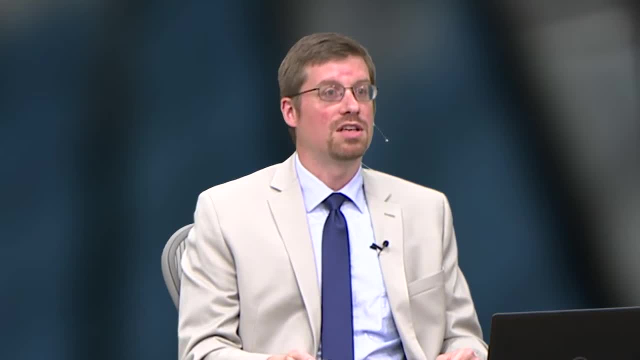 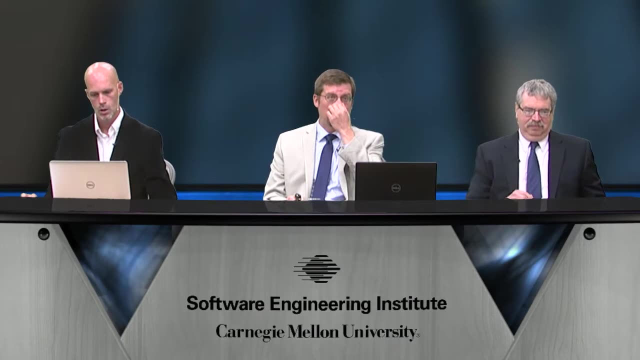 coding practices mean and how you can gain more knowledge on that. So here we have another question that I would like to ask to the group. So, while that one's launching Bob, I can go to some of the results from the last one. 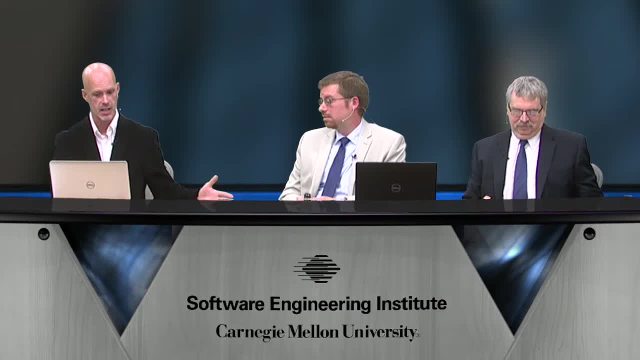 So we looked like we had 24%. with Java, It looks like C hashtag or C pound was C sharp. Is it 20%? Sure, Then C++ 18.. Those were the three main winners. Great Thanks for that. 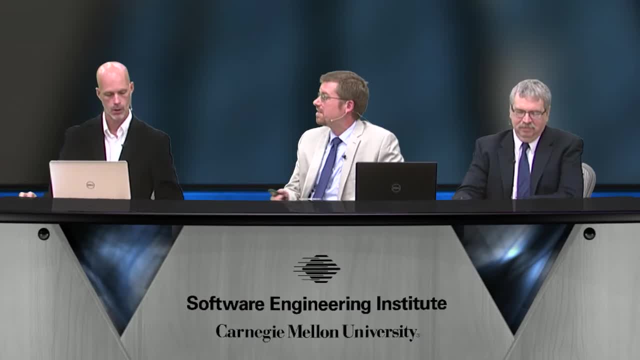 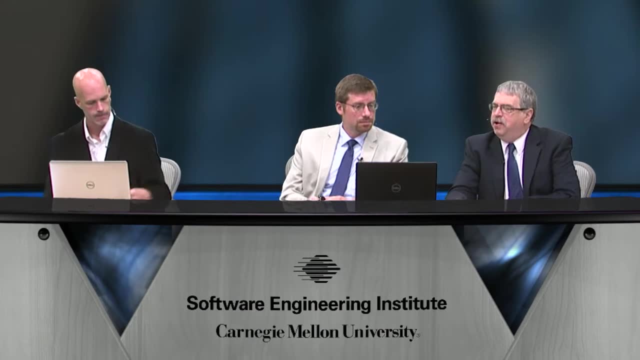 And actually, before we go to the polling question, unless you already pushed it, do we have any questions from the audience up until now? We actually have one interesting comment which we'll actually talk to about. It was a question about that SQL injection was noticed quite a while ago and yet we're. 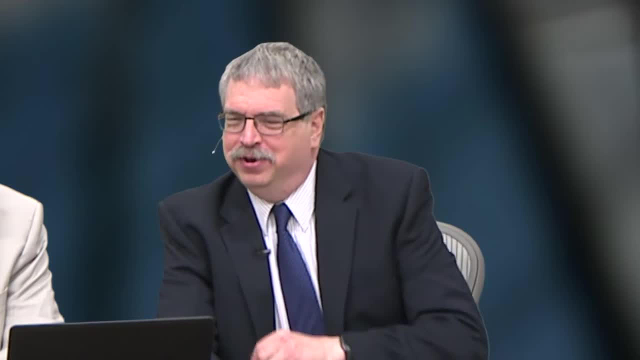 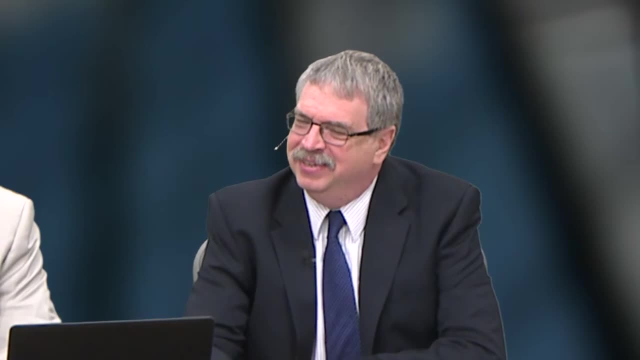 still hearing about it And I'll paraphrase: why is that? And we'll actually talk a little bit about that in a moment: Bobby Tables- I love Bobby Tables. It reminds me of me because my name's Bobby, So Yes, 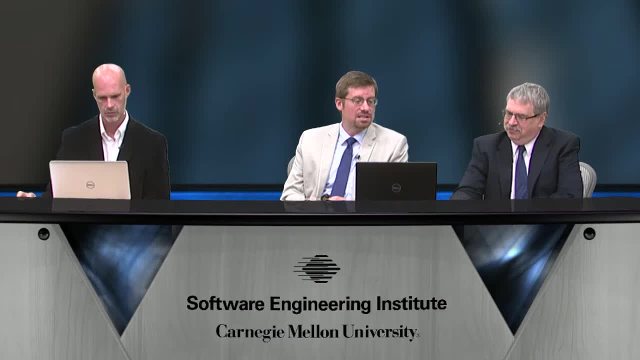 Yeah, that goes to the design issues and some things that have nothing to do with coding- Or in one language that then is interpreted by a different language. And just to wrap up our results: 47% with yes, they use a coding center for security. 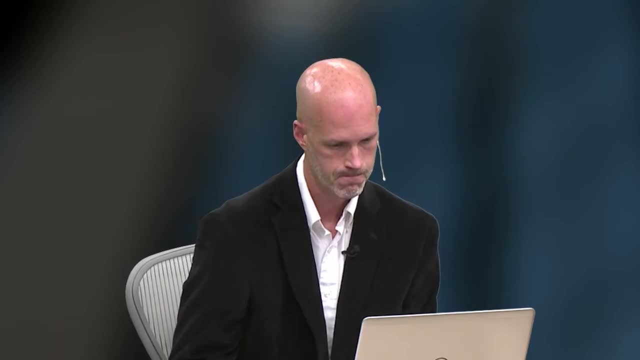 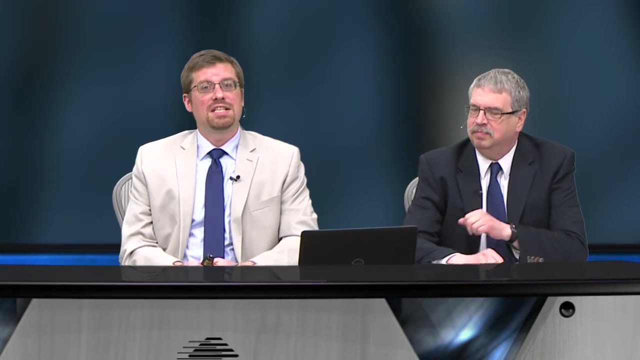 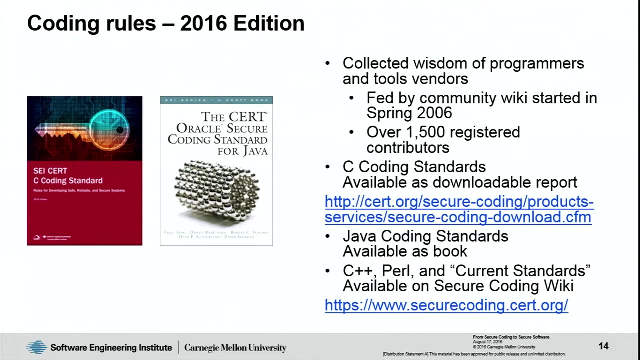 23%, no, 29% maybe. Okay, Great, Thank you. And so what are the standards? You know I've mentioned them several times here. Yeah, So at CERT, in the Software Engineering Institute, we started codifying best practices for coding. 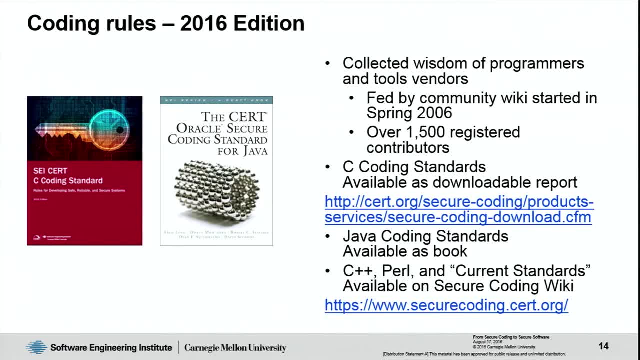 securely in specific languages about a decade ago, And it all started with the recognition that a lot of these issues are common. So we started looking at what's common and how can we prevent these common errors, In particular, which errors are being caused by misuse of the language. 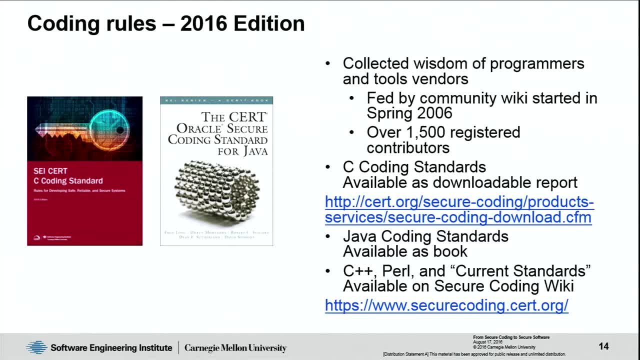 Yeah, And so that started with a general best practices book, And then, as our knowledge matured, we started writing specific coding standards- for C and for Java eventually, And so we're going to talk a little bit more about what's in those standards, but they're. 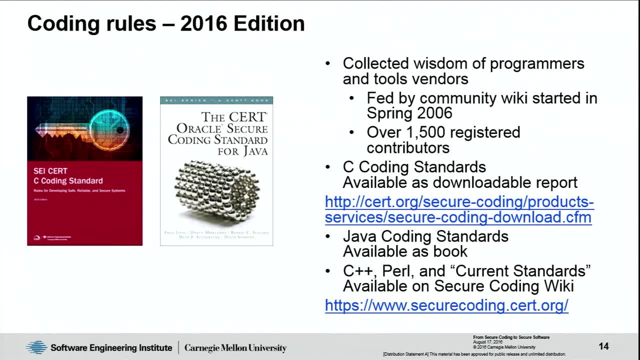 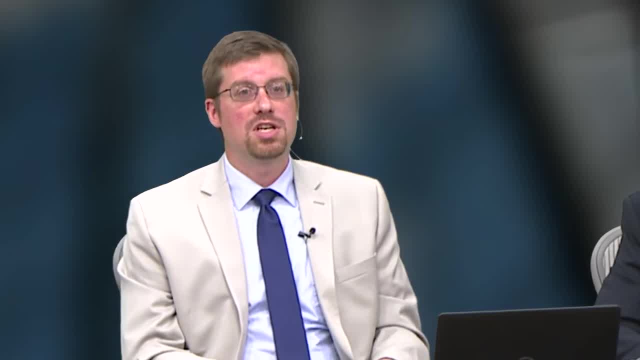 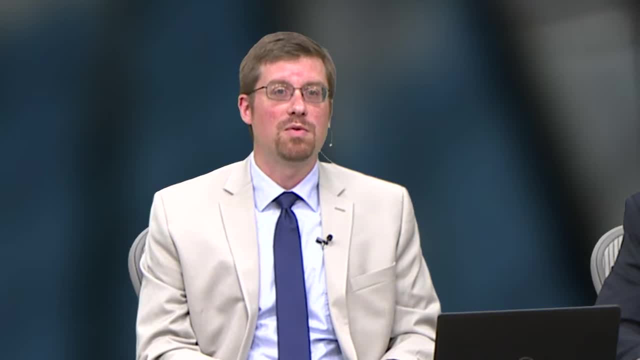 generally a compilation of how to use the languages and the constructs in the language securely avoiding common flaws. And so recently we just released- a couple months ago, Yeah, We released- a new version of the C coding standards as a downloadable report. The link is there so you can download that freely. 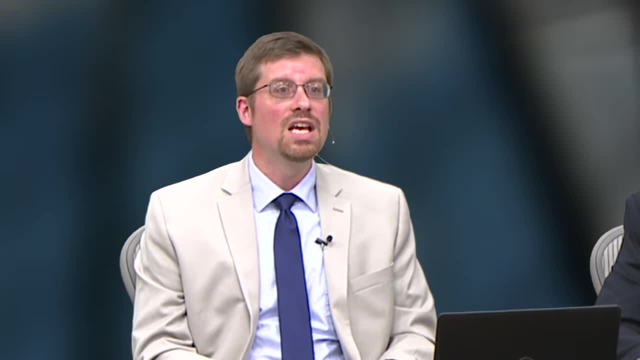 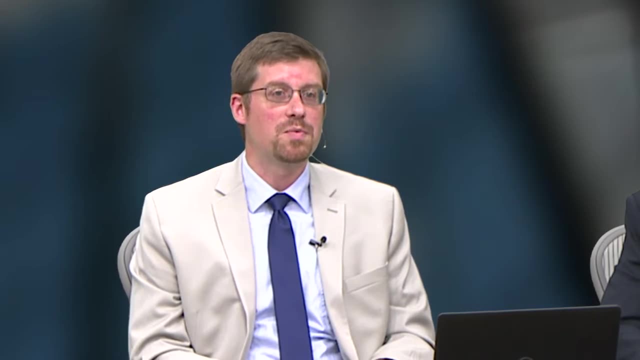 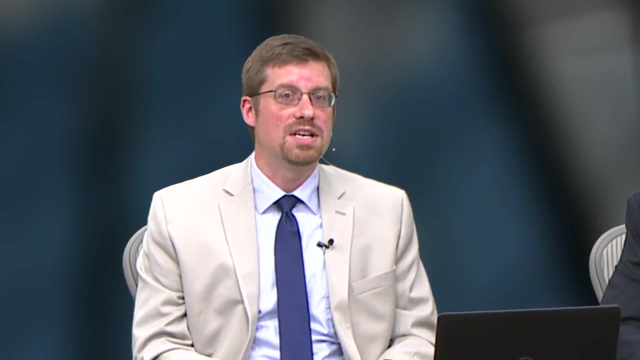 The Java coding standard is available as a book, And we also have C++ and Perl standards that are in development but available on our secure coding wiki, as well as what I call, or we call, the current standards. They're kind of the in-flight, you know, in-development, beta version of the standards. 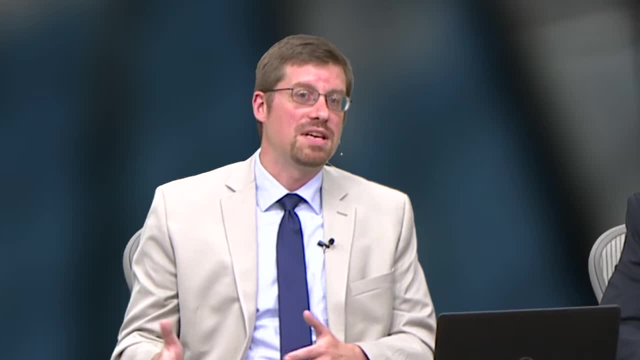 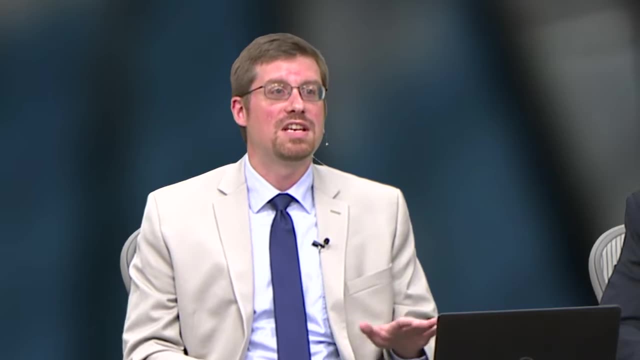 They're available on the wiki, but they have not been. you know the changes since the last iteration of the publication, basically, And so if you need a snapshot of it, you can download the PDF, But if you want the latest and greatest rules- and I'll even mention a couple things that 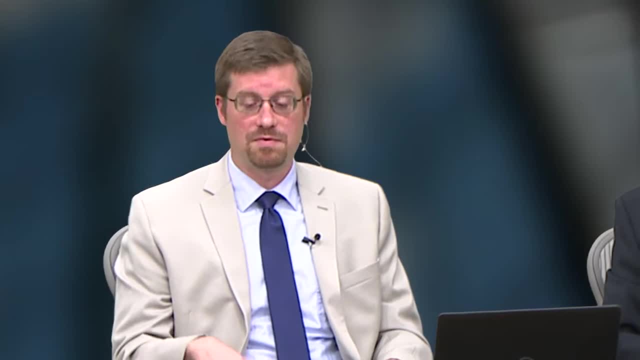 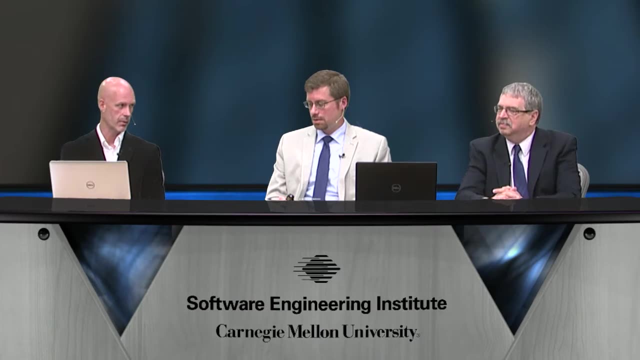 have changed in the last couple months. you can get them from the wiki. Now, are there any other questions? We do Just one from Ed asking any work on secure Python programming. Sure, So We have considered working on a couple developing languages, on a couple other language. sorry. 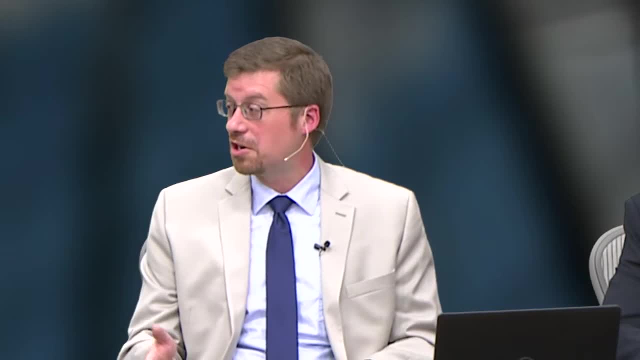 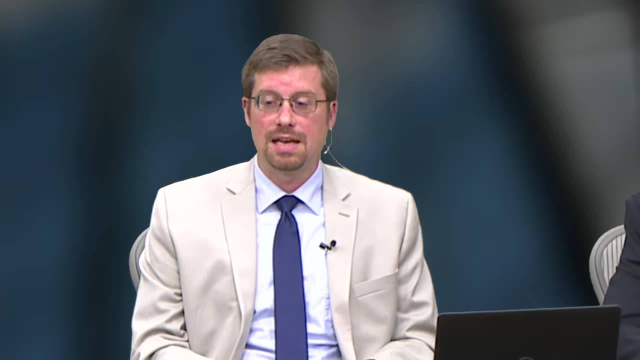 standards on a couple other languages, Python being one another common one, as you mentioned. The second option was C Sharp. We don't have one for that, And several customers recently have been asking us about Ada, which is kind of a surprise. 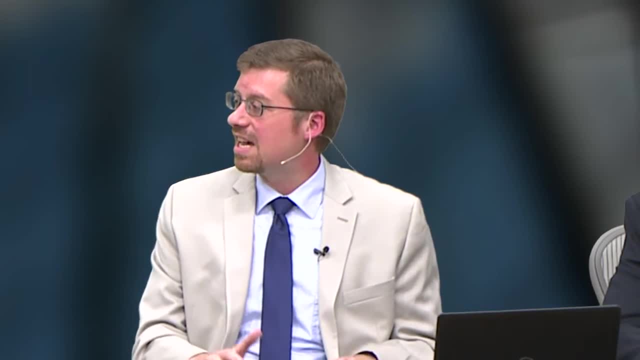 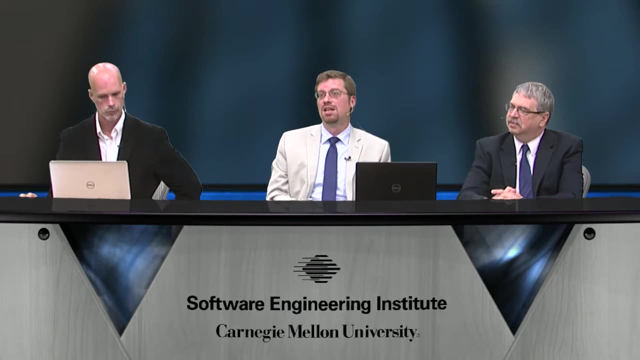 but it's come up. We're still kind of deciding what we're going to develop. We might start developing, as I said, kind of a beta version on the wiki soon, but that kind of depends and is often driven by customer demand, customer often meaning some sort of. 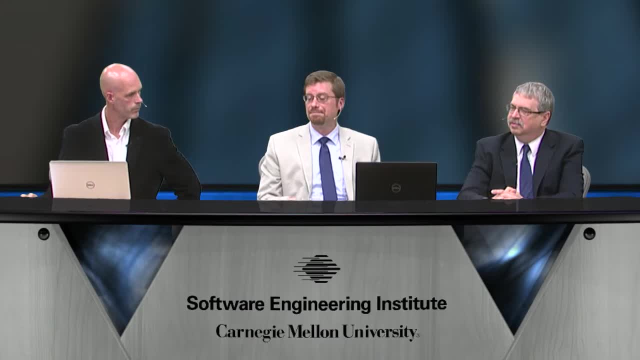 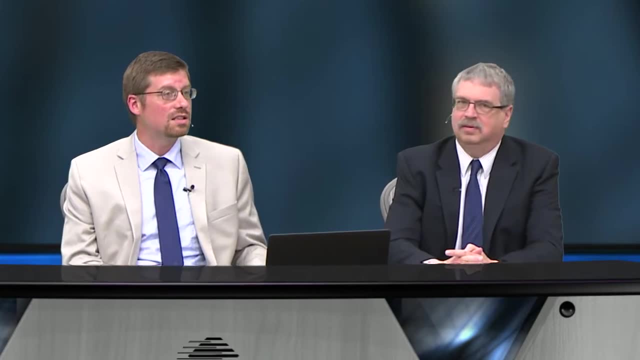 funding source. so it just depends on that demand. Okay, Okay, And actually, with that, I was wondering, Mark, if you could tell the audience a little more about the rules and how we develop them. Sure, I'd be happy to. 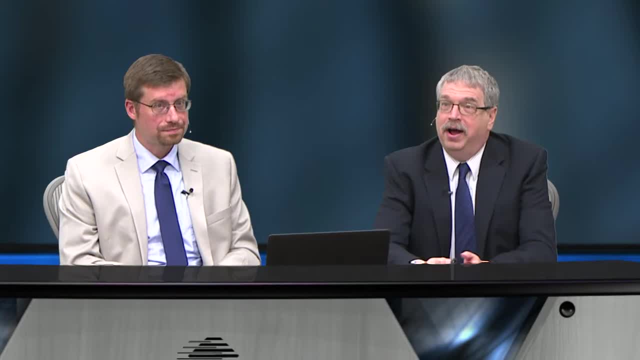 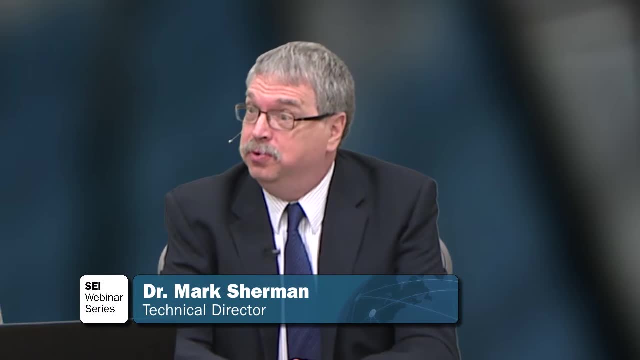 Sure. Well, first of all, I'd like to talk about the history and motivation as to why things don't seem to go away, and some of the discussion that has been going on in the chat address some of the issues, which is the reason why other languages that you might use to prevent. 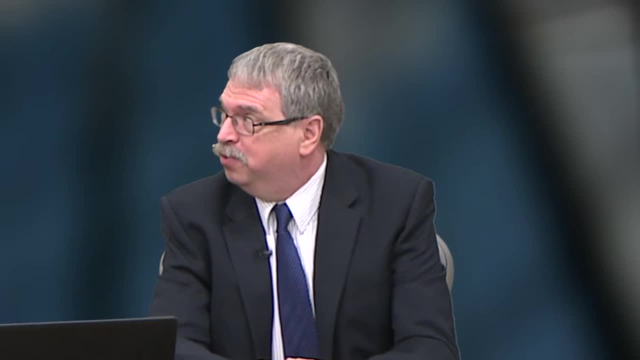 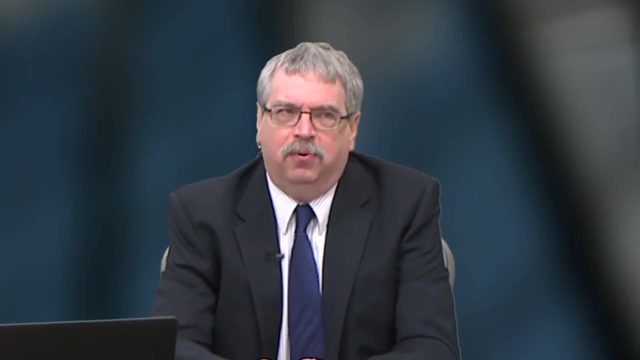 them aren't widely adopted is because they make tradeoffs in time and space that programmers may want to use. but that also makes the challenge in adopting the rules. So let's consider one particular example. SQL injection was the one mentioned in the chat room. 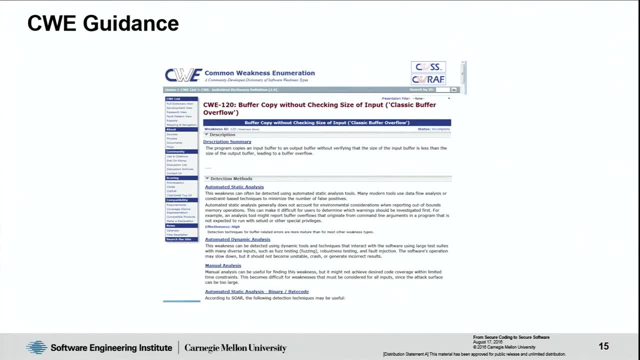 It's saying: we know about this, How come we're still going on? And SQL injection actually is an example of a more broad class of problems, which I call the eval problems, basically taking in a string of some sort and then performing an evaluation. 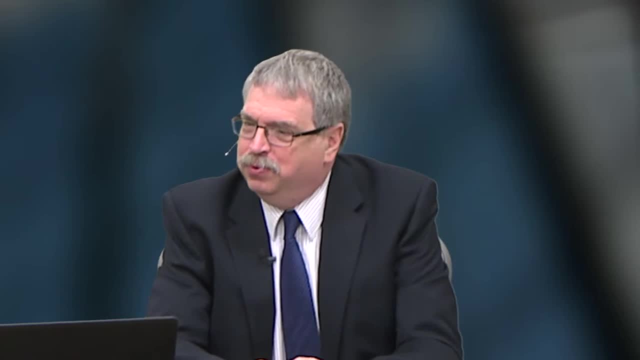 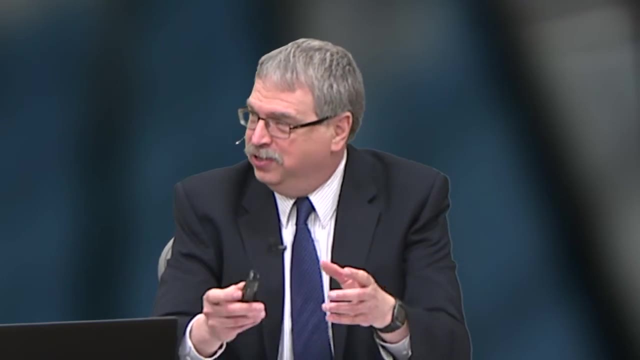 on it: Eval. if you're a Lisp guy, There's exec. if you're a SQL guy, There's a variety of different verbs for that. but the idea is you take in a piece of code, you trust it. you basically say, go, execute this code and it's bad code, and you get. 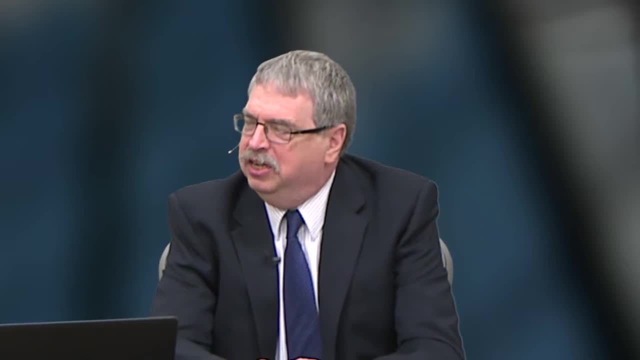 something like SQL injection, And part of the challenge in dealing with that is being able to give good advice to the developer on what they should do about it And rather than take SQL injection or cross-site scripting, which are a little more complicated examples. I'm just going to walk you through a little bit of a more simple example: buffer. 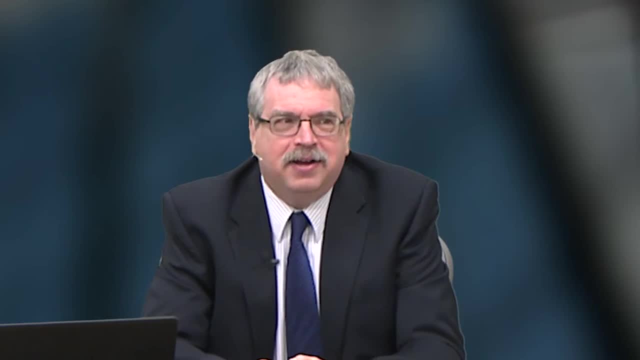 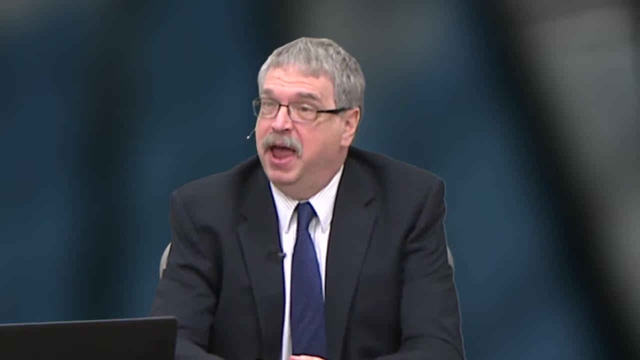 overflow. Buffer overflow, in the case you've been living under a rock, is an example where you're either reading from a space that you shouldn't be or writing the space that you shouldn't be- a mismatch in two boxes. And so there's a lot of talk, a lot of guidance about what to do here. 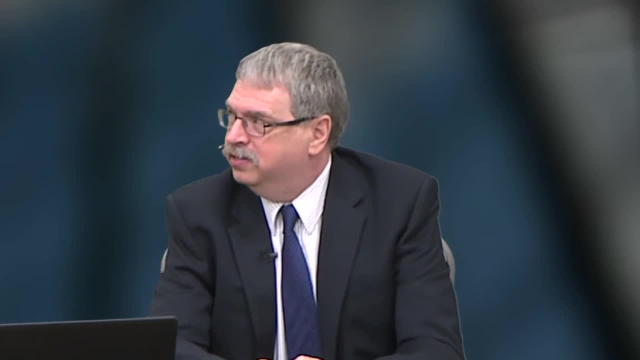 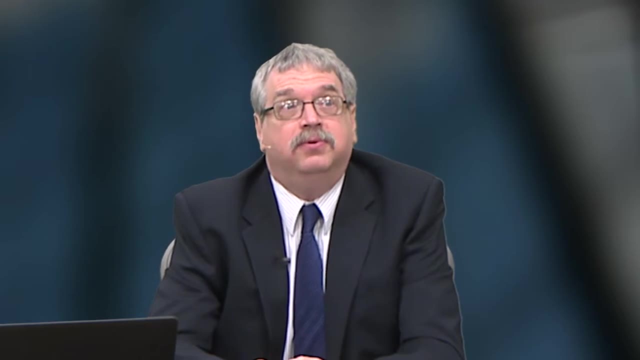 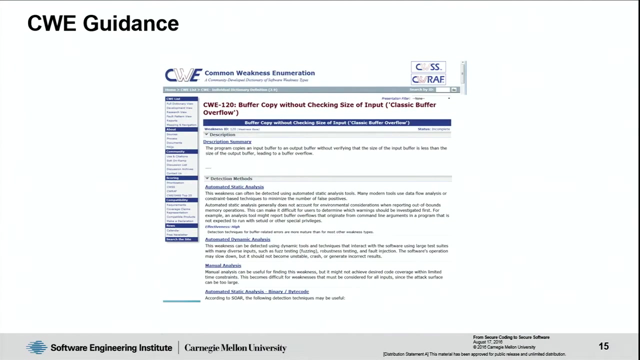 And just to show you the two most common sources of guidance that people look to: CWE that MITRE sponsors or MITRE hosts- I should say I think DHS actually sponsors it. Common Weakness Enumeration: This is a particular page that what I picked is their guidance on for classic buffer overflow. 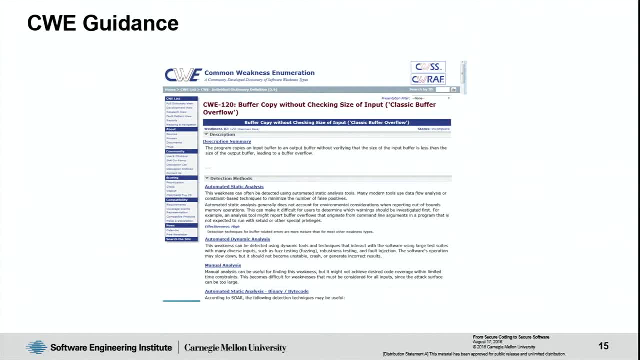 And I don't know if you can read it on the fly, But you'll certainly be able to study it later. It says: what should you do about buffer overflow? And it says: well, read your code very carefully. It says: have someone else read your code very carefully. 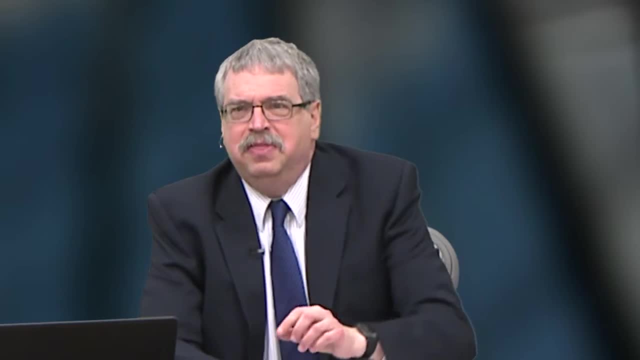 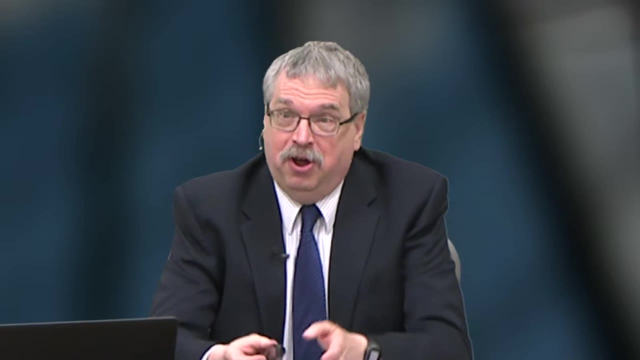 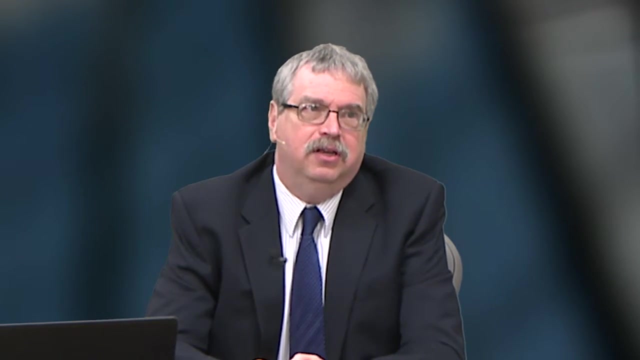 It says: run a tool to see whether you can find the problem or not. That's not very specific advice that you can give to the programmer on what to do. Programmer, when they write code, don't intentionally write bad code. Probably the next most widely used source of guidance is OWASP. 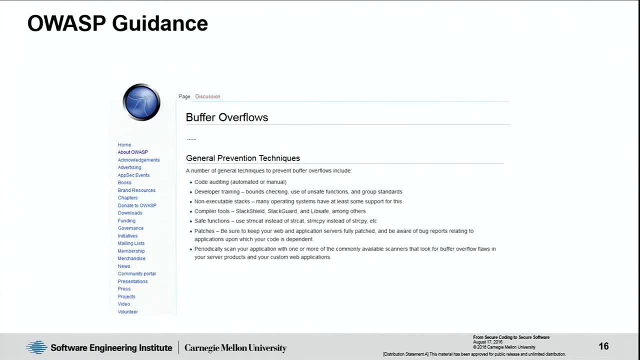 The Open Web Guidelines. And again, here's the generic buffer overflow guidance that they give. And they say: so what should you do to prevent it? Well, it says: code carefully. It says: read your code, have developers look it over. 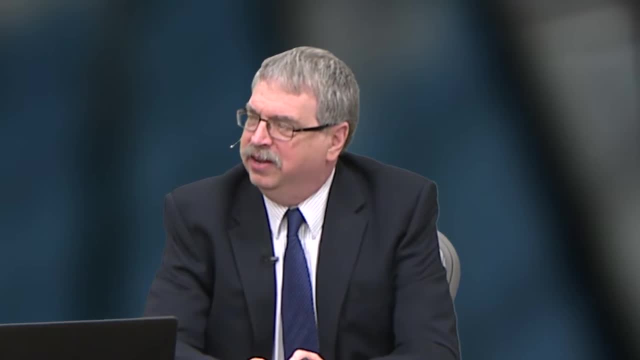 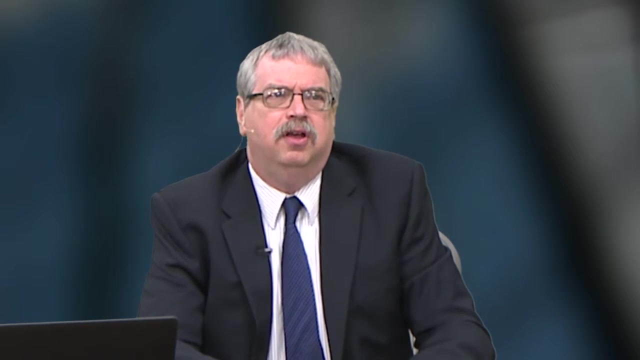 Run some tools on it. Some you might even see things like check that your indexes are OK. That's a little better, but still is not very prescriptive of what you should do or proscriptive of what you avoid. And again, let's consider some reasons why. like again, the usual buffer overflow. 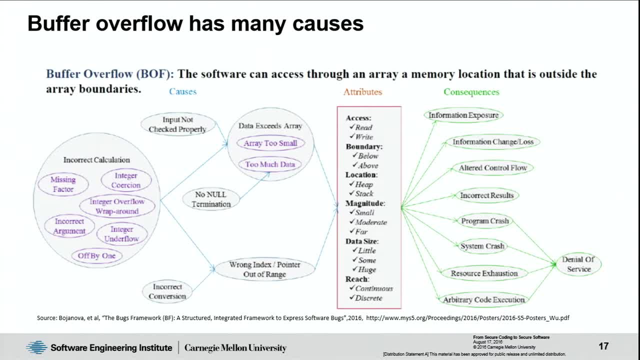 It turns out buffer overflow, and this is a simple one, As I said. for the other ones, they're much more complicated. Buffer overflow actually has many, many different things that cause that problem to occur. So, for example, it could be that the input that came in through the system is tainted. 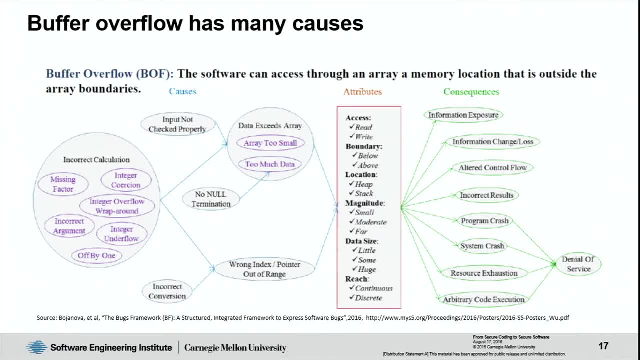 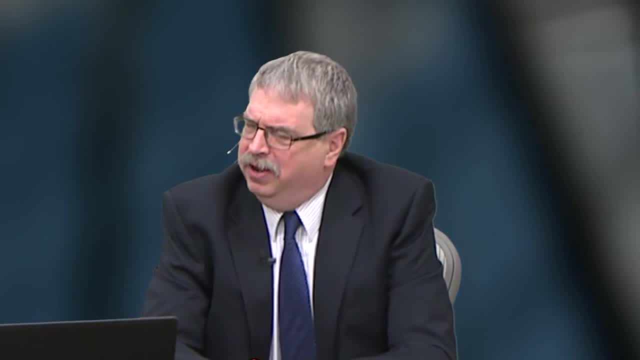 It could be that you didn't have the right scaling factor. It could be that you had some sort of integer overflow or integer underflow. Now that one may not seem apparent, but let me give you an example of how that might work in practice. 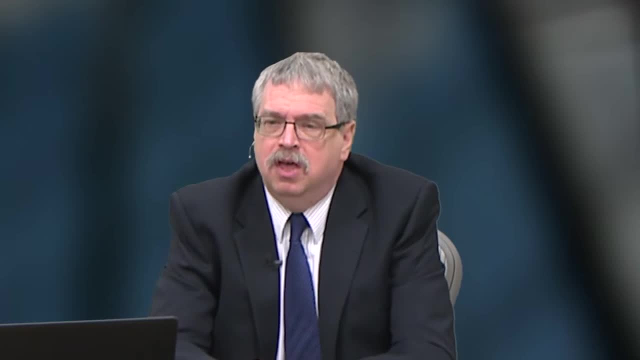 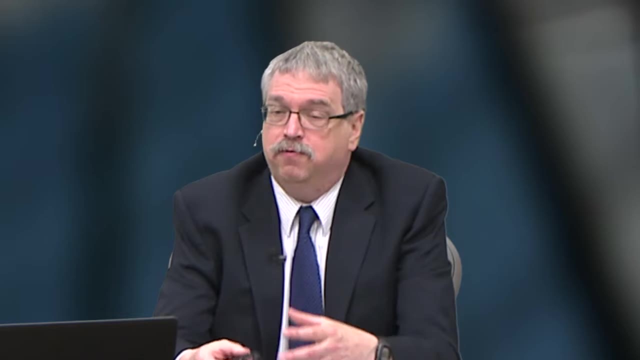 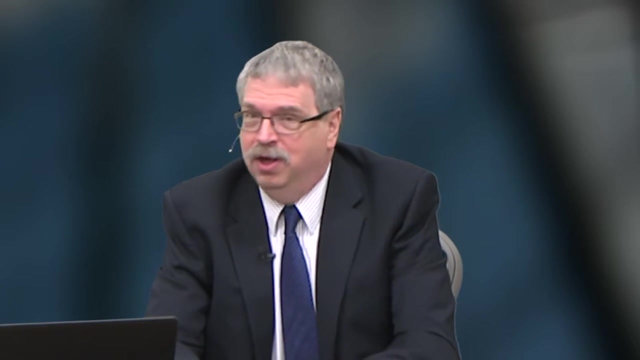 And again it goes back to the realization that people pointed out that when you're writing code, especially if you're running something like C, you're very conscious about trying to be very fast, trying to be very small. So, even if you give the guidance, check your bounds and that will prevent buffer overflow. 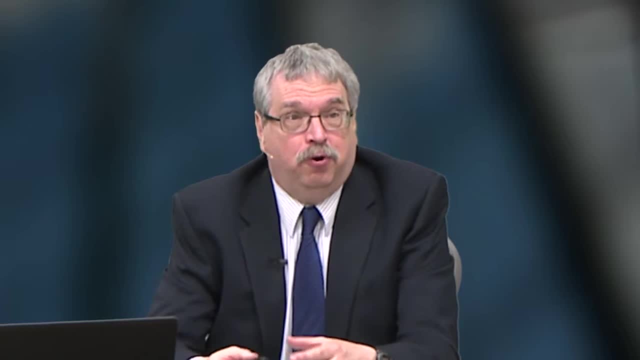 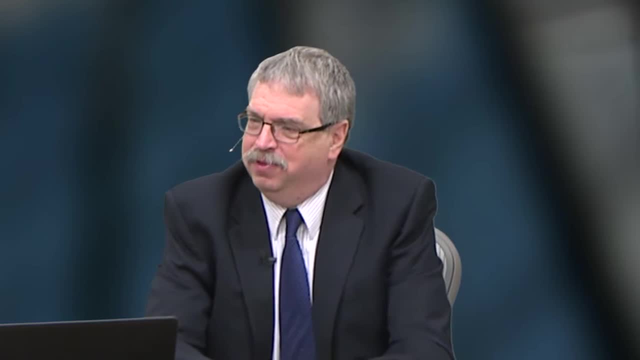 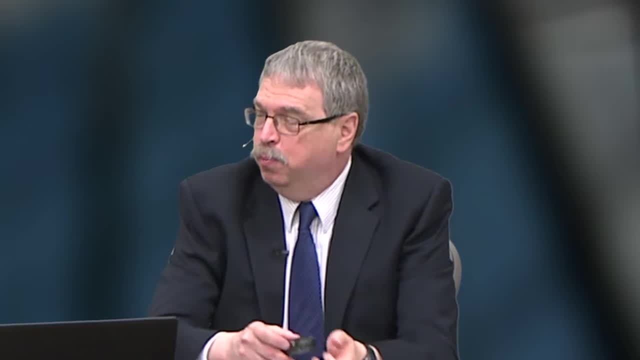 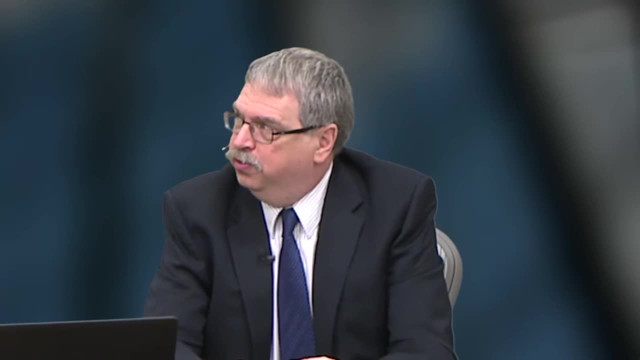 You just basically take an address, a pointer, and you add a number to it, And then that gives you a pointer into the array And then you use that to index. And so the efficient way in C in order to see whether you've exceeded the bounds is 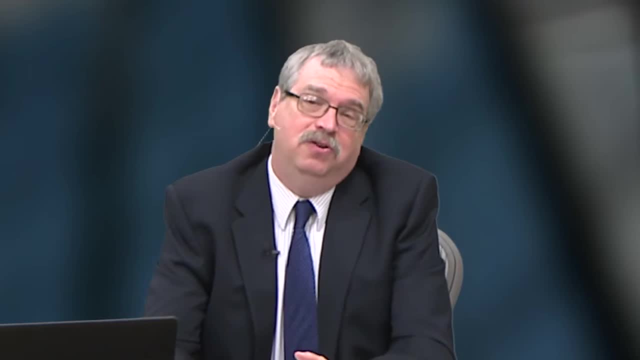 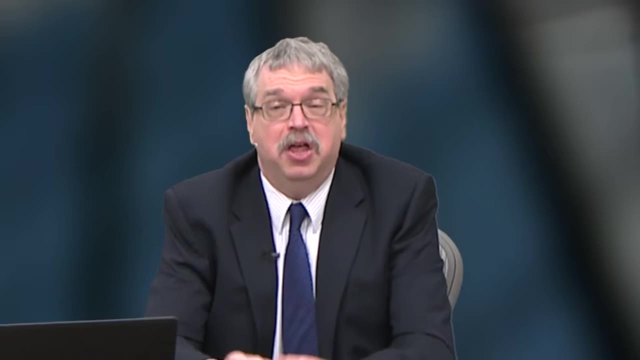 you start with the start of the array as a pointer, You add in what you think is the test index, some value that you read in from the outside, And you compare it to the pointer that is at the very end. You think you've now checked the bounds. 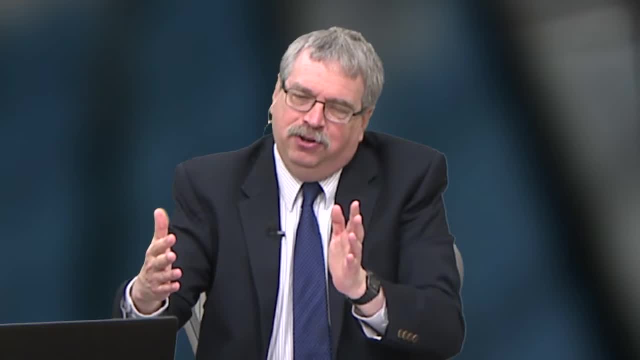 You think you've now checked the bounds, The thought being, let's say, if you have an array of 10, and you get an 11, it's a little bit beyond the bounds. You see that it's beyond the bounds. You say, oops, there's an error. The problem is, if you're having something malicious, is that it's not 10 going to 11 that comes in. It's 10 going to 100 million that comes in. When you add a gigantic number to that initial address, you get an integer overflow. 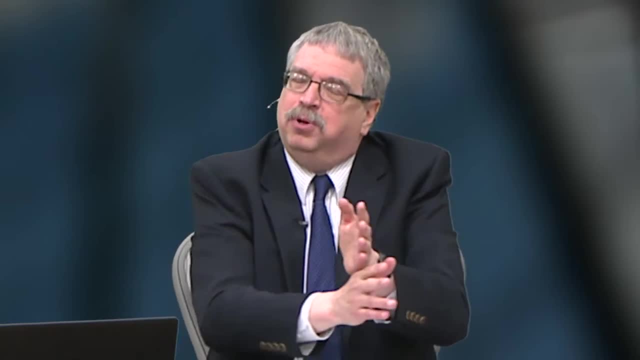 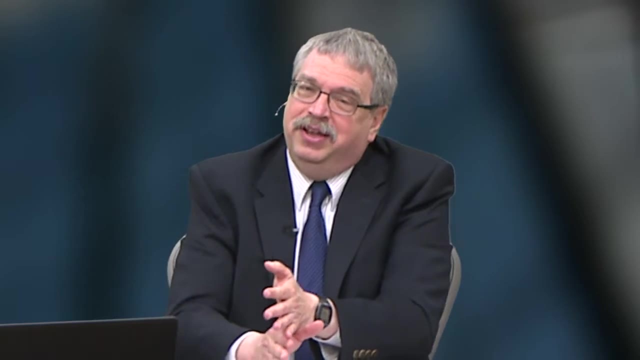 That's a fancy way of saying that a number wraps around and actually be below the original base. So if you want to see: have I gone beyond the end of the buffer? the answer is no. It'll look like you're in front of the buffer and you'll say everything is fine. and then 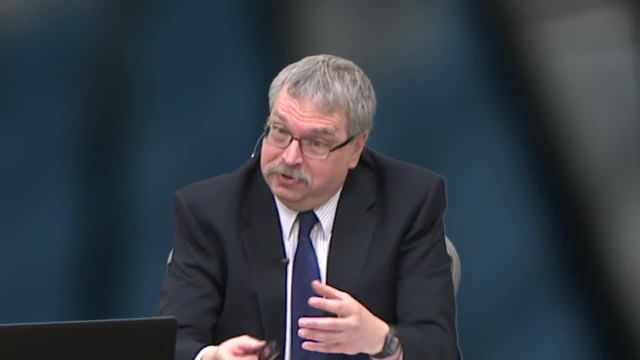 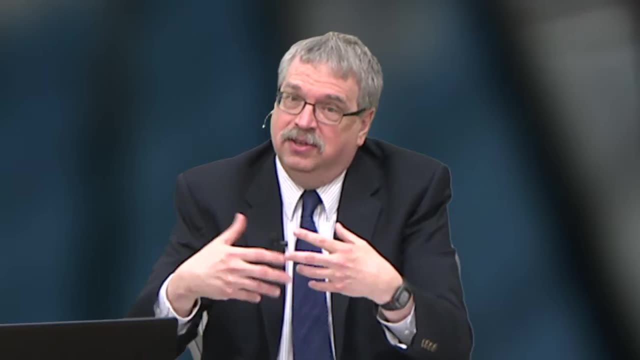 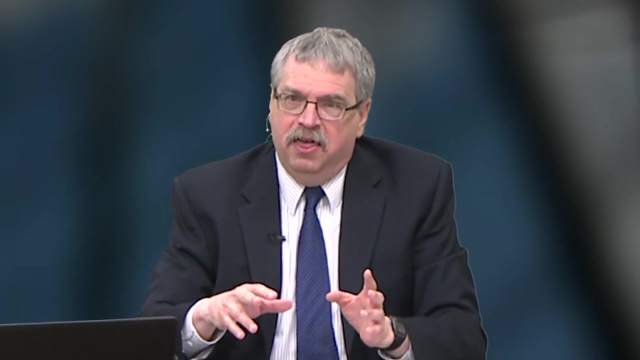 you start getting into problems. Now there is a way to do this kind of buffer overflow checking, bounds checking, But it's a lot more subtle than what you might expect to do as a standard C programmer, Coming up with those kind of actionable, precise rules that actually help you build programs. 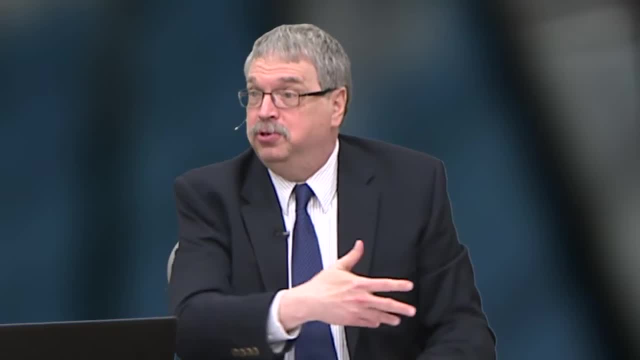 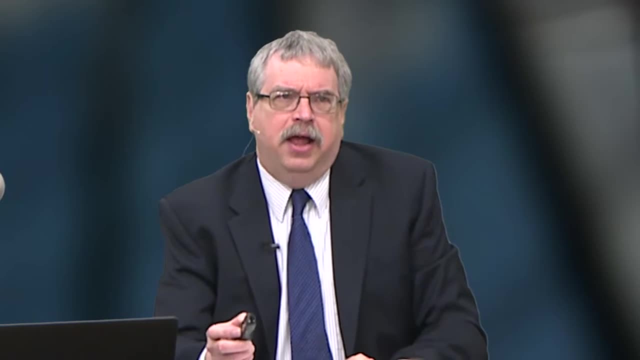 that are resilient. It's really what rules ought to be about, as opposed to what we see here in a lot of the overall guidance, which is useful at one level but not really actionable. And so what a couple of groups have done- we are one of them, frankly. MISRA is another. 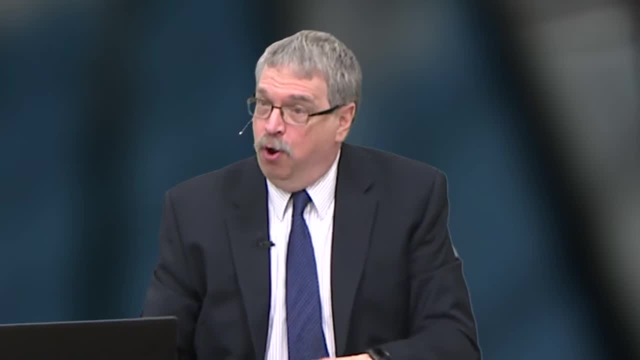 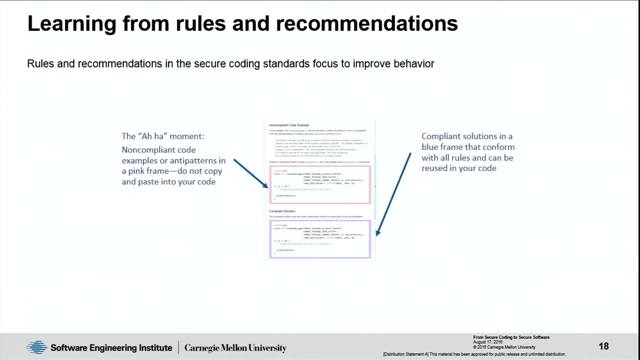 one is: develop standards that don't say: don't do buffer overflow. They say here's how you should carry out the pointer arithmetic in these kinds of situations so you don't generate these overflows and you actually check to see whether you're in. 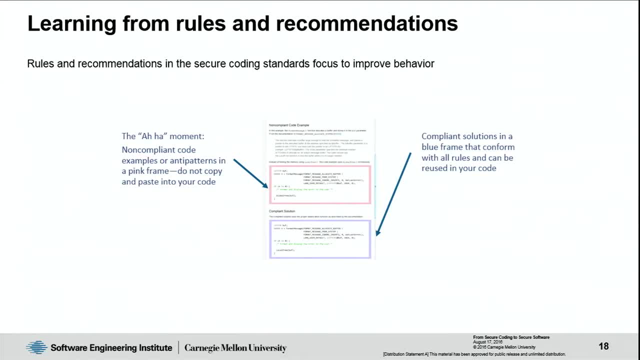 bounds or not. That is a way, then, that you can make sure that you are meeting the goal of not creating a buffer overflow from at least one source: the integer overflow. Now, in the case of both UF and MISRA, the way we do it is: we have some rules. 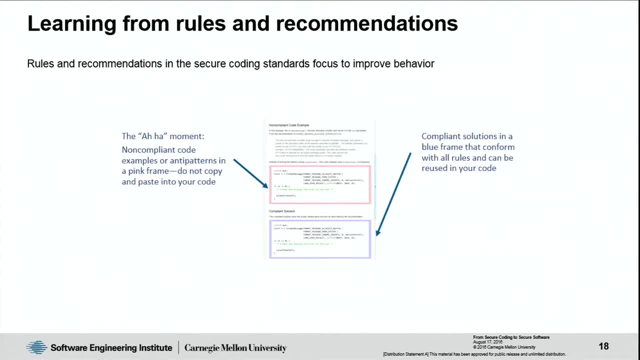 That's what the very top part of this is, But perhaps as important is, in the next section of the standard we give examples of what code that looks good might seem but really isn't, as the example I gave where you're trying to do the pointer calculation. 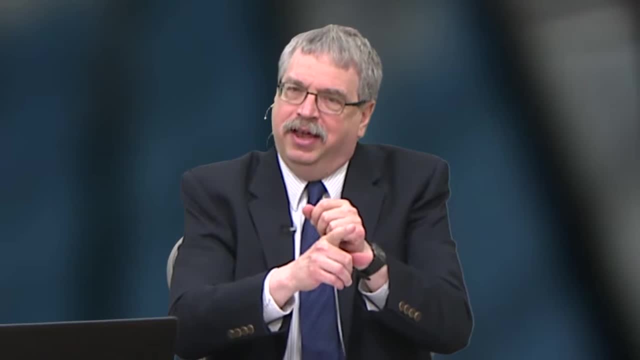 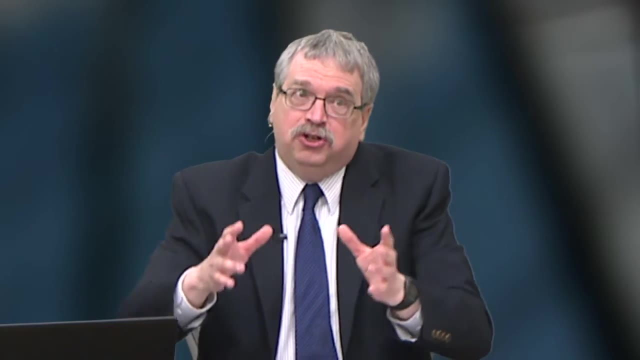 And you wind up wrapping around and you think that you haven't exceeded the end of the buffer, but you have Showing you then how you might have written it which is not correct, and then showing you the right way to do. it is provided so you can see the better way to do it and actually 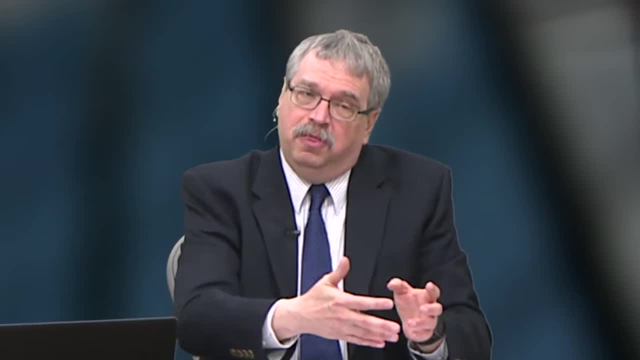 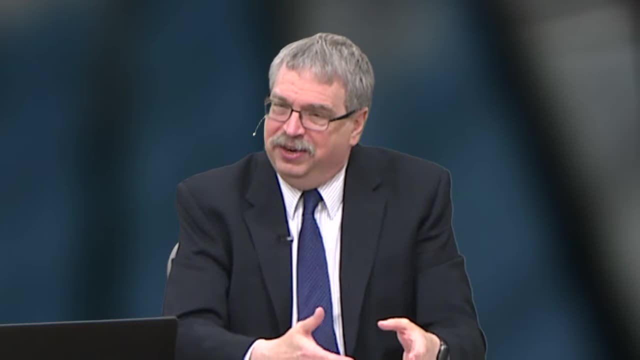 accomplish what you want, just to not have the buffer overflow. So I mentioned why the CWEs don't have as many of these kinds of things. We focus on it, MISRA focuses on it. We focus on particular elements to make things secure. 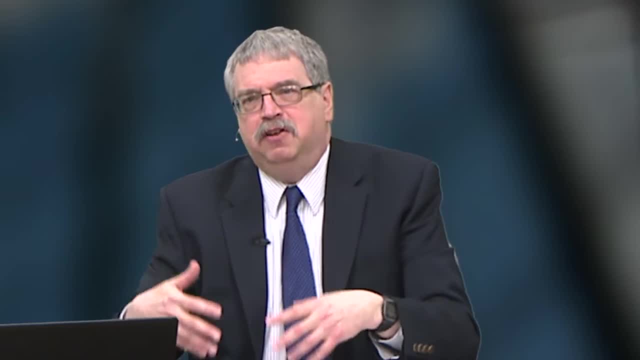 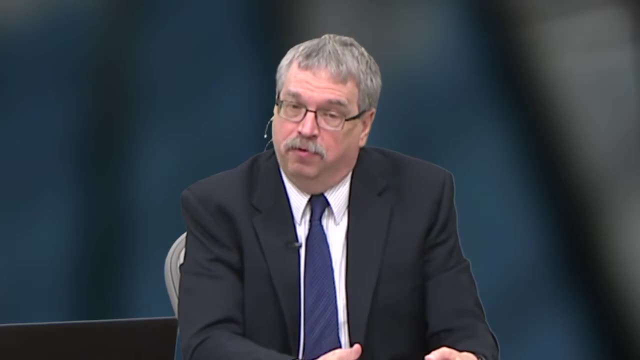 MISRA makes. MISRA focuses on particular things for safety in embedded systems. Just to give you an example: we worry about things like integer overflows, driving buffer overflows. They worry about running out of space, so their rules, for example, would include: don't. 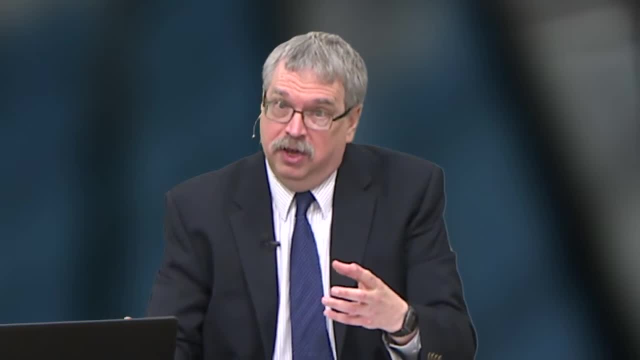 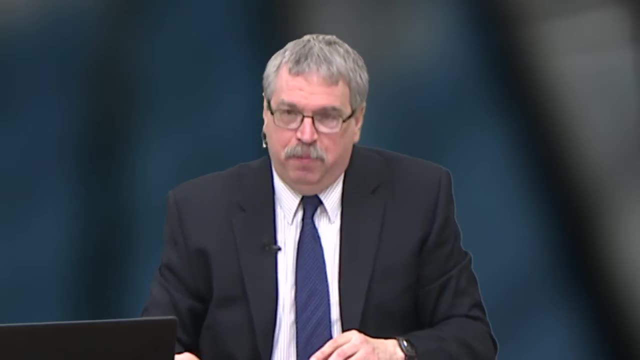 use malloc- no recursion in functions, things of that sort- as a way to maintain static memory allocation so that your card doesn't run out of space as it's trying to do some kind of thing. But the point is, these two sets of rules are actionable. 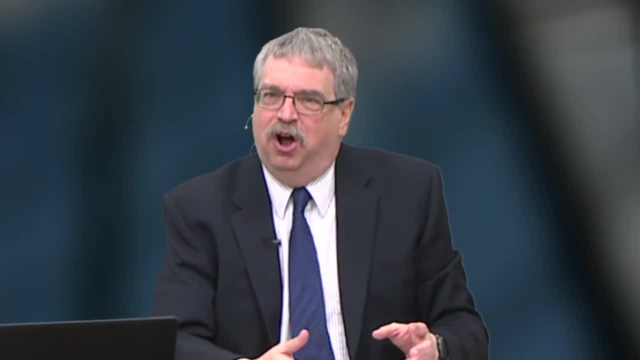 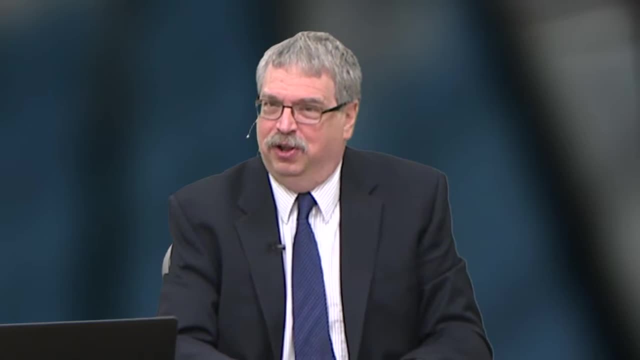 As opposed to many other sets of rules which are don't do something bad And for something like SQL injection. it's a lot more involved to explain to a developer how it is that you should code in order to prevent SQL injection. other than something. 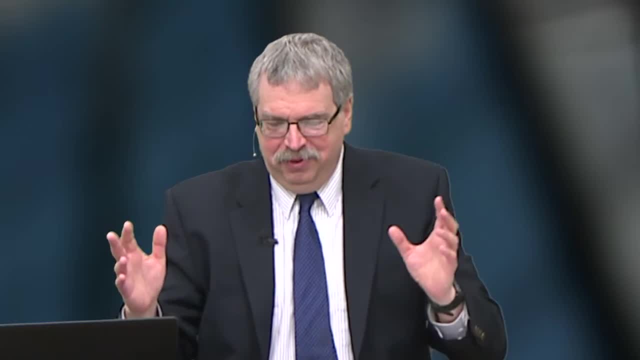 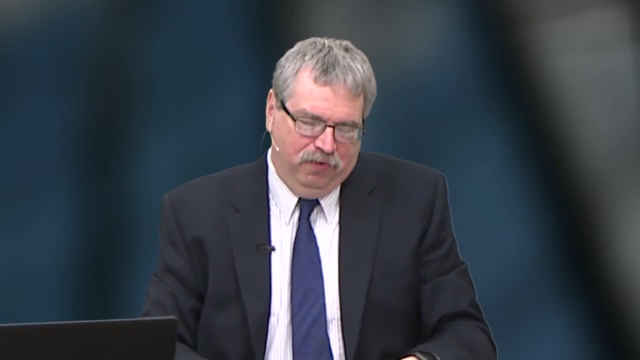 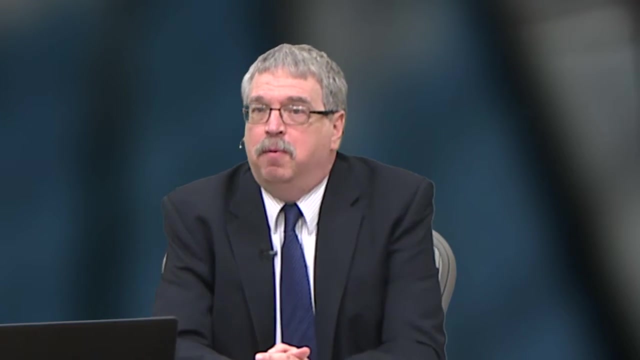 very overwhelming, like don't do any executable code, which is kind of difficult in today's environment where you want maximum flexibility. So how do we generate, How do we integrate these kinds of rules? Well, we actually have developed a methodology, So we've done this for a couple of languages and we can apply these to other languages. 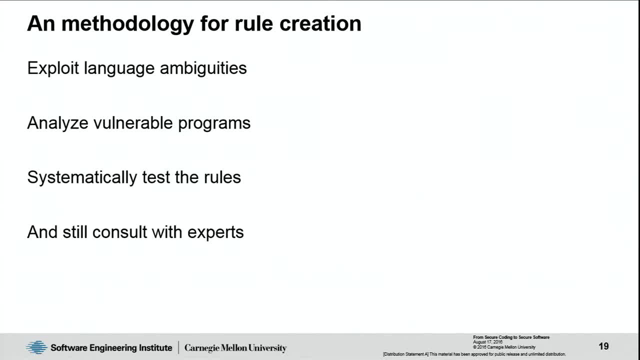 And if you wanted to build your own set of rules for your own company, you might do this as well. First, we look for ways to exploit language ambiguities. We then actually look at vulnerable programs. Where has things gone wrong? We create some rules and systematically test them. 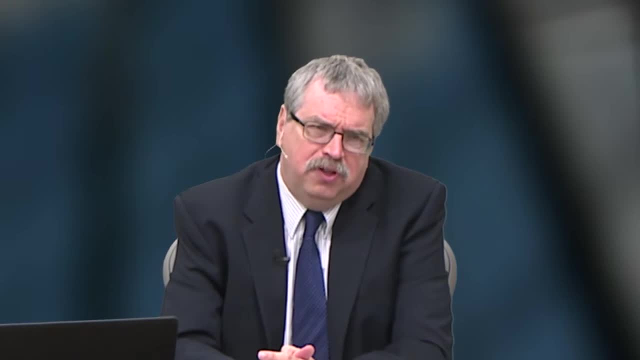 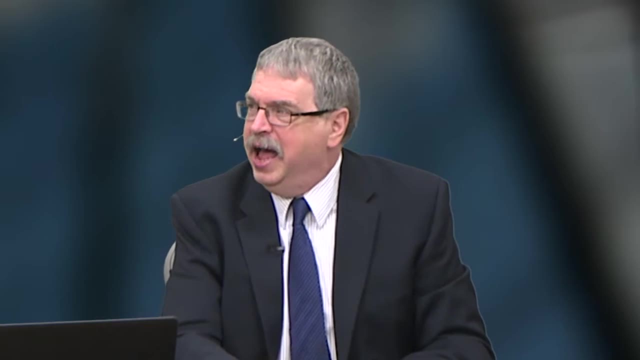 And we then ask for personal opinions from experts. Most of the other rules that we talk about You read are, frankly, just that last one: a group of very smart people that get together and say I think it looks like this, But then you wind up with these sort of generic rules of what can you do about it. 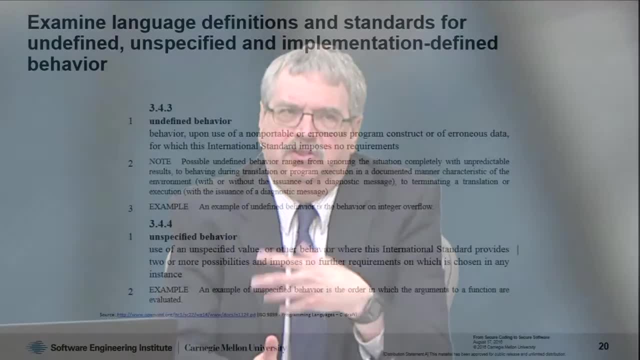 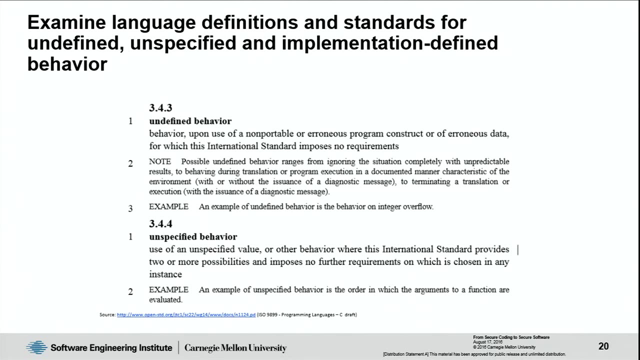 So, as an example, this is from C. The C language has things like undefined behavior, unspecified behavior, implementation, defined behavior. Each of those things, each of those ambiguities in the language, offers an opportunity for exploitation. Now They were put in the language. They were put in because different compiler writers for different architectures and different systems wanted to have different interpretations of those so that they could optimize the language for their system At the same time. that leaves open the other interpretations which can be exploited, sometimes for security flaws. 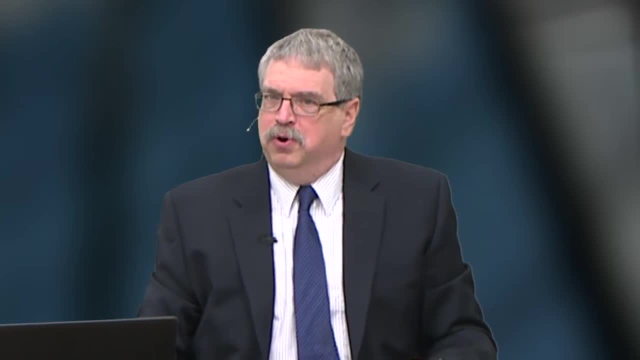 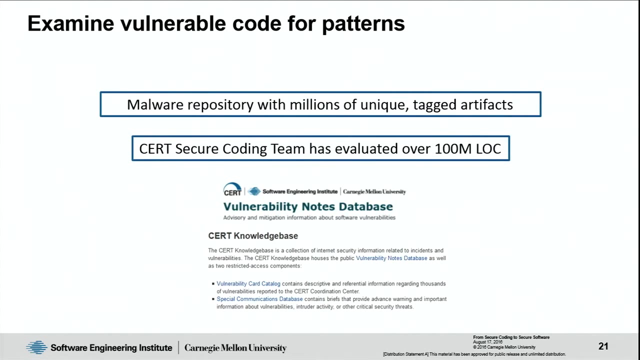 Second thing we do is we look at a lot of existing programs. We're fortunate in this respect at CERT that we have a huge malware repository And As part of our research work, we have evaluated a lot of code- over 100 million lines of code. 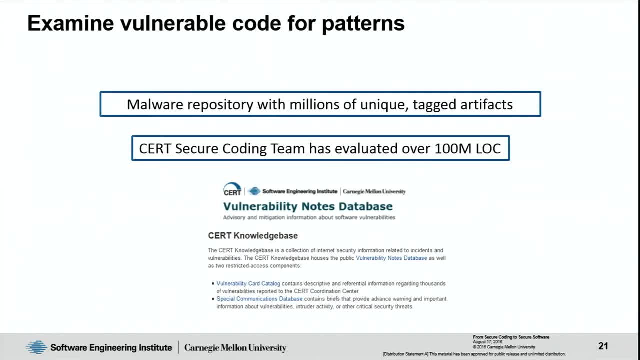 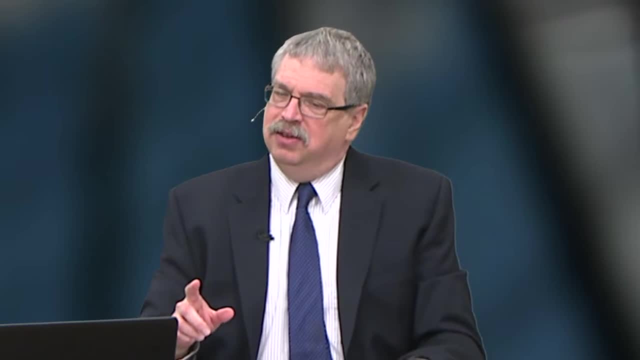 And so we have seen both other people's code and problems that have arisen in the security area, in that basically how the bad programming happened, And so that gives us the patterns of things to look for to at least advise people what to avoid. Having done that, we then take the next step, which is kind of tricky as well. is we then? 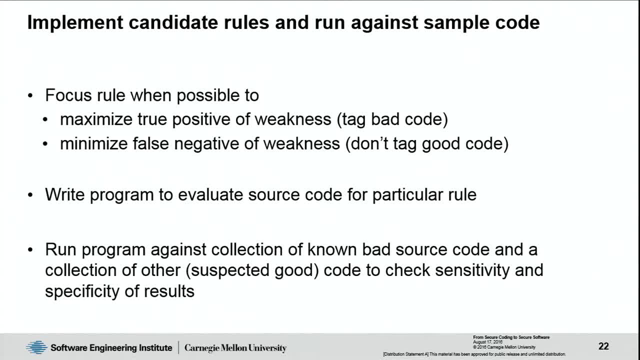 kind of come up with Rules. If you've used any of the static checkers- and I suspect many of the people have- the problem of false positives is endemic. You put something in and you get hundreds and hundreds. if you're lucky, thousands and 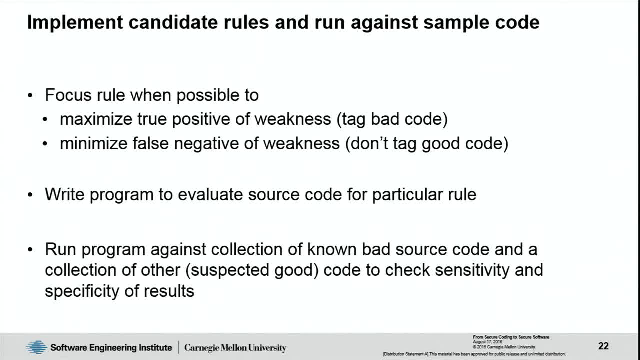 thousands, if you're not, of messages telling what's the problem with your code, And it's very difficult to actually then do something with that, And so the challenge is coming up with a rule that will maximize the true positives. You really want to find the bad code. 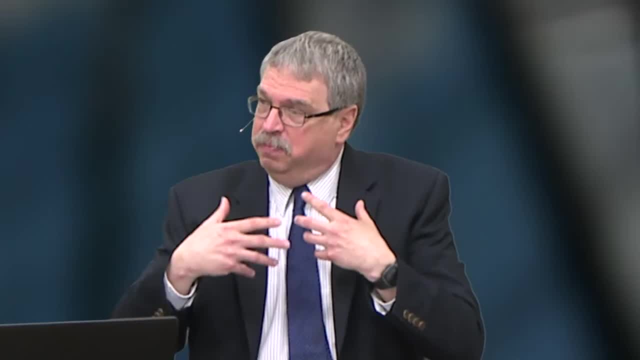 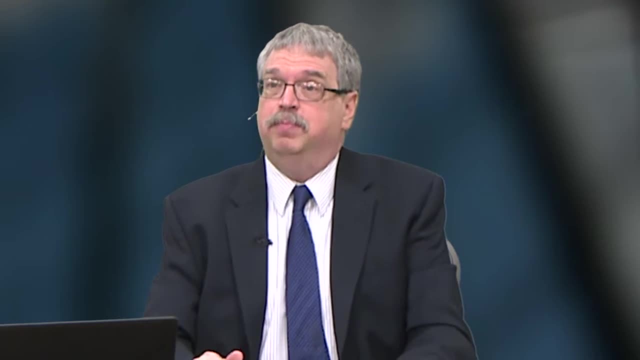 But You want to find the good code. So what we do is we generate some of these rules And, because we want them to be precise and concrete, we write a program that implements them and we run them over. a lot of code, usually about tens of millions of lines of code. 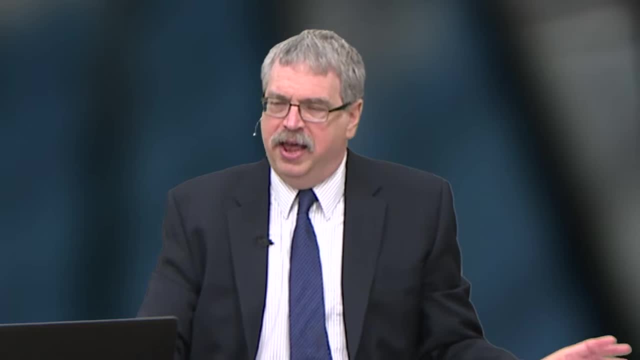 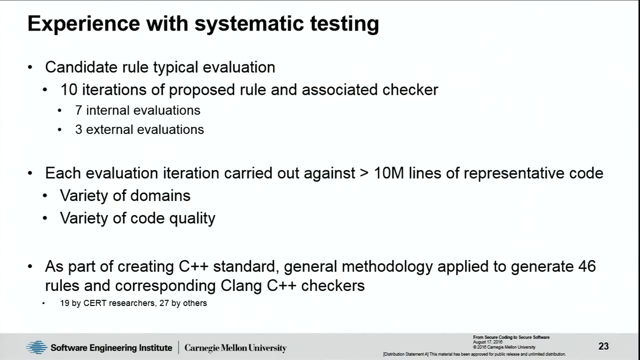 And we see what the results are And that sometimes we tweak the answers and then get something which is a lot more precise. For example, we typically do this ten times in order for us to get the rule right. if you're curious about our experiences here, 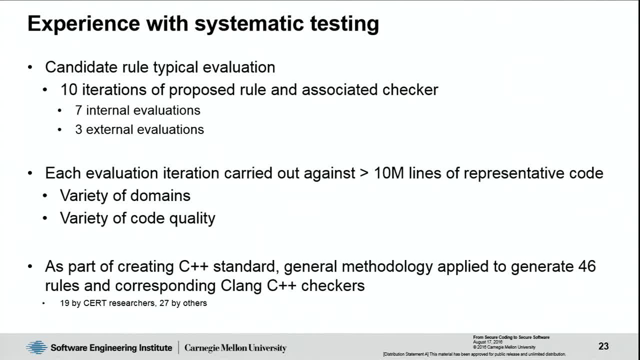 And As part of the Most recent standard that we're working on the C++ in about a year's time, we were able to, working with others, generate about 46 rules. So if you want to know what the how much effort's involved in trying to put something. 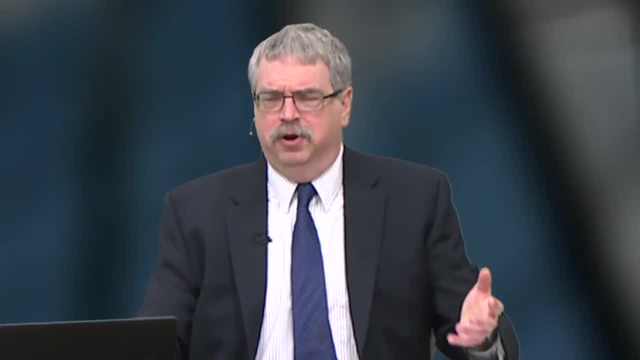 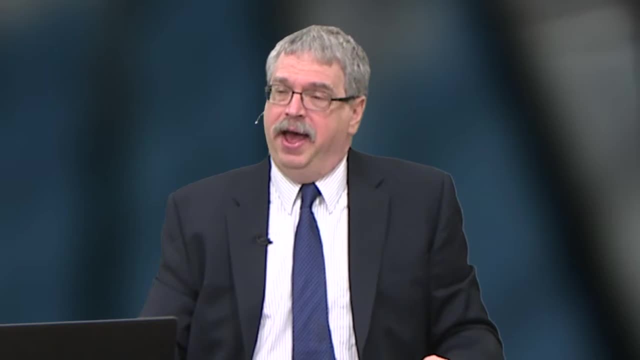 like this together. that's been our history here, And, of course, while we do the systematic analysis, judgment always comes into play as well, And so we do have a wiki that we invite people, experts and other practitioners to participate in. 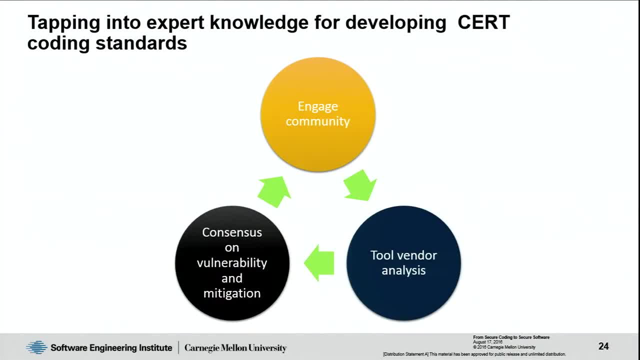 We'll probably talk a little bit about that more later, But it's a way for both people who want advice to see the discussions of the various kinds of rules and their implications, and for those who have advice to offer a forum by which they can share that knowledge. 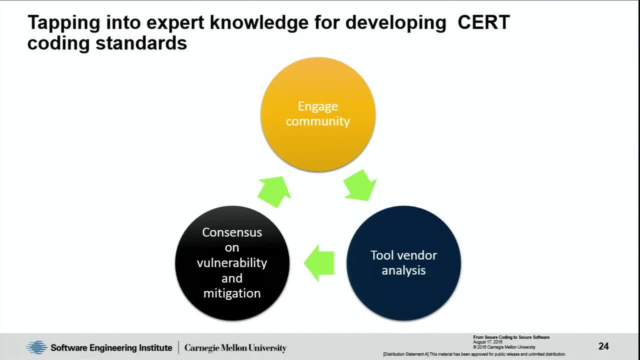 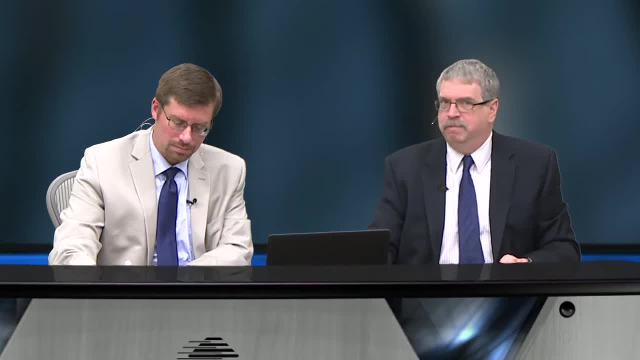 And of course, it feeds into our process for how we go about developing these new rules. And to give you some more concrete examples, I'm going to turn this back over to Bob and let him show you some of the rules. Yeah, Thank you, Mark. 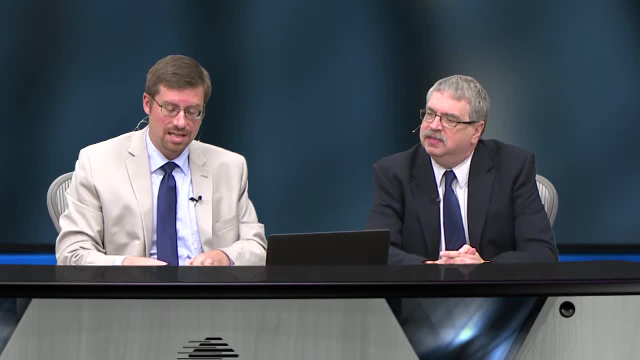 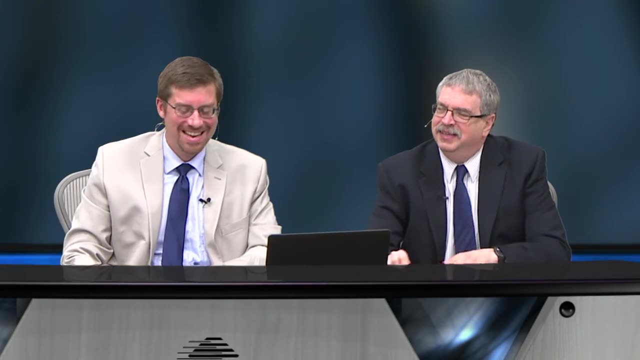 Before I say that, Let me, Before I get started with that, let me just say that I've been watching some of the comments and there's a really great discussion going on. Thanks to everyone for keeping it professional. There is. I'd love to throw in some comments on everything that's been talked about. 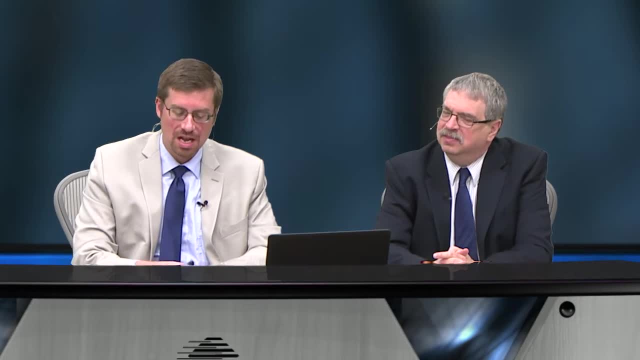 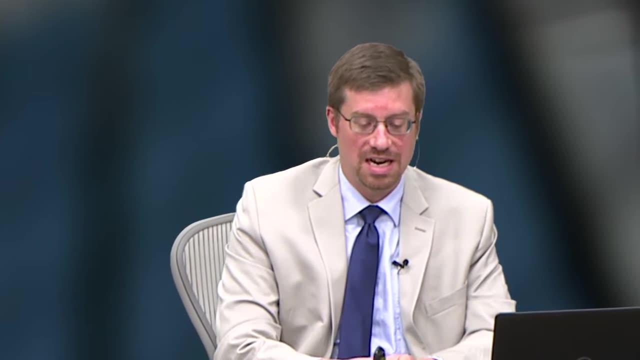 There's one in particular, though, that I really want to mention or refer to, a question by Brian about: aren't the C++ rules and recommendations marked basically with page warnings right now about them being outdated? We're actively updating the C++. 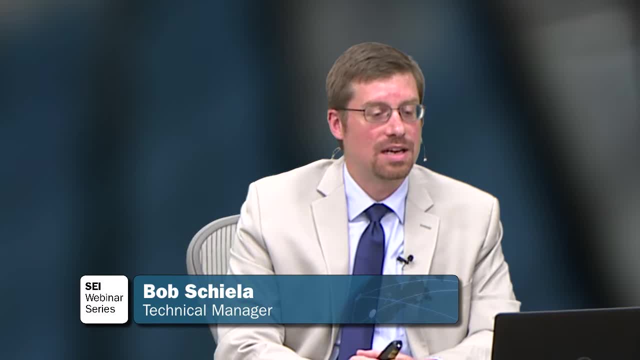 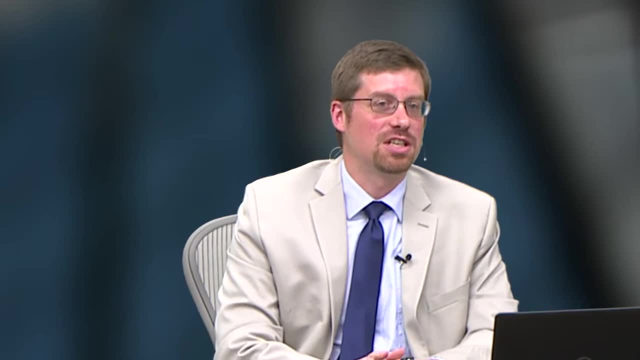 Yeah, We're updating the C++ wiki site right now And as part of that effort, one of the first things we did was went through and marked mostly recommendations- not roles, but most of the recommendations. We just noticed that a lot of them have not been reviewed in a while. 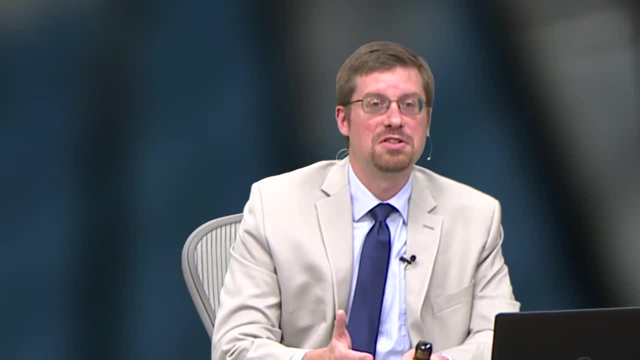 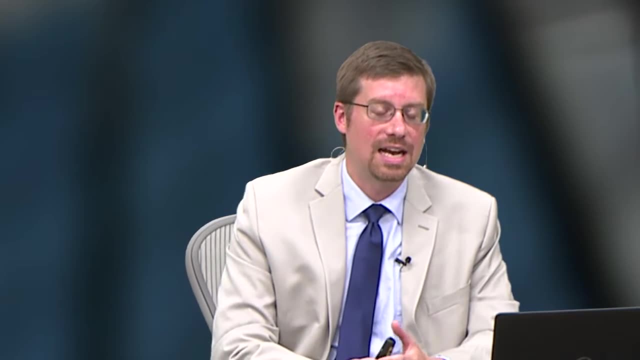 And when we reviewed them, we had some concern about some of the accuracy. And since we had to stage our efforts to update the C++ guidelines, we decided to start with the rules, Because those are the most important, And so we're working on those first. 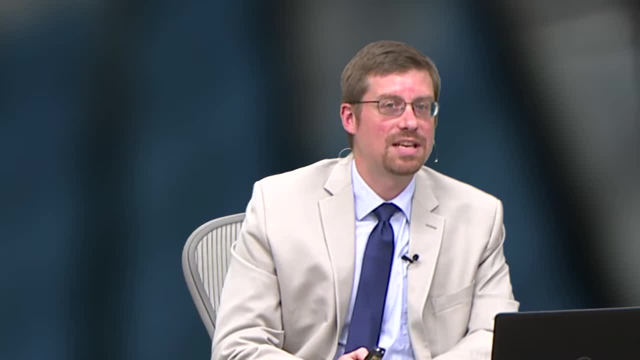 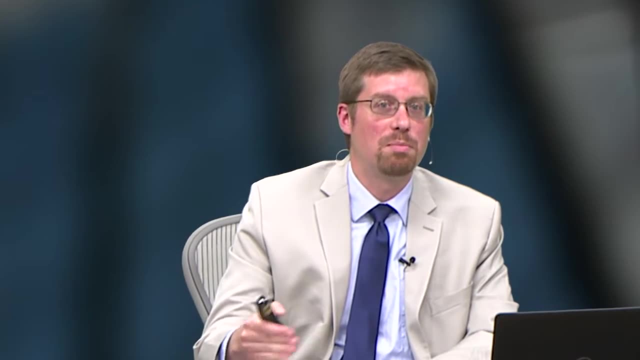 So you shouldn't really see many, if any, of the outdated marks on rules, Because we're updating those now And then, once we get to the recommendations, we'll peel off those warnings about the outdated nature of them. And you're welcome, Brian. 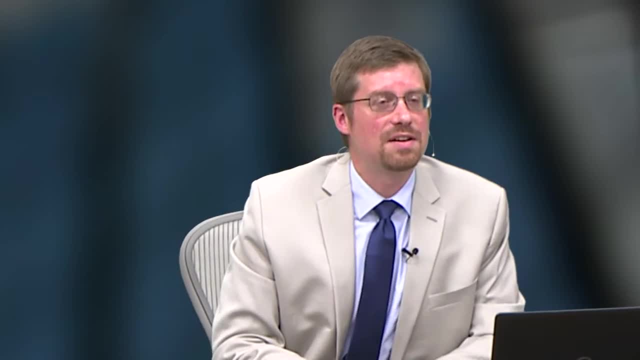 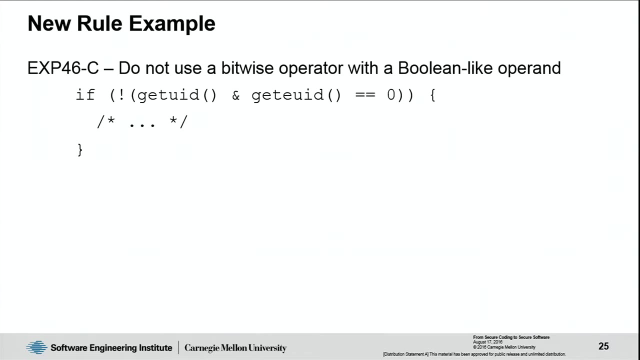 So, as Mark said, I'm going to just mention a couple of examples that I pulled from the standard. They're relatively simple Because we don't have a lot of time. We don't have a lot of time to go into in-depth code. 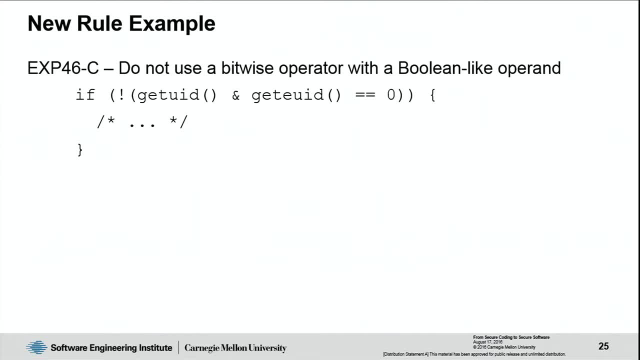 But these are two examples that I pulled out specifically that are in the updated C standard in the PDF, compared to the previous version that was published in late 2013, early 2014.. So this first one is kind of a simple piece of code. 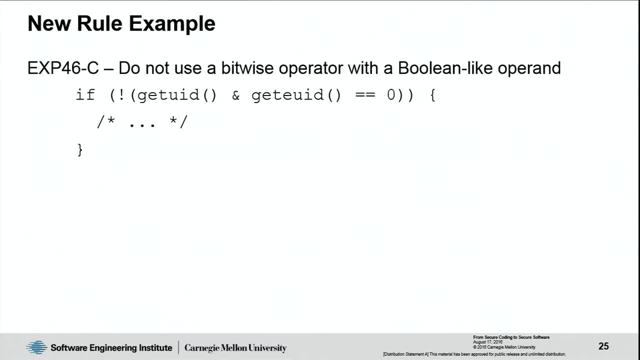 And here's the rule: Do not use a bitwise operator with a Boolean-like operand. And here's the rule. And depending on its use- I mean it's a conditional- So it might be used and it might go down a path that you're not intending, which might 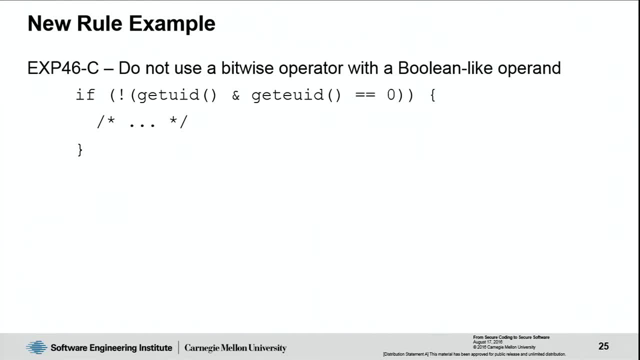 lead to a security issue, But it looks pretty innocuous. You see an and there And you see a comparison with an equal to. The issue here is that that's a bitwise and not a logical, and And it's a fairly common issue. 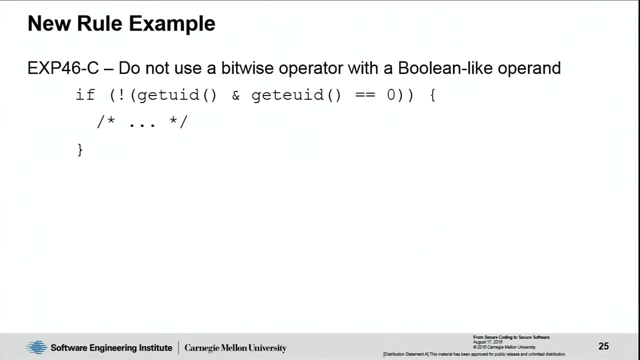 And a lot of static analyzers will find this, And so we added this as a rule recently. And just to show you the comparison, that's the fix there with the logical and. And this maps to CWE 480 for anybody looking against the CWEs, as Mark was talking about use of incorrect operator. 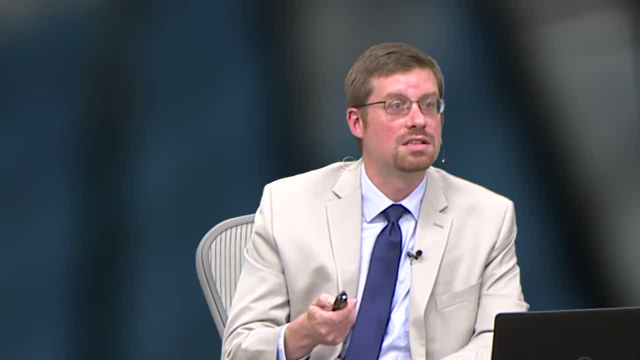 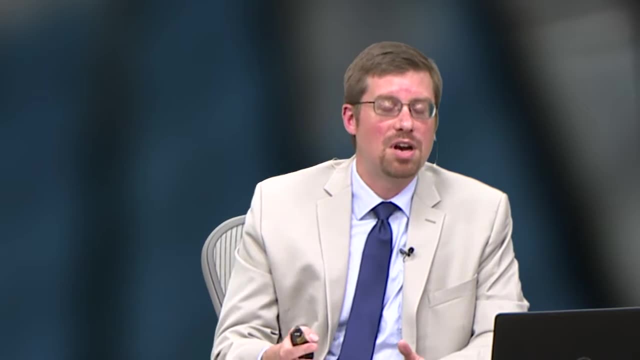 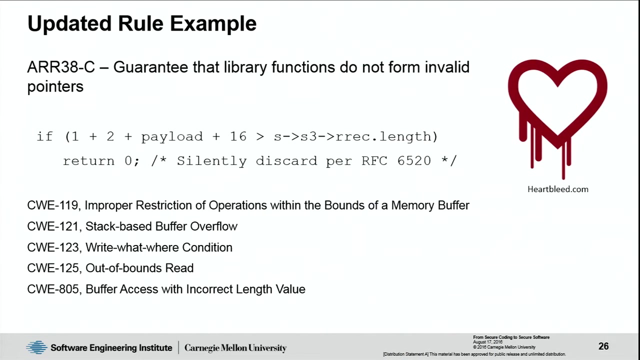 And so this is a rule that we have added within the last couple years. Another one that I have here, more so because of its popularity or notoriety, is related to the Heartbleed issue of 2014.. And so this is not a new rule, but we've also updated the rules in the comments and notes to keep them current when examples pop up that become fairly well known. 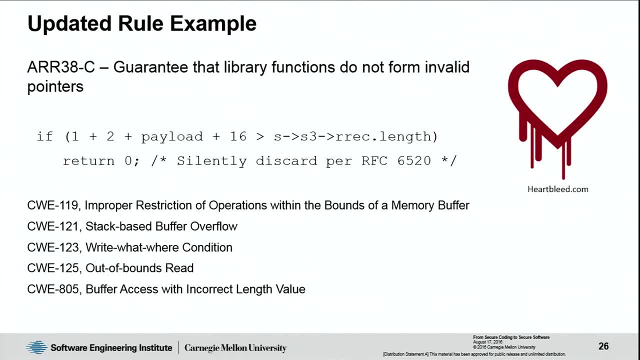 And so here we see, This is the the correction of the code. The issue is, as many people know, was that Heartbleed had was an SSH- or sorry, SSL- defect. where it was, you could query it with a heartbeat request and it would give you more memory than it should have back as a response. 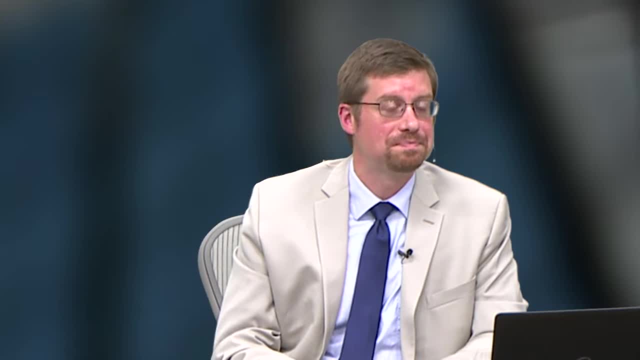 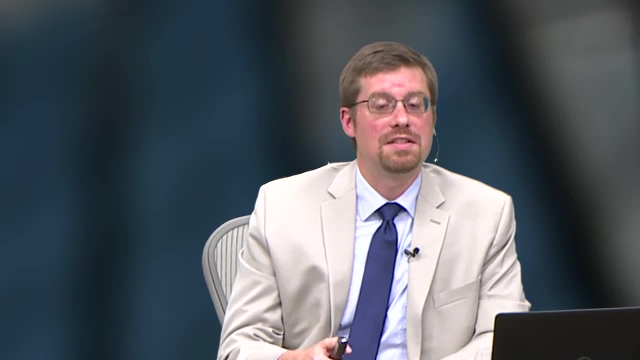 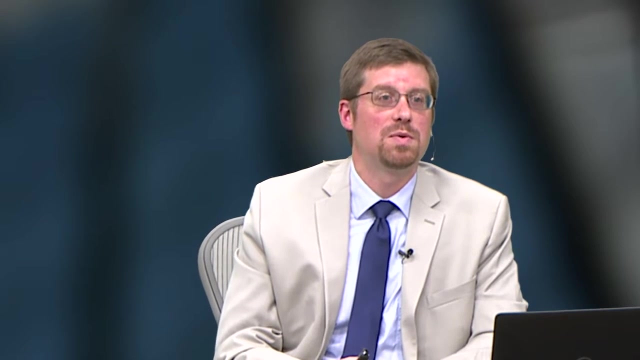 And it was basically an Information leakage issue and the reason was because they didn't have this simple comparison here. what it was doing was asking the user, or you know the code. it allowed a user to ask for a particular size and it didn't check to make sure that the size was asking for actually match the size of the buffer that it was supposed to to. to respond with: 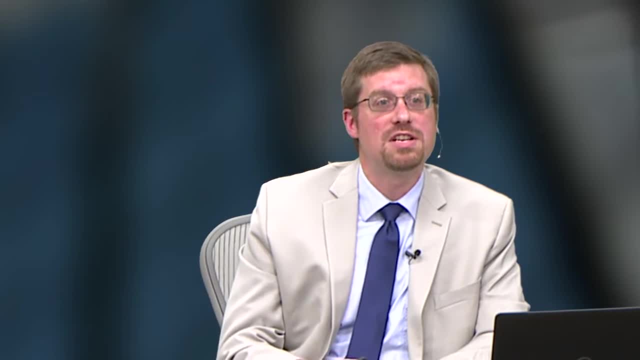 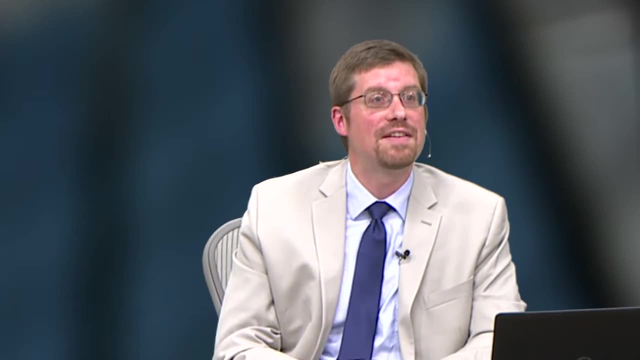 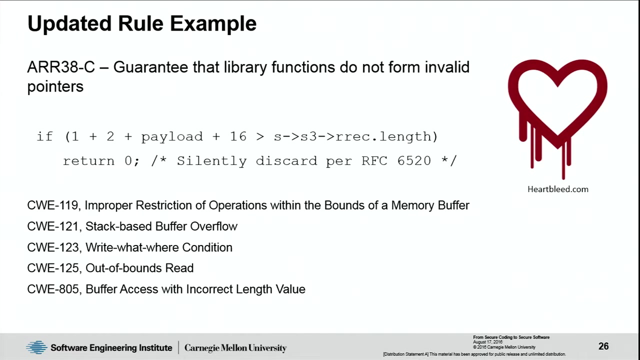 And so you could ask for a buffer larger than you should have been able to get access to, And it would give you information such as SSL keys and other other information that you shouldn't have access to, And all it required was this simple, this simple comparison: making sure that the payload that was asked, of the size that it was asked for, actually met the size of the buffer. 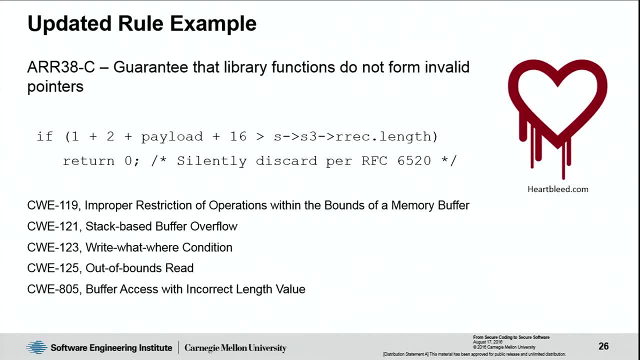 And so that again is not a new role, but we added a reference to this particular piece of code, And this role actually is a very long role. There's lots of examples and lots of nuances, But it also, as you can see, is pretty connected to or refers to several CWEs. 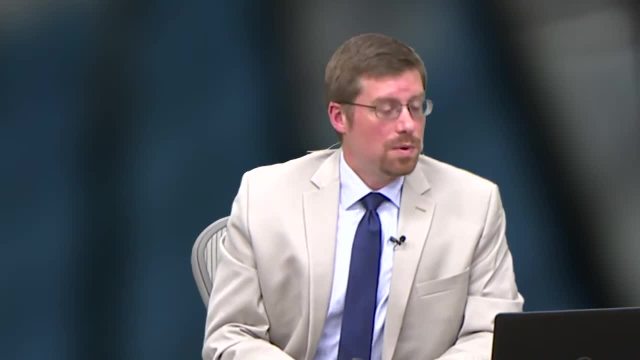 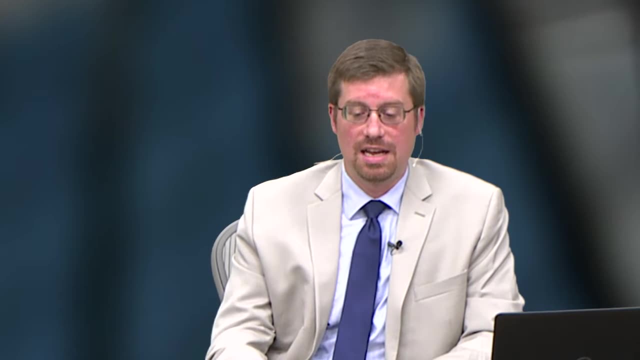 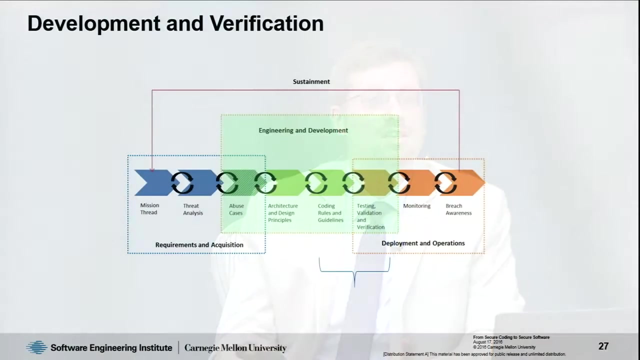 So now we're going to talk for a couple minutes about how can you use these roles and, in particular, secure coding and adopt, and So first again, just to kind of focus on where we are, here's our, our Secure development lifecycle, or software development lifecycle. 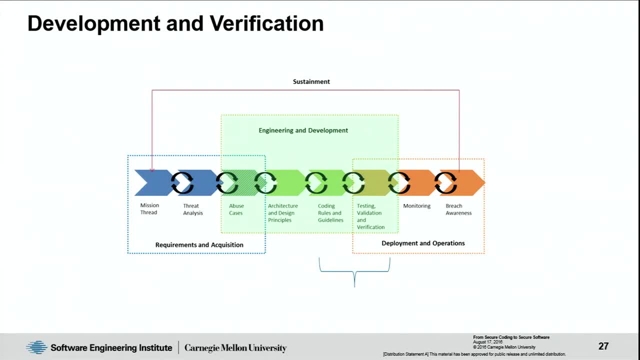 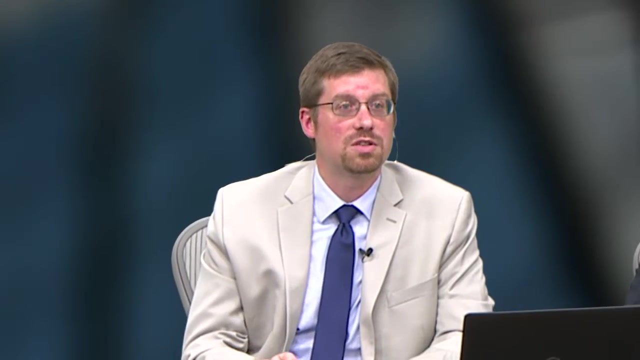 And Focusing On coding rules and guidelines and testing, validation, verification and, largely for secure coding, those are the development and verification is really where the action happens. So you need to know how to develop secure code and then you need to either be able to analyze it, review it, test it or know what secure code looks like, to verify that those practices and those coding contracts were used for the 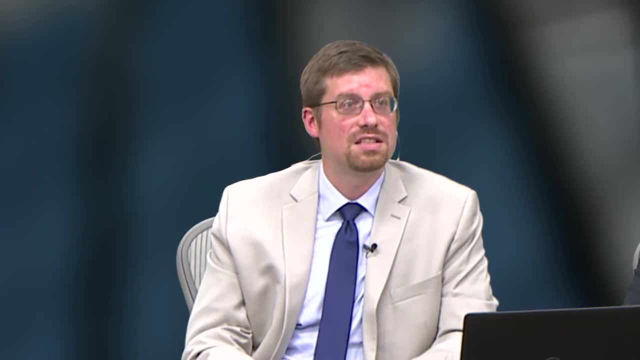 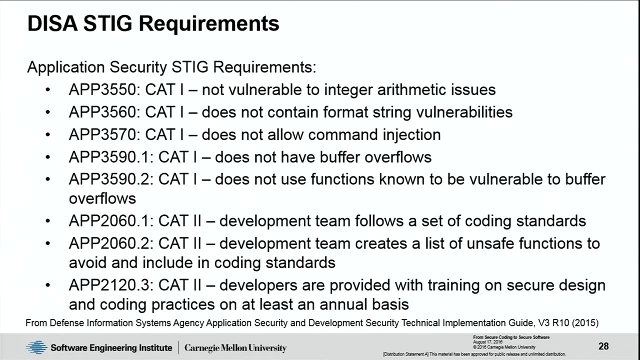 People on that are in the Go Government or, in particular, in defense that have to deal with this is Stig's. That's the defense information system agency security technical implementation guide. I just have this as a reference. These are just some of the Stig requirements that are related to our secure coding rules and standards. 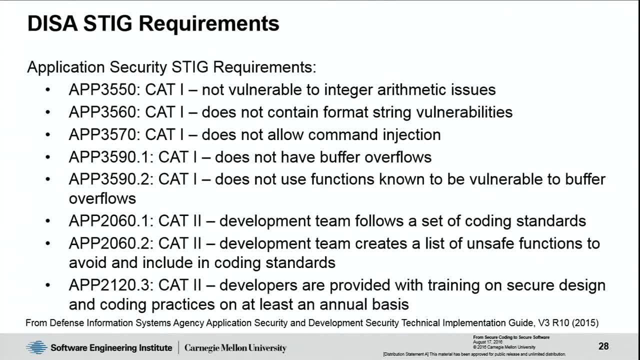 So if you're trying to and you notice there's several cat ones and a couple cat twos, you're trying to, if you're required to Address these, then following the standards are setting up a your own standards based on our standards will help to to affect that. 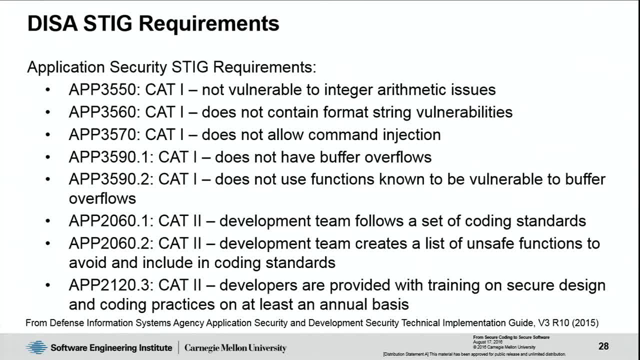 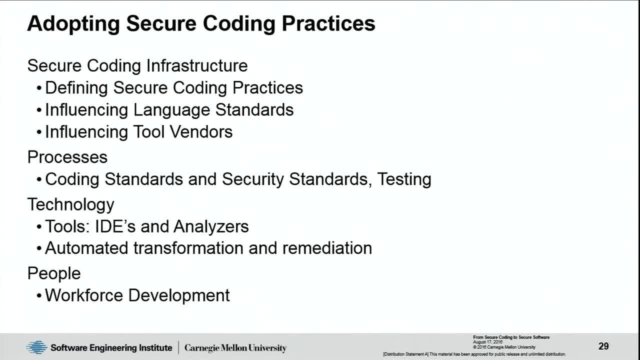 And you notice the lattice, or I'll point out the last one. there is it developers are provided with training on secure design and coding practices, and we'll come back to that. So, adopting secure coding practices- how- how to do that? well, we're trying at certain at the software engineering institute, we're trying to do a few things to help the 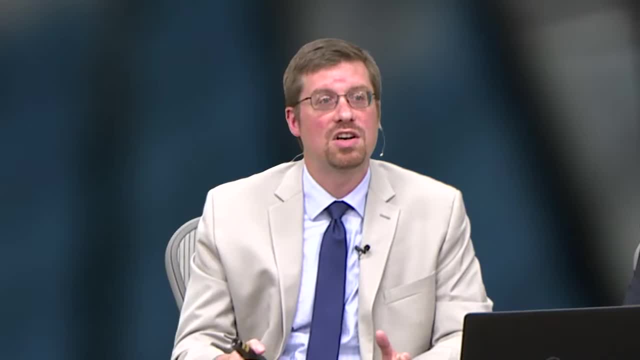 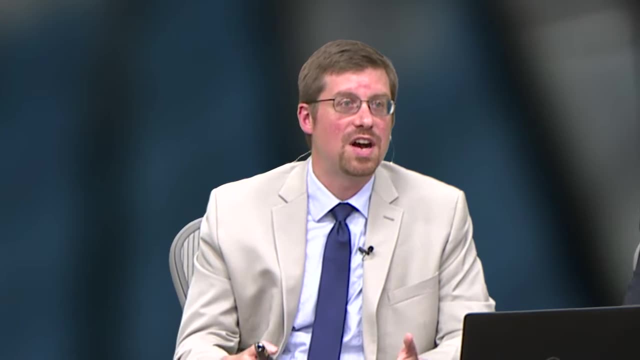 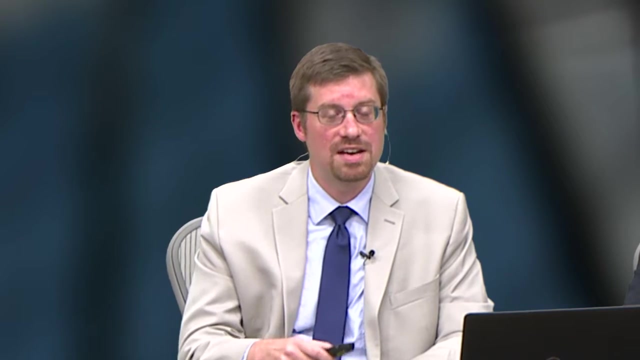 Community- and so I wanted to start with that just for a moment- of is what I call a secure coding infrastructure or community adoption. so, as I mentioned, we're we're obviously defining secure coding practices. we're also to help the Community adopt them. we're trying to influence language standards and, if we get a chance- I know there was some discussion on the chat about different languages and maybe we'll have a moment to talk about the languages, although it seems like other commenters have addressed some of that. 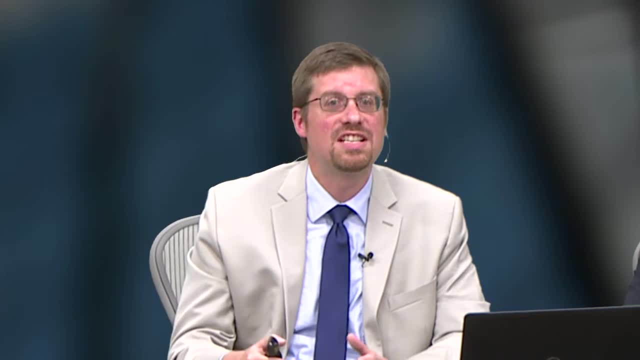 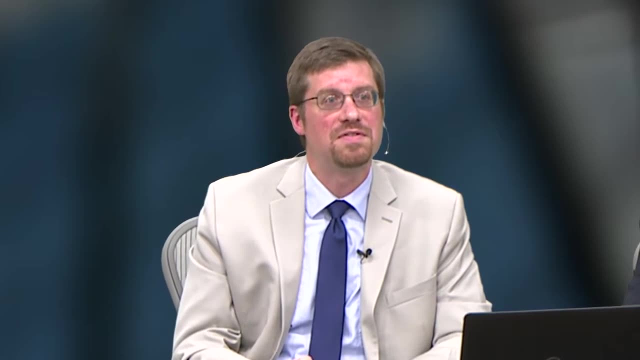 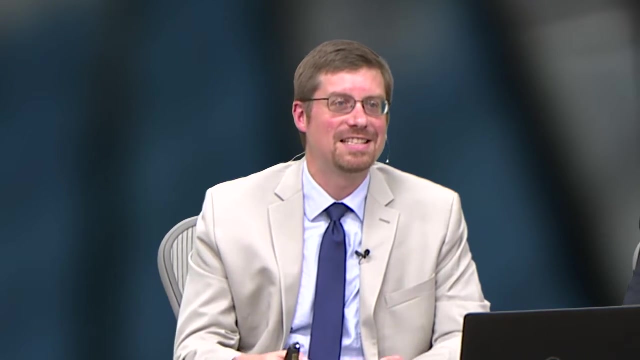 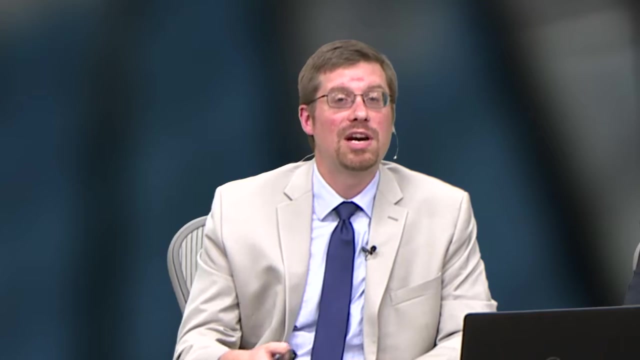 But we're trying to influence the language standards so that they adopt secure code. are you improve the language itself to to make it easier for developers to develop secure coding? And we're also trying to influence the tool vendors. the tool vendors are also connected to the language community, so it's not too far but trying to help the tool vendors and or help people's awareness of the tools that can help their their secure coding. 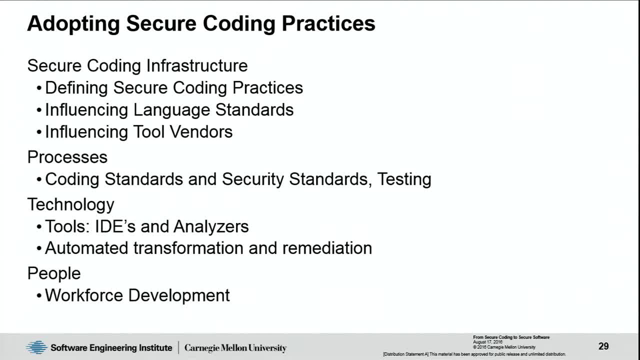 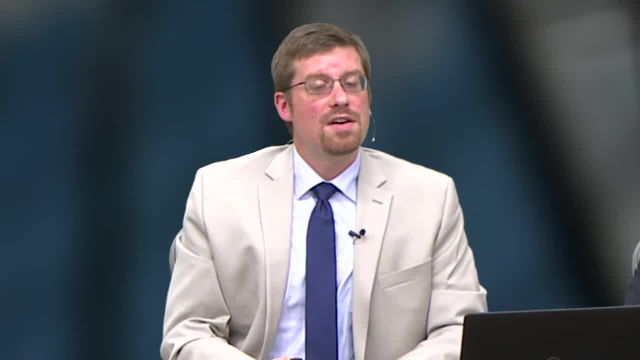 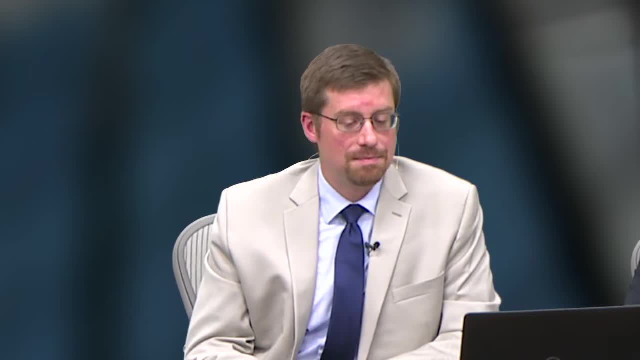 And so we'll talk a little more about processes, code coding, standards, technology you can use, and and workforce development and training. So, one of the issues with adopting this and improving your practice- well, I'll start, you know, and this has been commented in here- we will talk, you know, or I'll talk for a couple minutes about developing your own. 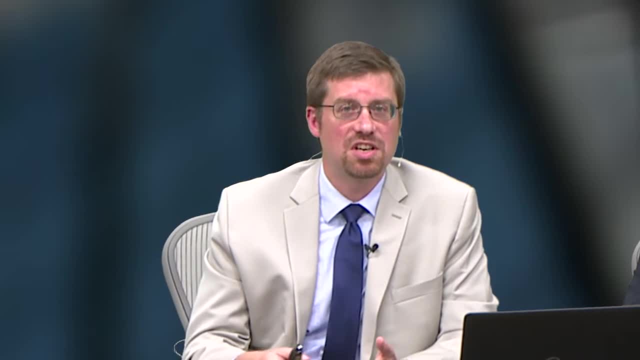 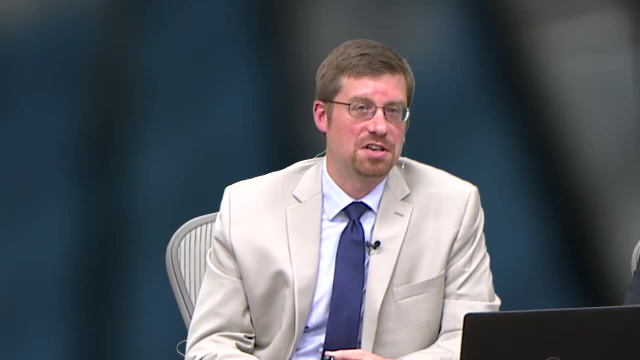 Standards. so developing your own security coding standards with something to base off, like ours Is, is a really good start. The problem is, it may seem overwhelming at first because the security coding standards are fairly voluminous. there's right now, I think, there's ninety, nine C rules that you should be following. 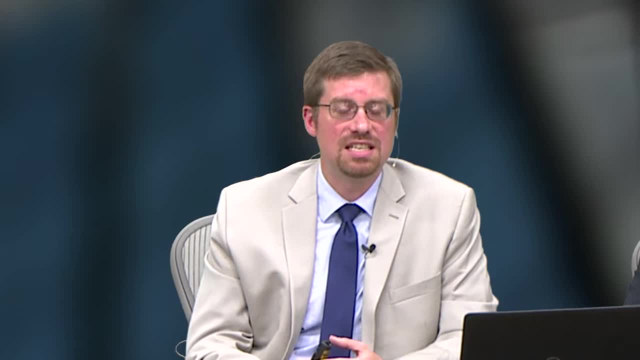 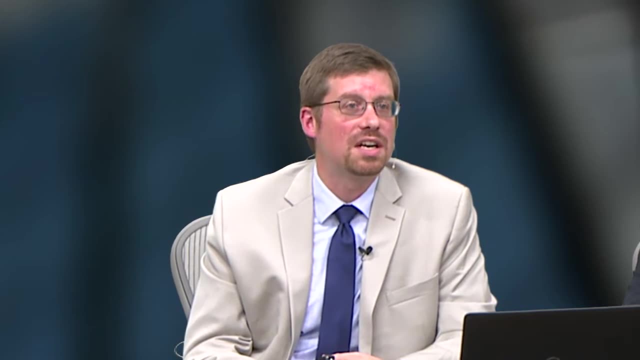 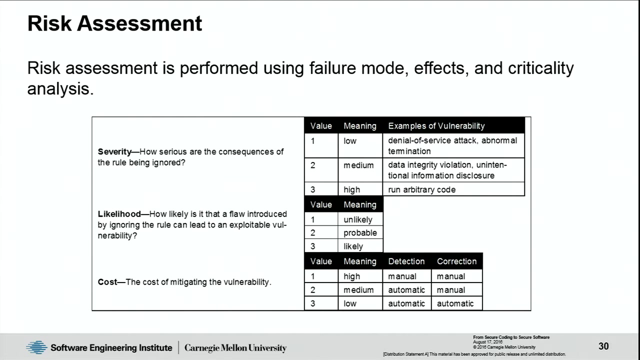 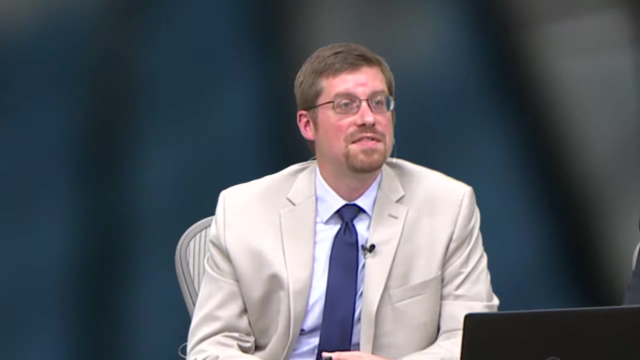 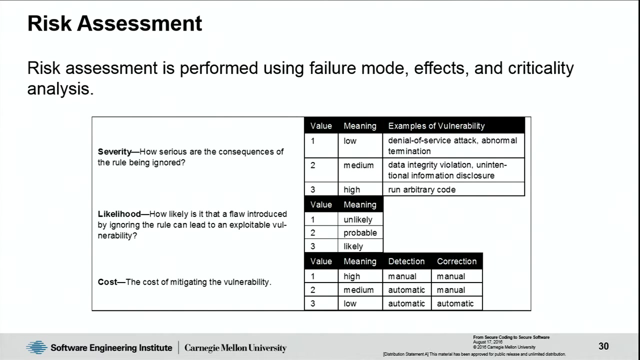 So one of the challenges is to prioritize those, especially when you're trying to adopt them, and so we have a few mechanisms of guidance of how to prioritize. one is we have a risk assessment, And so the risk assessment For each role provides a value of how risky a, a defect or a weakness related to that role is, such that it's likely to to end up as an exploitable vulnerability. and so here we have this rating, and it's on three different dimensions: severity- how, how bad would it be, and how, how exploitable, or what would it. 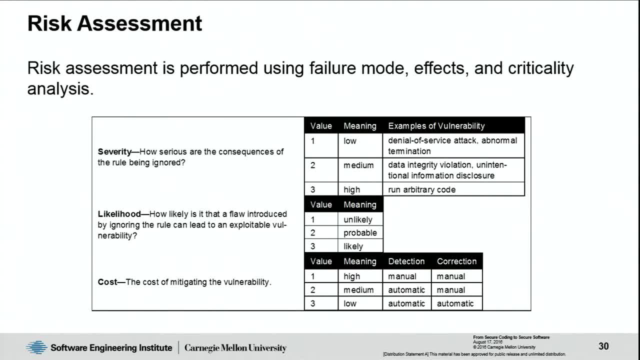 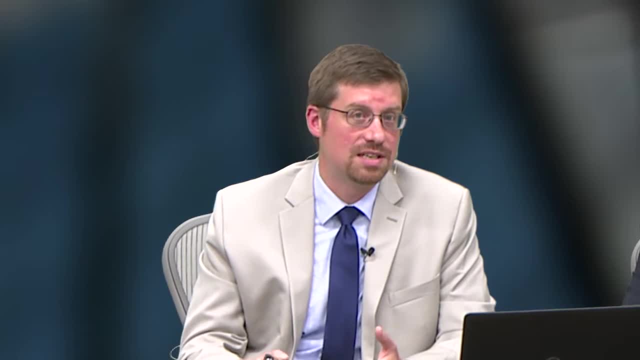 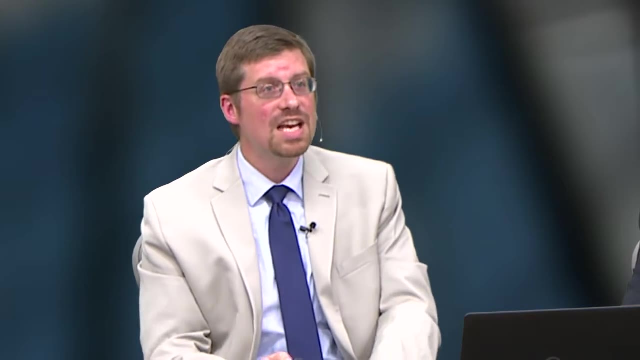 What would the effect be, the worst being running arbitrary code and giving control up, The Likelihood being another dimension. and then the cost of remediating or mitigating, which is how hard is it to find and or fix? and, as mark mentioned, a lot of tools give out a lot of false positives. so finding can be a challenge, or as much of a challenge, if not more, than fixing it once you find the issue. 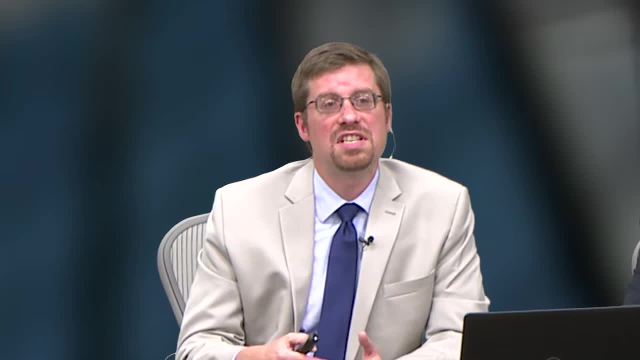 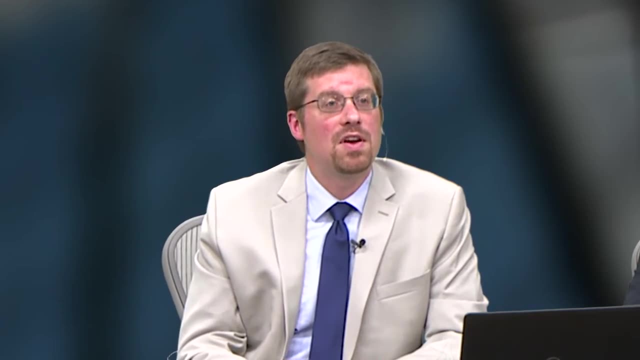 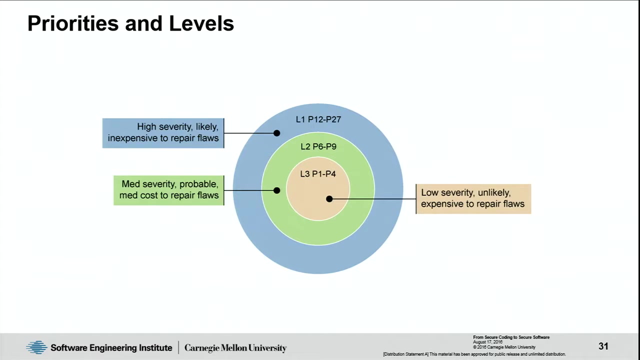 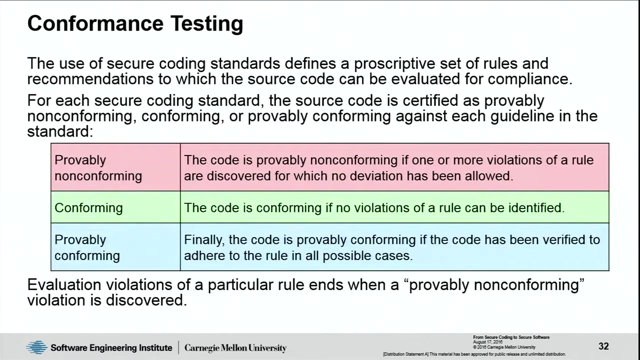 And so you can use our risk assessment on these rules to decide which rules you're going to first adopt, because they're the highest priority, And so We map those into these priority levels just to make it a little easier, rather than having twenty seven and and the actual numbers are a little less, but. but there's three different ranges for the priority levels of rules. 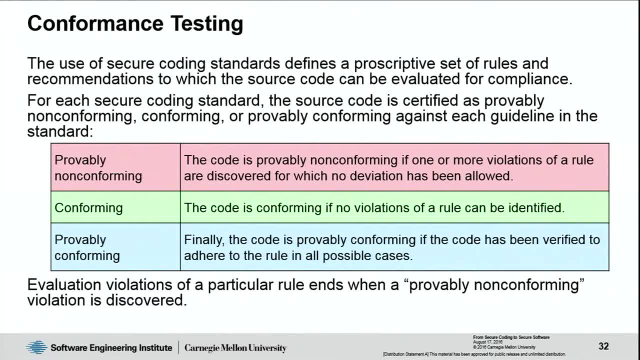 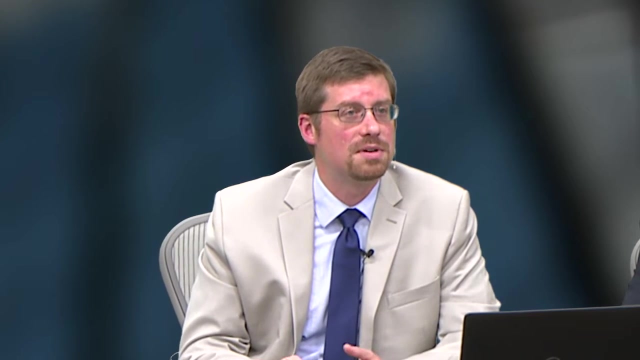 What you also want to be trying to do, ideally, is looking for code that conforms to the security coding standards, or the security coding standards that you choose to adopt, And so that's kind of the The goal of Of analyzing and and verifying your code is you're looking to conform it? because looking for conformance? because conformance means that the software will be much more secure because it won't have these weaknesses that lead to vulnerabilities. 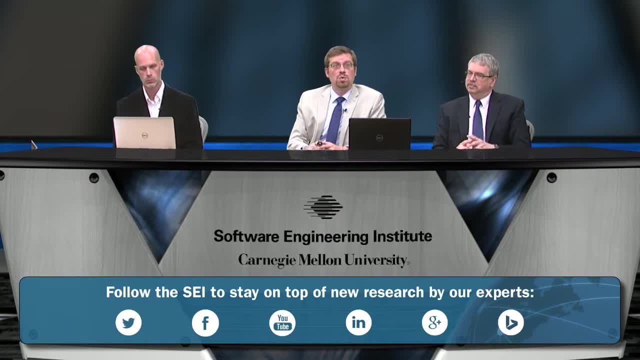 With that and before we get started talking about tools and analysis- and I know there's already been some comments on On On On the chat about that- I was wondering if we could find out more about what you use to analyze currently in your processes. 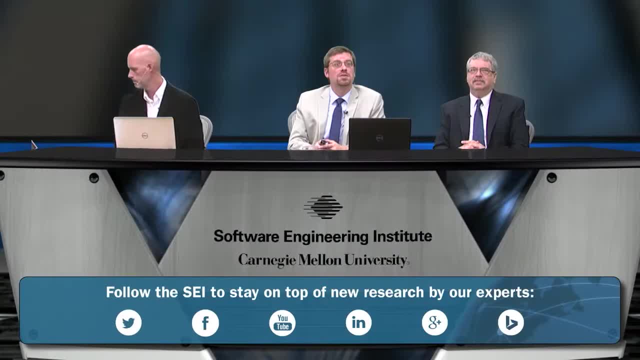 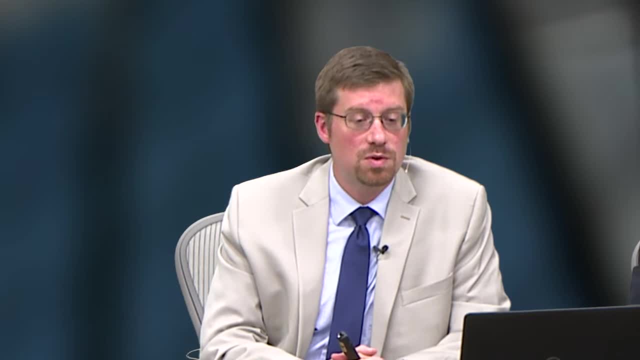 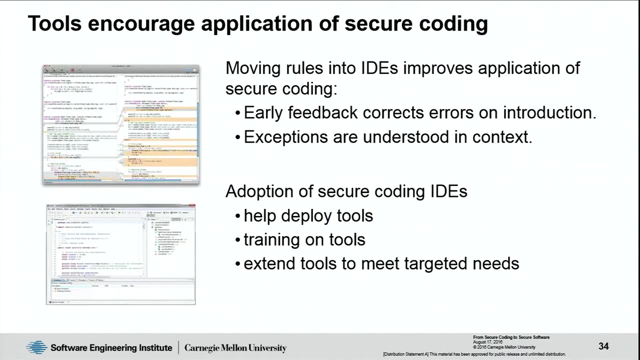 So that question is posed and we can wait for some results. Sure, sure And so. so now to talk about tools. the first, The first tool that a lot of people don't think about is the idea itself, the environment that you're developing. those tools can provide warnings that can be really helpful to 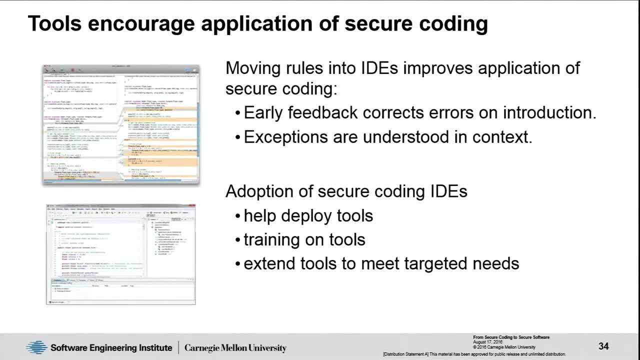 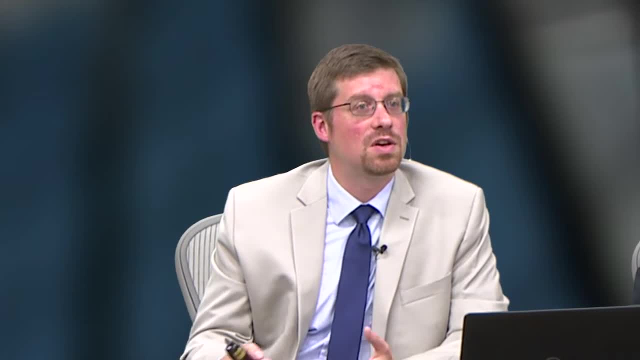 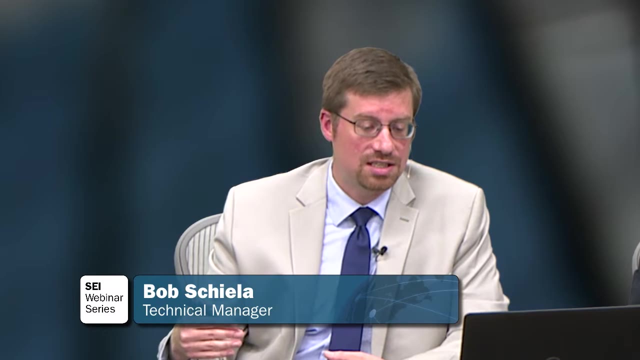 To To To at first. First site find and fix some, some simple issues, and so we absolutely recommend looking at those diagnostics from the ideas. Ideas are getting smarter About presenting information to the developers, and so are. what we're trying to do in some of our research is align our diagnostics, or diagnostics the tools find related to secure coding vulnerabilities. 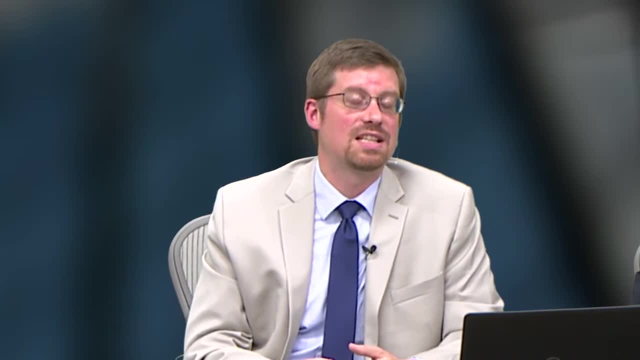 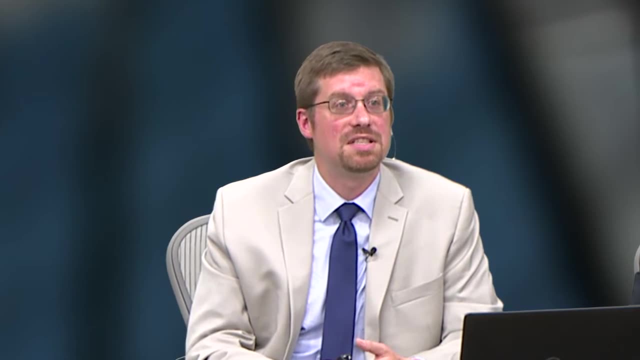 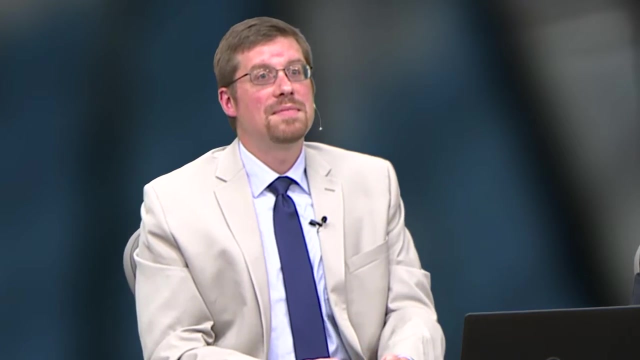 And present that to the developer while they're coding, because finding and fixing them, of course, earlier in this in the life cycle is cheaper, but finding them right when they when they write them, is the cheapest it can be because they're already presently. you know mind is present in the code they're writing. 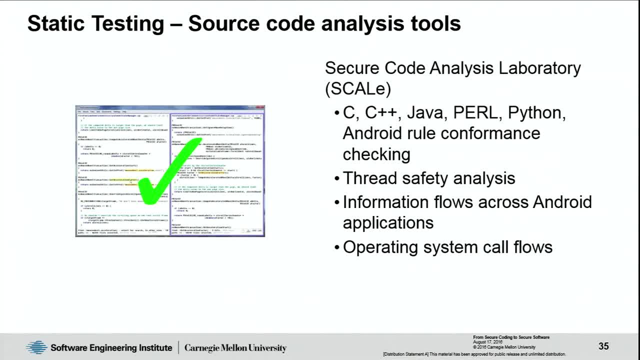 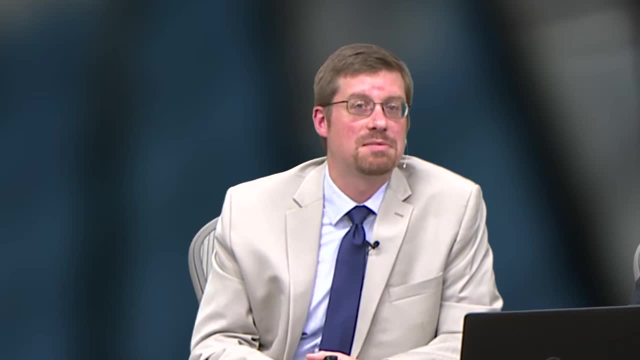 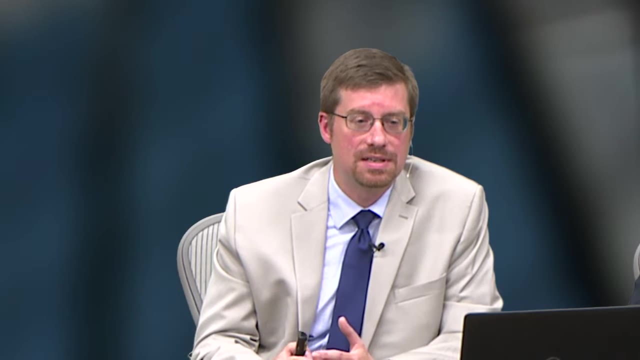 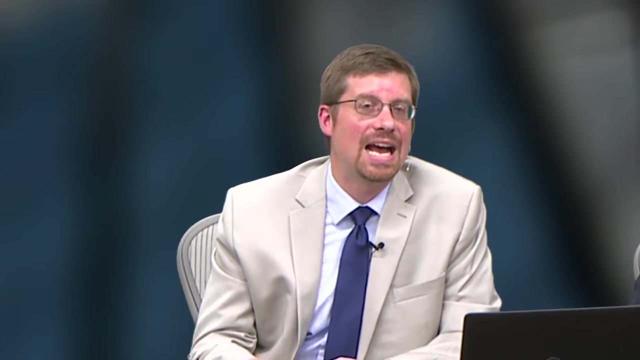 Static analysis is definitely a practice that should be used. there is a question about one particular tool, whether or not it's good enough. We have a recommendation that No tool has complete coverage. every tool Has. it has prioritized or optimized particular types of defects that it's trying to find with really high accuracy to try and reduce the amount of noise of false positives. and so that's where they're. they're market differentiation is what they're trying to find. 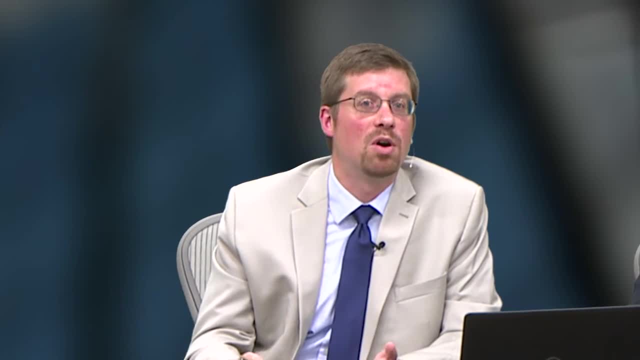 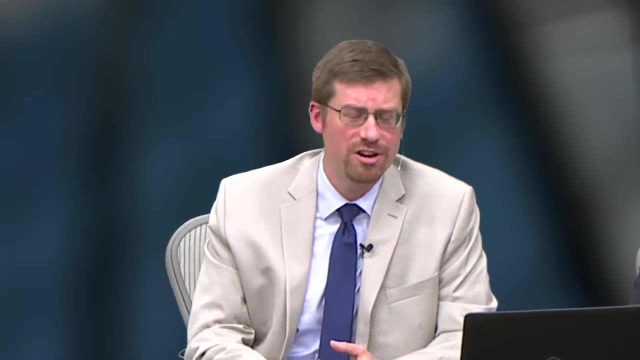 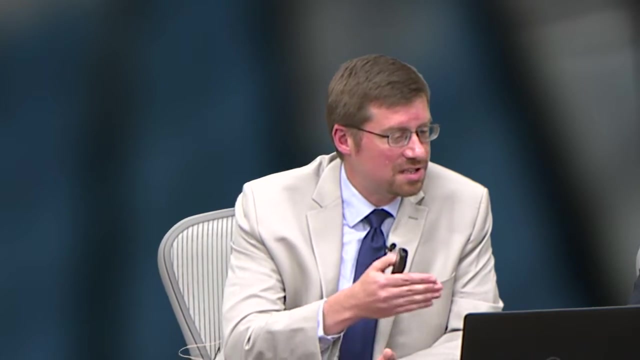 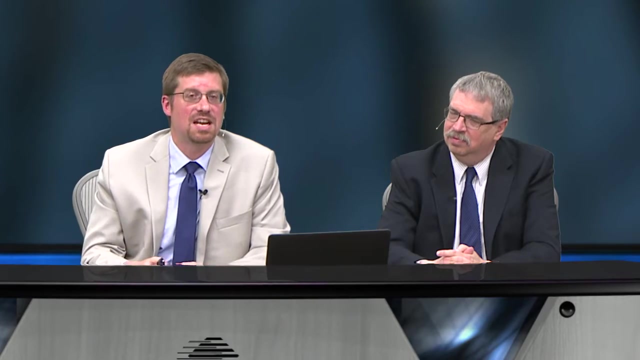 And So we recommend that you use multiple tools and, as I said, consider your idea, your development environment at all, or even, if you're programming in GCC, just running it with diagnostics. Similarly- and Mark mentioned this, was also some discussion in there about how different languages are optimized for different things: some for speed, some for safety and protection. 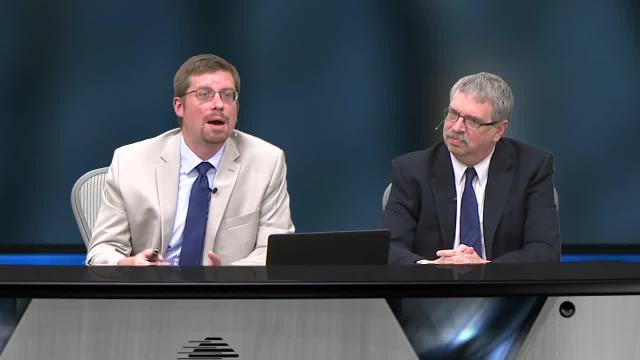 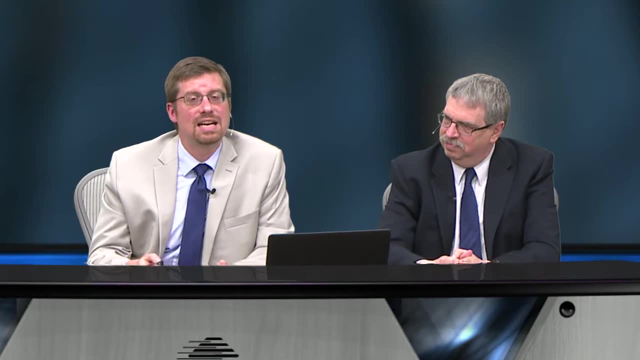 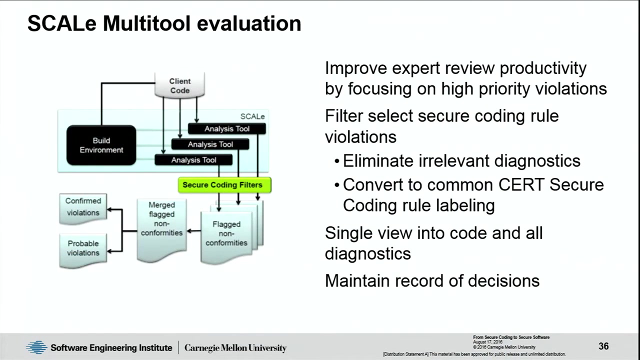 The static analysis tools and even the dynamic analysis tools are optimized For different things. now, of course, if you're, if you're running multiple static analysis tools, you have multiple environments where you're getting lots of diagnostics, and so we also recommend using a diagnostic aggregator of some sort. there's a few on the market. we also have a research tool, and one that we use whenever we do audits ourselves, called scale, the source code analysis laboratory. 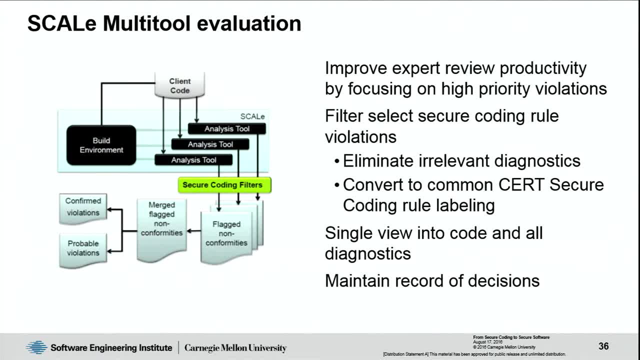 And what that does for us is. it is, you can see from the the graphic there- we run multiple analysis tools and then we run it in through scale, which first Runs it through some secure coding filters to help us prioritize the diagnostics it found related to security, as opposed to style or or other issues that are unlikely to be affecting security. 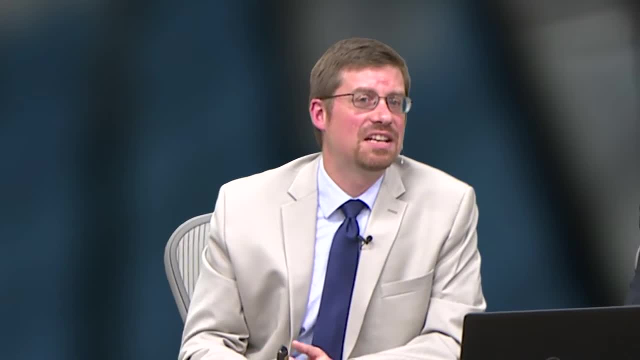 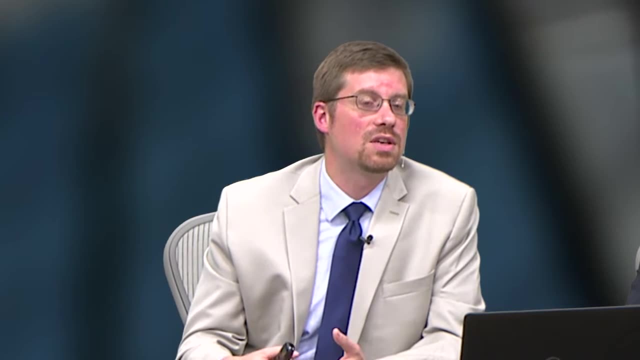 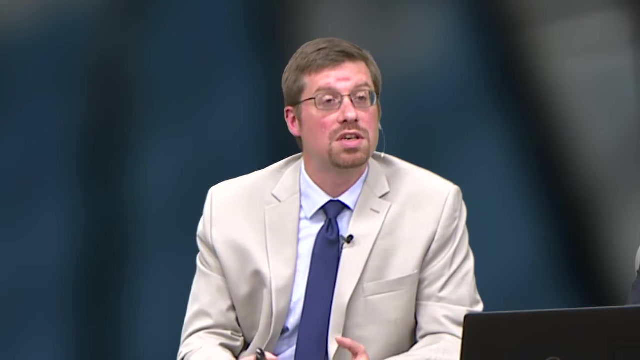 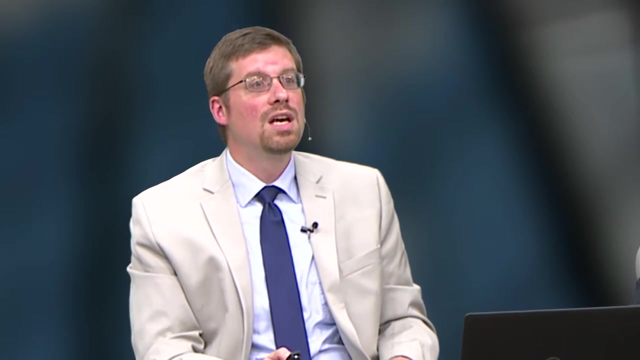 And then It aggregates all of that Data so that we can all the diagnostics of the tools, so that we can review and audit the code in one interface and with one data set and database, and it also connects us directly to the, the source code, to easily find the lines of code that that the diagnostics are pointing to. 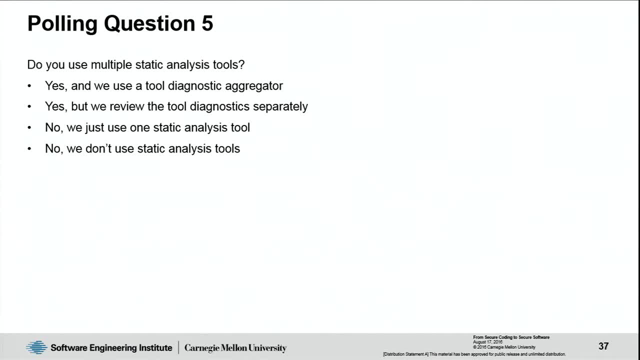 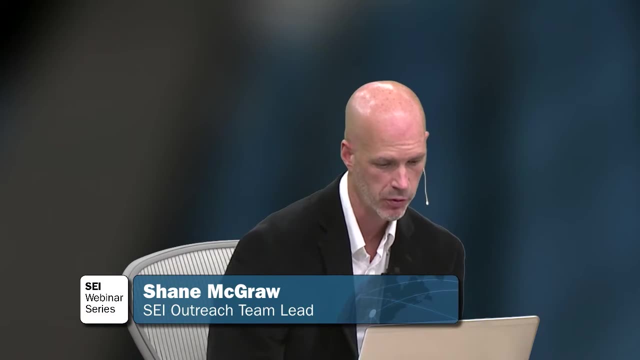 And so with that, as I mentioned, I'm curious to find out about our audience, what they're doing currently with static analysis, If they're running multiple static analysis tools and how they are so, so that questions pose and we'll give the results here from the last one. the last question was: what testing does your organization perform on your software? we had forty four percent with static analysis. 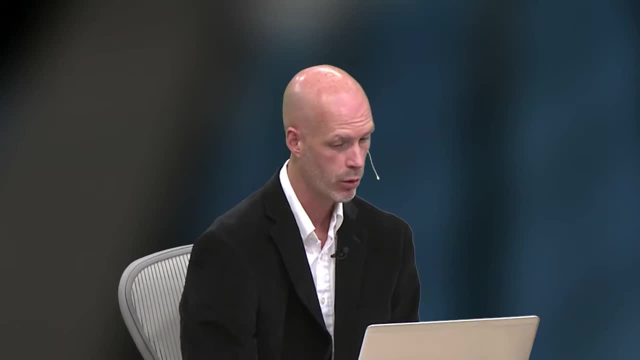 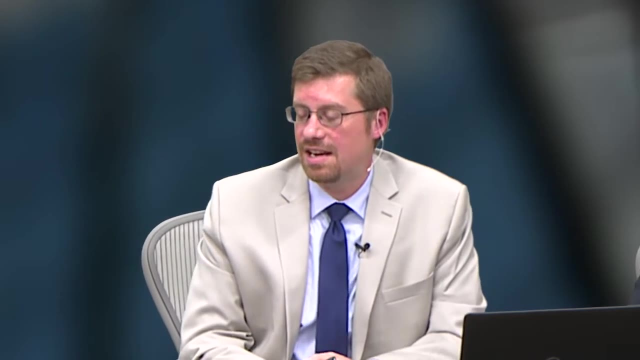 Four percent with dynamic analysis, forty one percent with both, twelve percent with none. okay, so next one's launch. so back to you. yeah, so I will. I'll just mention that dynamic analysis. I'm not going to talk about it too much. we do have a group here at 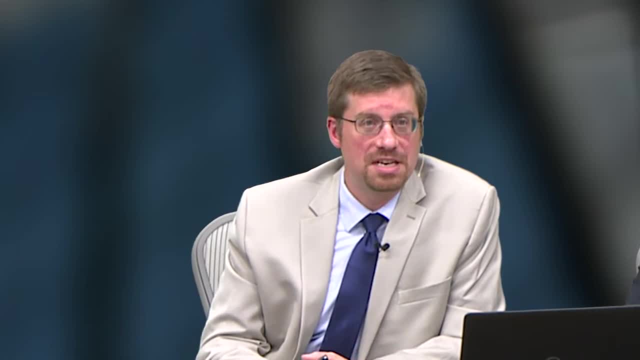 I'm not going to talk about it too much. we do have a group here at. I'm not going to talk about it too much. we do have a group here at. There's a third thing on that. I will tell you about it. so the first one. 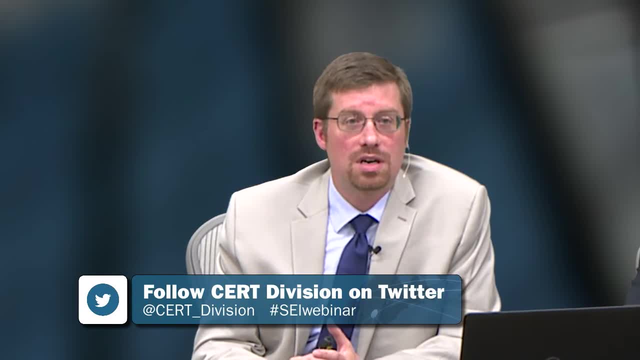 We usually it's award committee, for example. who is there and and what's your name? Lawyer, or til a, or creations Lawyer, Tennessee, fam, how you know, supporting Italian. nay, and it's a group of faculty at break. so two roommates who are comp showed up two fleet. 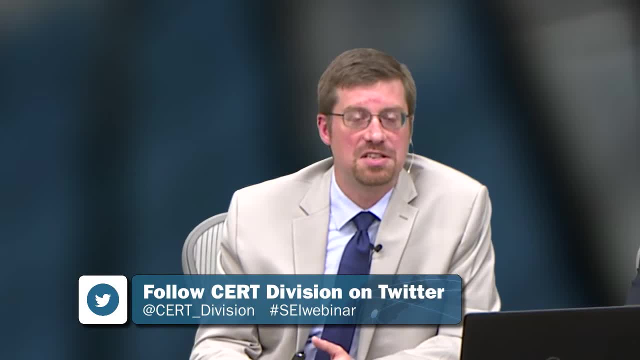 I'm sure they've met my assistant a few weeks back earlier today and they're both here. it was at the restaurant with a clienting contact education program. I'm sure they've met my assistant a few weeks back earlier today and they've both here. it was at the restaurant with a clienting contact education program. 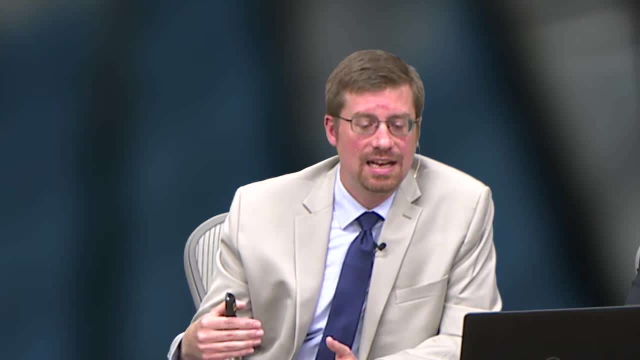 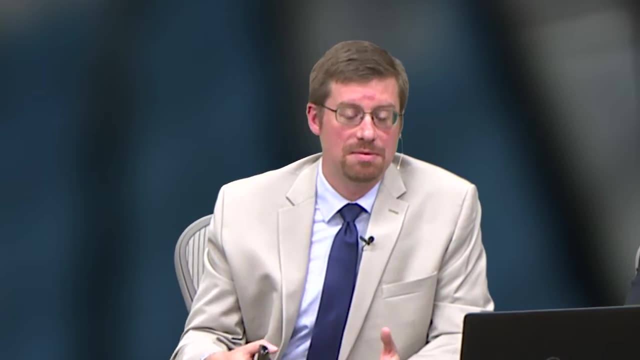 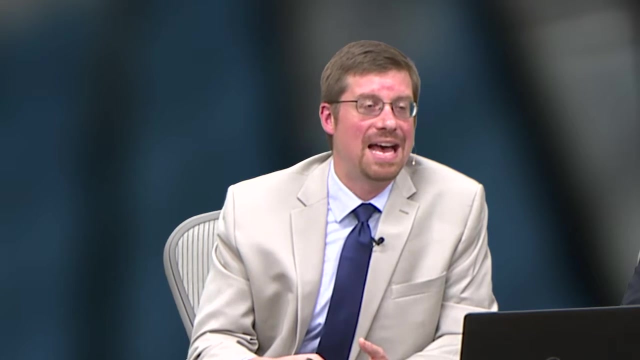 is concerting high school and has it's kind of like a lecture or apaid feedback s an on a life as a performer. wait a moment, They're was a fire. Actually, I'm just happy to done it. defects in the code. that may be part of a path. 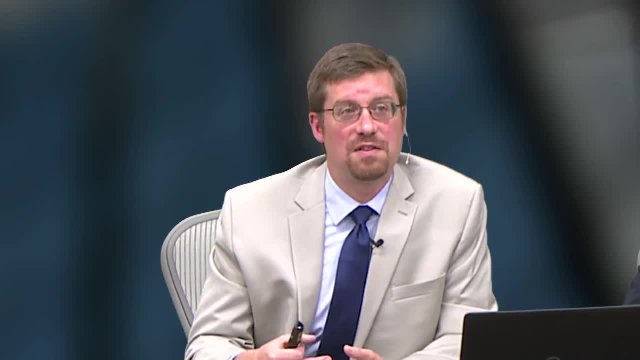 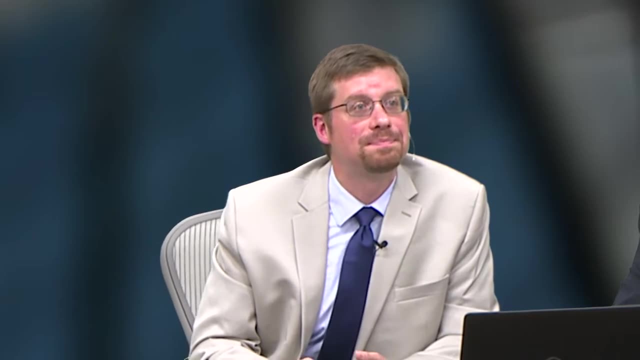 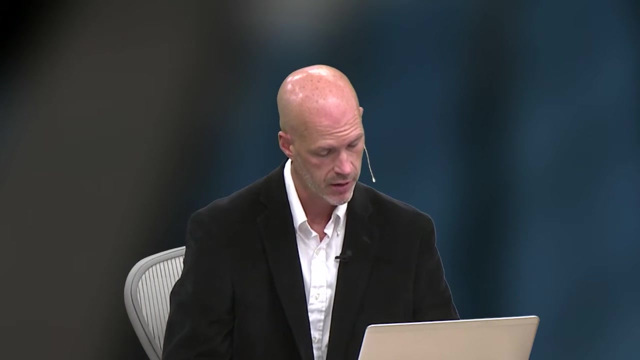 that isn't going to be taken. So it's really effective at finding vulnerabilities in code, so we definitely recommend using that as well. Just to close out this question, Bob: 52%. the question was: do you use multiple static analysis tools? 52%. no, we just. 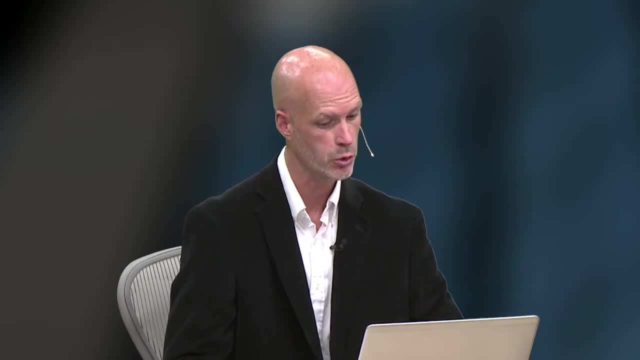 use one tool: 22%. we just don't use static analysis tools. 22% is yes, but we review the tool diagnostics separately, And 4%, yes, and we use a tool diagnostic aggregator. So I'm sorry, what were the first two? 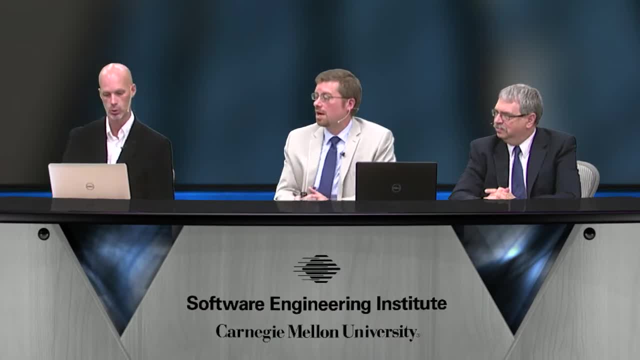 52% at. no, we use just one static tool, Just one, Okay. so more than half is using at least one, So that's really good. As I said you should, and several of the commenters on the chat have. 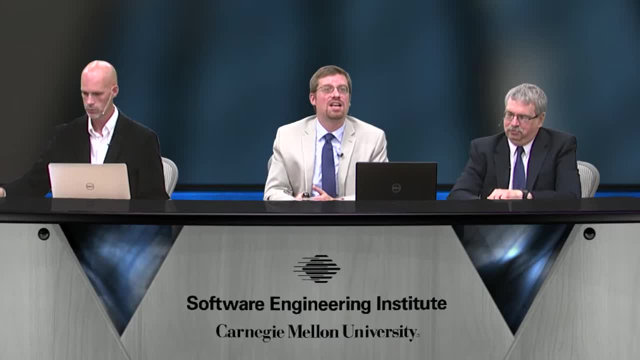 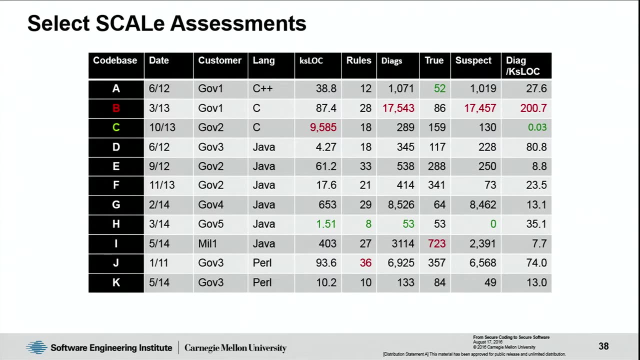 said, static analysis is a really effective way to find defects, And here I just want to speaking of that specifically. so here's some data of the audits that we have done across several projects, anonymized of course, but it shows that, on average, 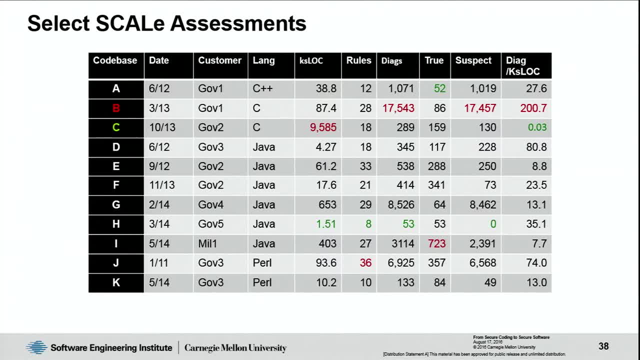 there's a large disparity across projects of the quality of the code But on average we've seen about 20 to 30 diagnostics that were true issues per KLOC or the S there is significantly remove white space and some other incommens and things like that. 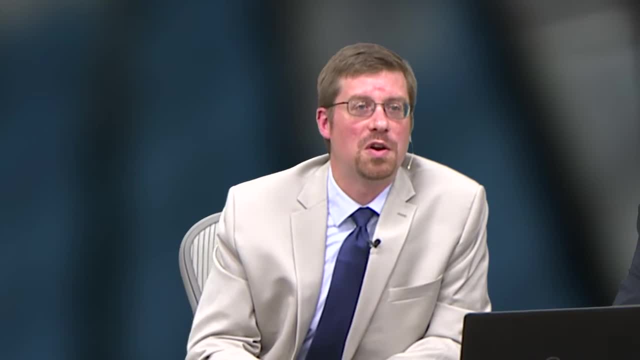 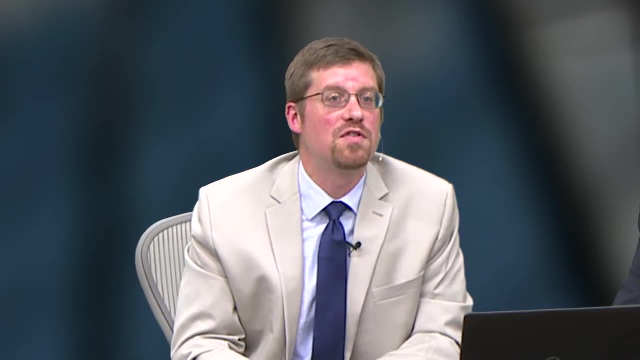 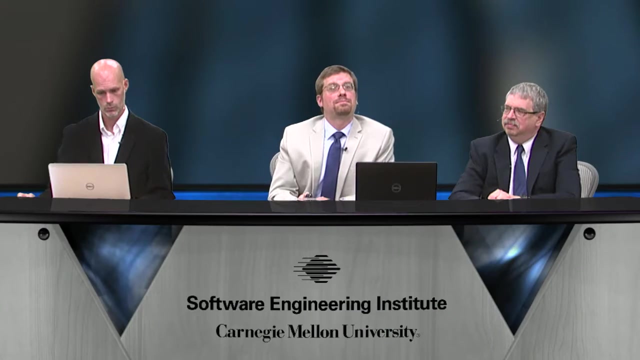 But the takeaway from this is that just about all code will benefit from static analysis, regardless of the process that you went through. If you've not done static analysis, you should, because you will find defects. And so here I'm. you know as we. so we've talked a little bit about the 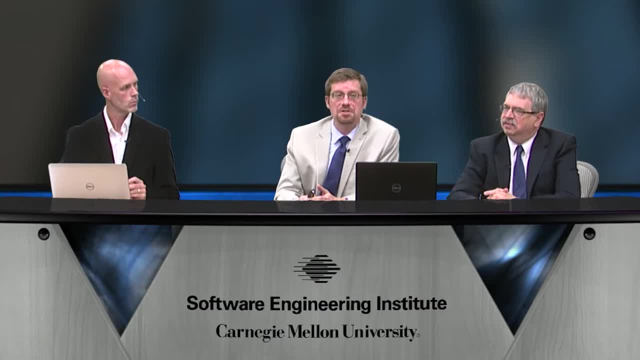 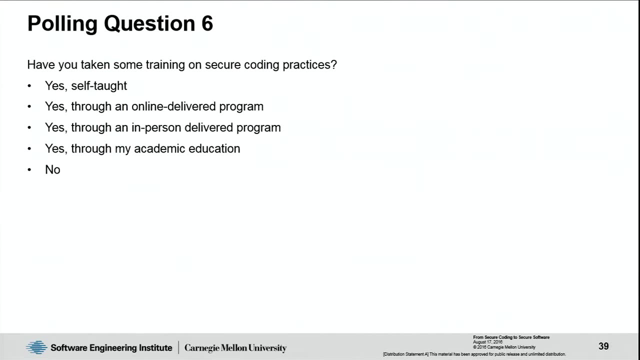 processes and adopting security, coding, standard and tools. I wanted to talk a little bit about training and development of the staff and the developers, But before I do that, I was hoping to see about this pool, this polling question: about what training? Yeah, so that question is one. 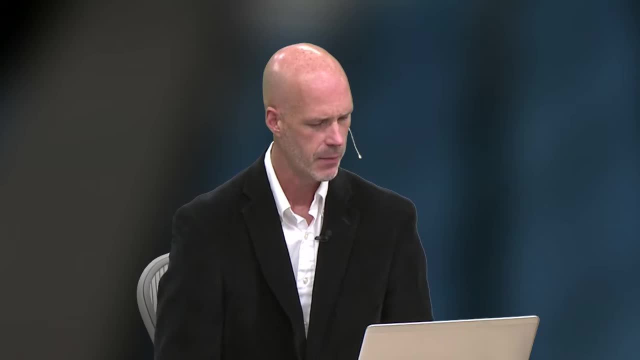 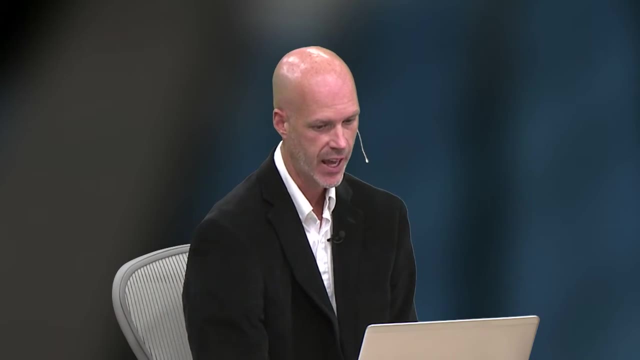 So maybe we can work on one question from one: Why this is launched, Bob Sure, And maybe you covered this or not, but I'll just ask it, Sure sure, It came in earlier- How effective is static code scanning- ie Fortify- to detect bad security practices? 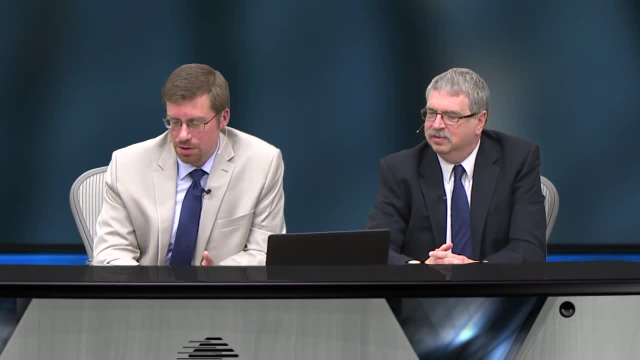 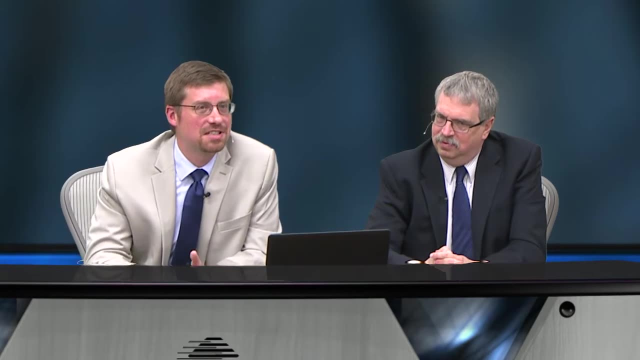 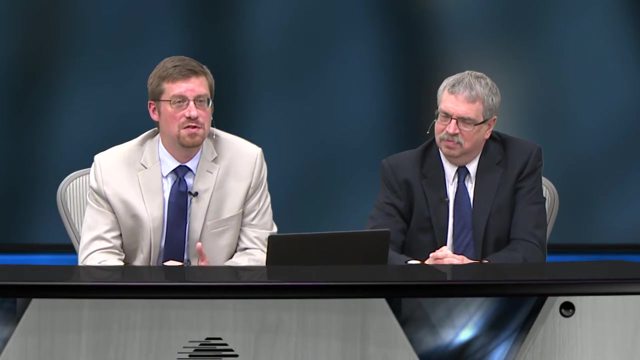 How effective is static code scanning? ie, Sure, sure. So that's the static analysis that I've said. So I've not given quantitative metrics other than showing that it's that it is very effective in finding issues. Again, if you've not done static analysis, 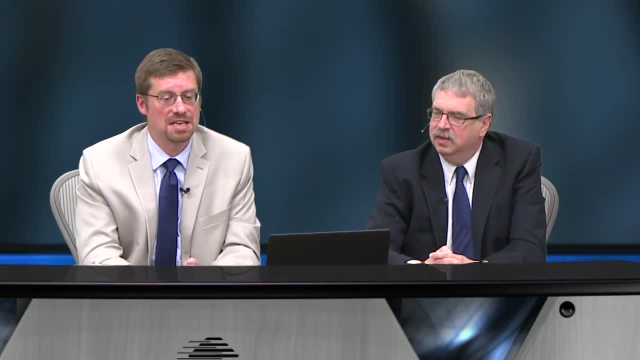 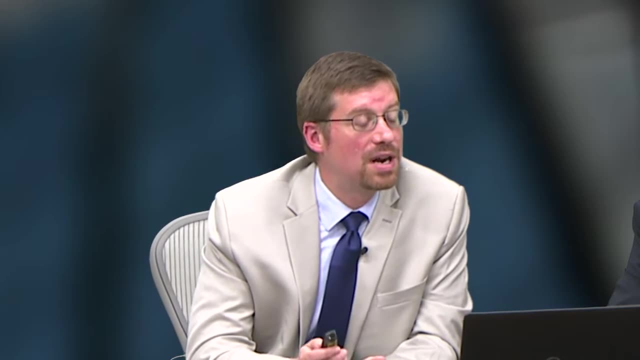 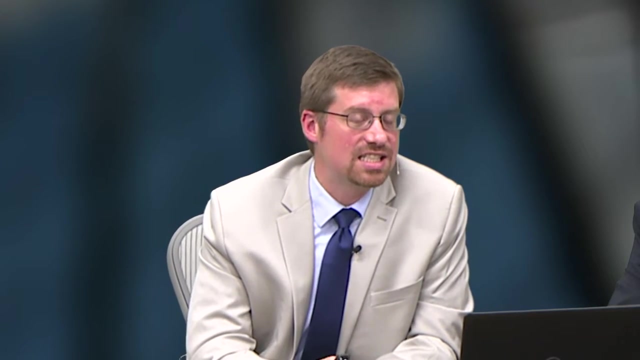 You will almost definitely find issues by doing it. HP Fortify is one of the top products out there. And what I didn't make clear about scale- I think I might have implied it but didn't make it clear- Scale itself is not a static analysis tool. 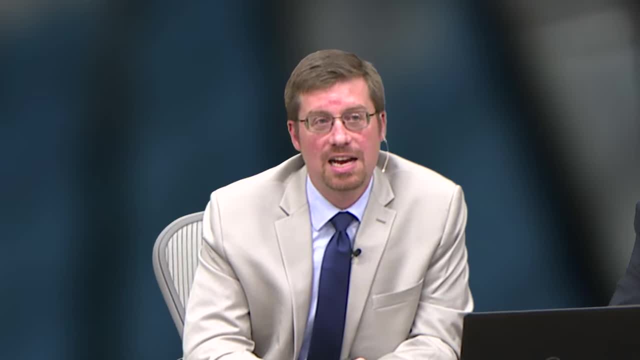 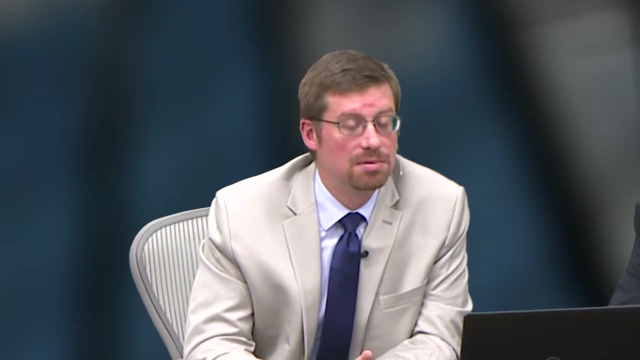 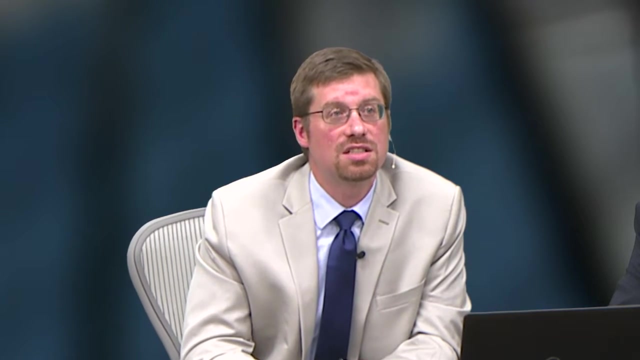 It is only an aggregator. So those boxes in the diagram about static analysis tools, we're using a lot of the same tools that are available, Some that are available to the public, like Fortify and some others, And then we're reviewing those diagnostics. 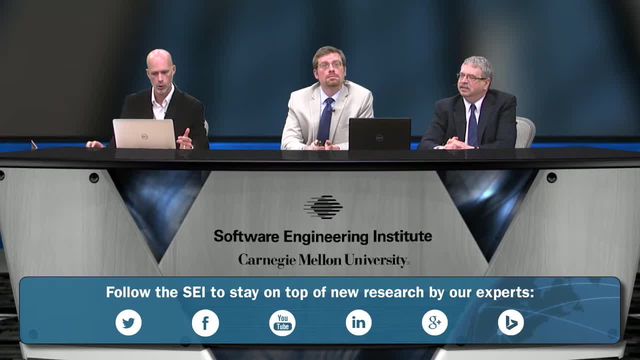 So it is very effective. Okay, We'll just wrap up this polling question here. Sure, And one other question. The question real quick was multiple people asking if an archive or recording is available from the talk. An archive of the whole seminar will be available by tomorrow. 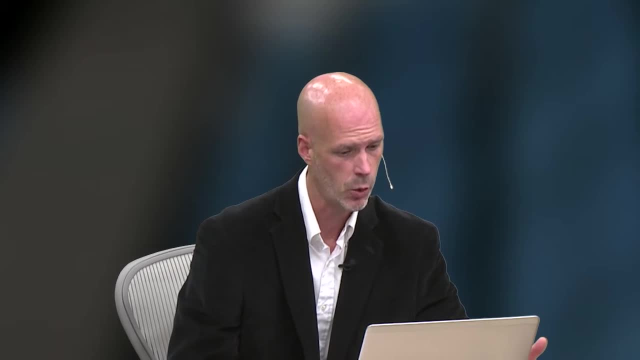 Same registration URL that you used today that you can watch the archive. So the question was: have you taken some training on secure coding? 31% yes, self-taught- 12% yes, through an online delivered program: 14% yes, through an in-person delivered program. 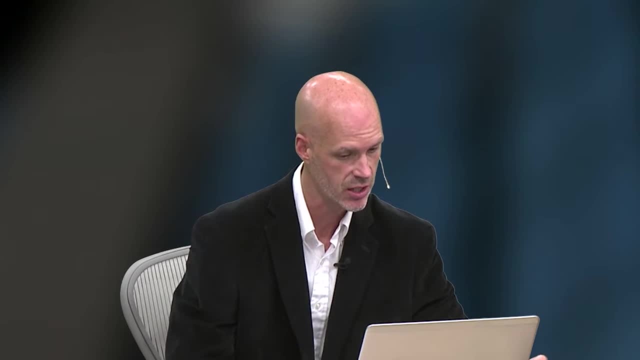 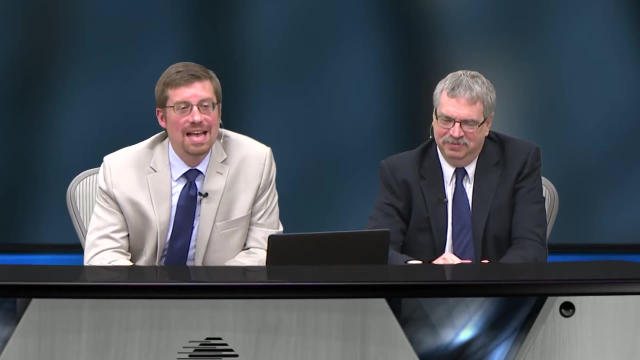 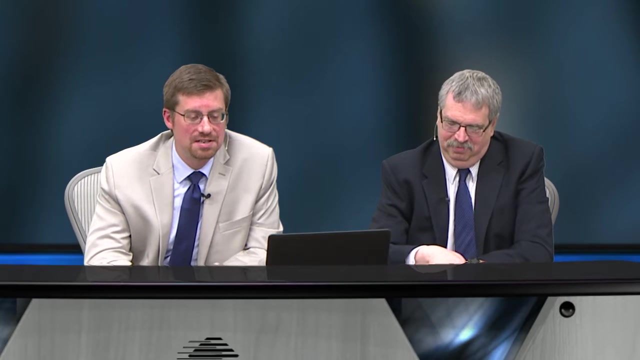 Five yes, through an academic education And 38% no. Okay, Okay, Great, And thanks for everyone for being honest. So it's actually a little better than I thought. I like to say generically that in today's world, because it's so easy to program that 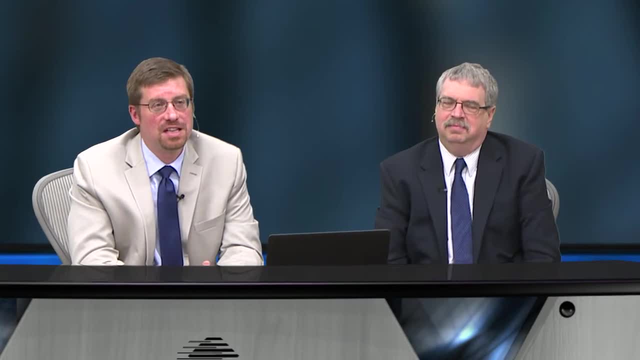 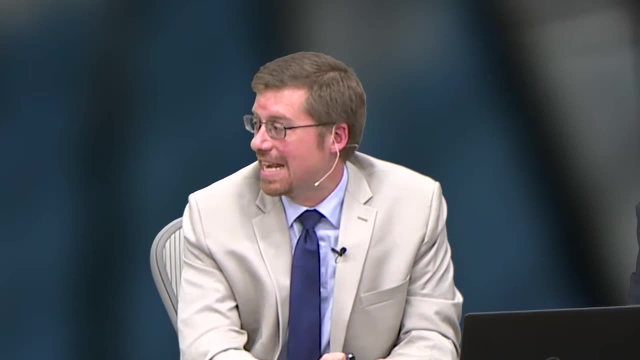 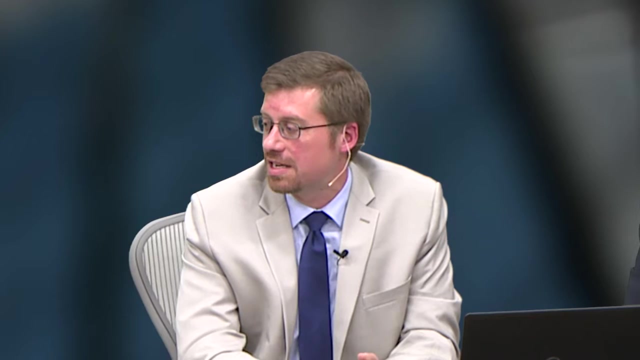 a lot, if not a majority, of developers. people that are software developers have not been properly trained in software development, And almost none of them have gone through secure coding training, So it's actually even the self-taught people I think are better off. 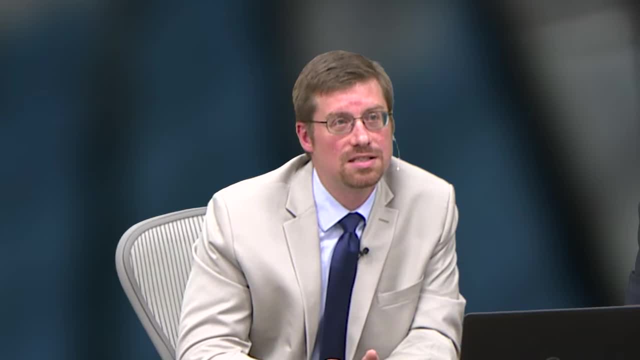 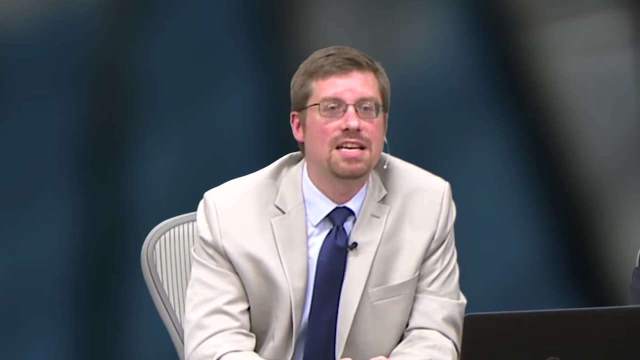 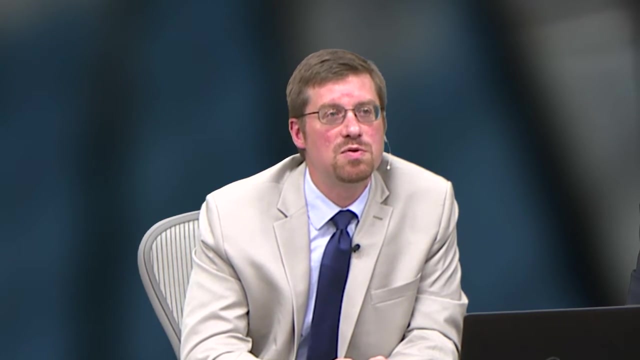 It shows that you have an interest in learning about secure coding practices And it's a lot more effective than not having any. So for the, I think it was 38%, 38%, that was no. I would definitely recommend at least trying something online as a MOOC or something else. 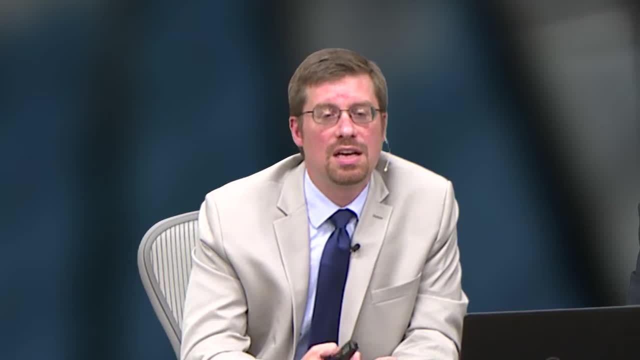 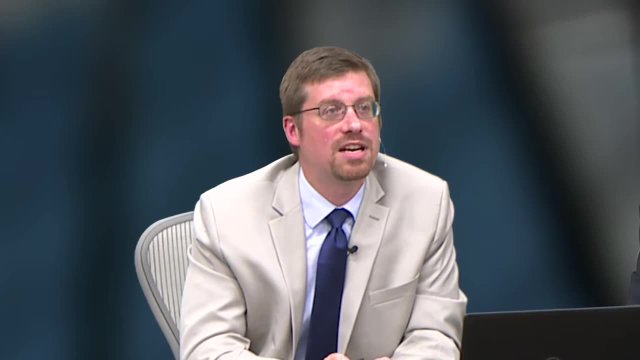 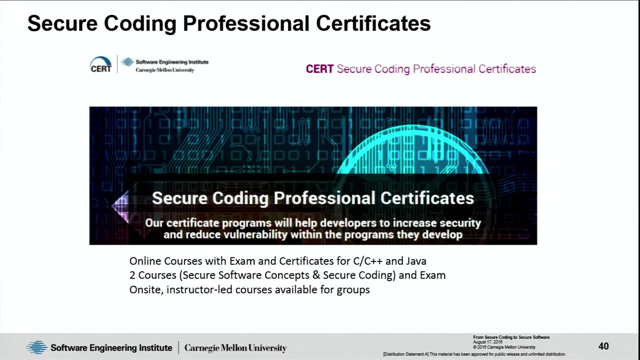 And if you have a large group, we have instructor-led training. We also, if you want something more formal- and I'll talk about this in a minute- but we have online training as well, And so, to kind of roll into that, as I was mentioning there, we do have online training. 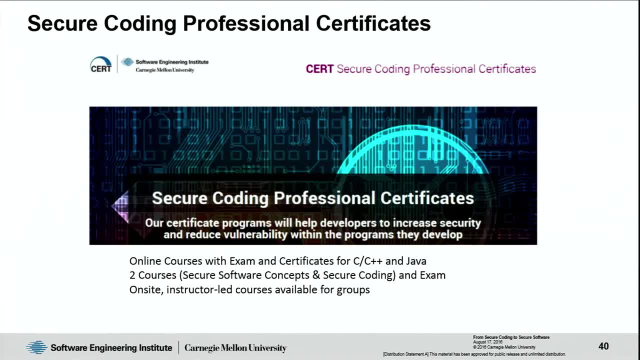 that ends with a secure coding professional certificate And this training is in the C C++. So one edition of the training is C and C++ combined And the other is Java. And each of those certificate programs have two courses: a software, a secure software. 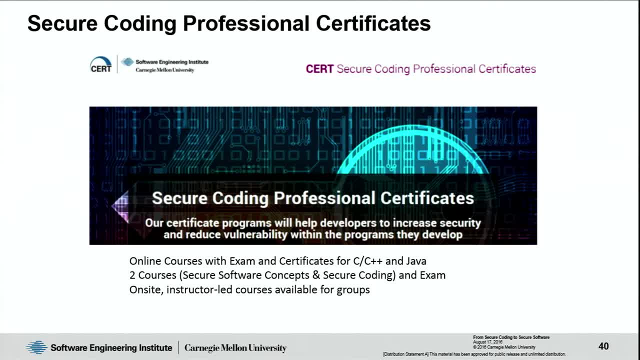 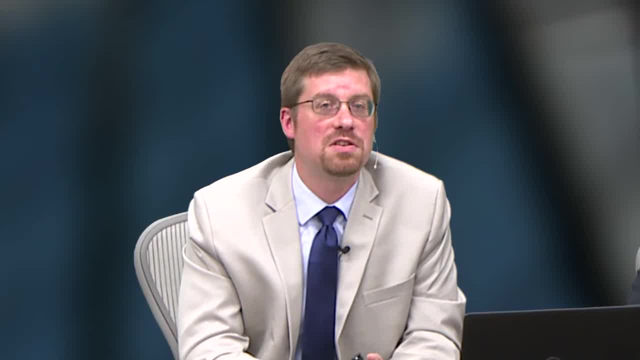 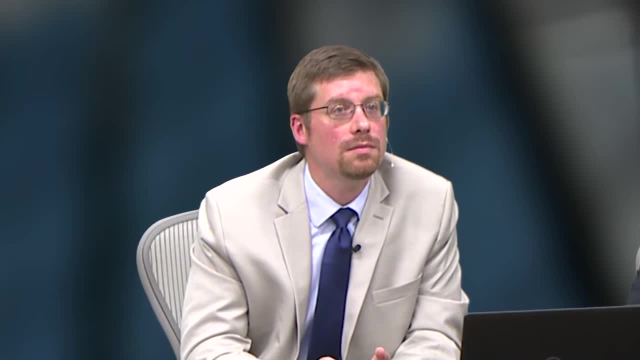 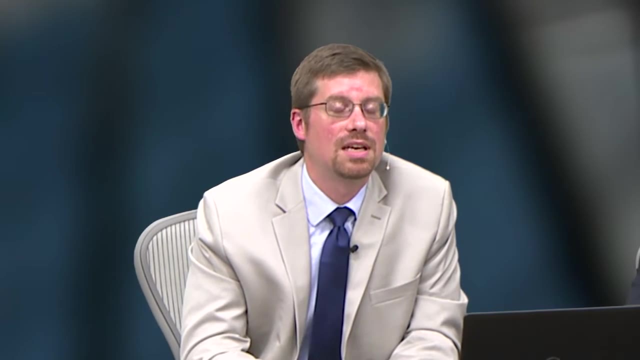 concepts course and then a secure coding in the particular language course And then it ends with a completion exam. And then we also, as I mentioned for larger groups at an organization, we have instructor-led courses on site as well. Here I'll talk just for a minute about the some of the topics and the objectives of the. 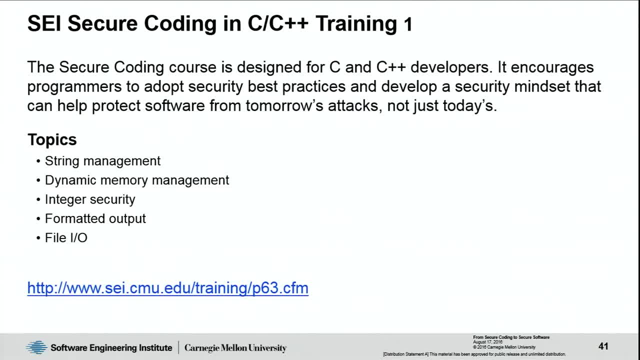 course And these are really topics and objectives that you'd look for any course that you were going to take in training. These are kind of the common issues. So secure coding in C++ Obviously really important for string management: String meaning, array meaning buffers and buffer overflows. 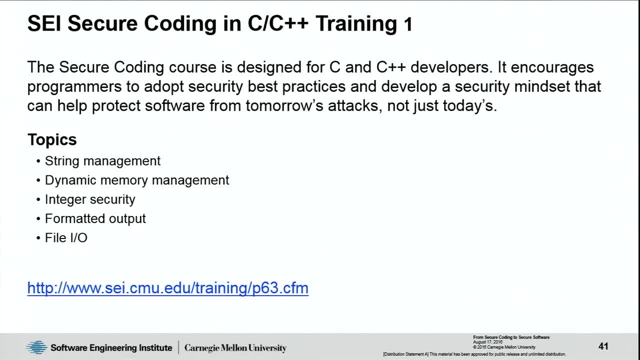 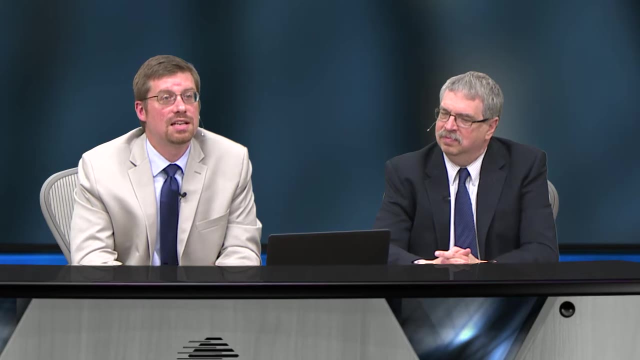 Dynamic memory management is another big issue, And pointers and freeing properly memory. You have integer security, as Mark was mentioning, wrapping of integers and that, especially if it's in pointer, arithmetic That being an issue- And formatted output, that being format strings and then file. I O 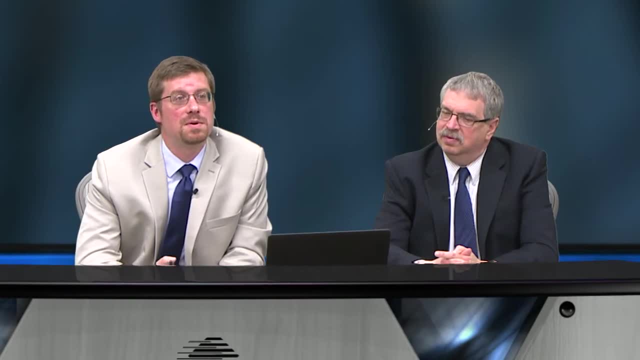 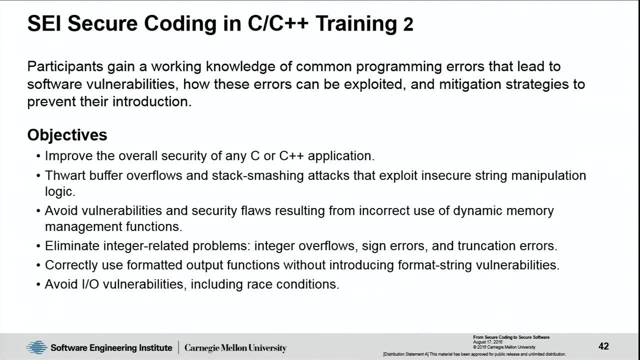 And the objectives are, you know, to improve the overall security of the C and C++ applications that you're developing, Avoiding vulnerabilities by learning what again the constructs in C and C++ are that you shouldn't use or how to use them appropriately. 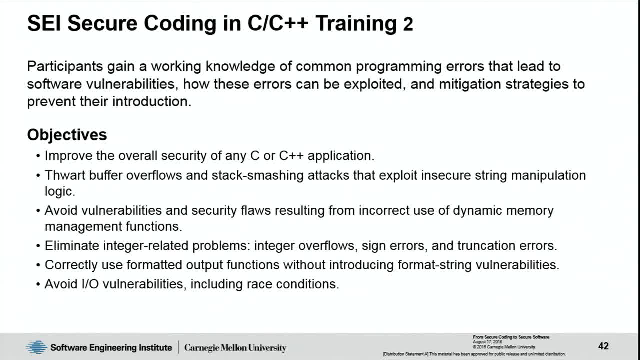 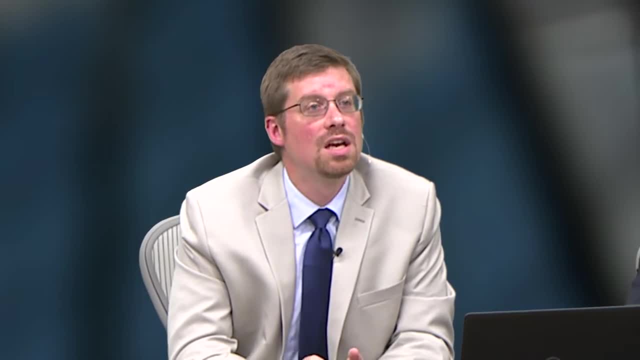 Because often just calling a particular method or function is not the right way to do it, That there's other checks that you need to put before or after you call functions to protect the software, And this teaches you how to do that. And then the Java secure coding course, as I mentioned. 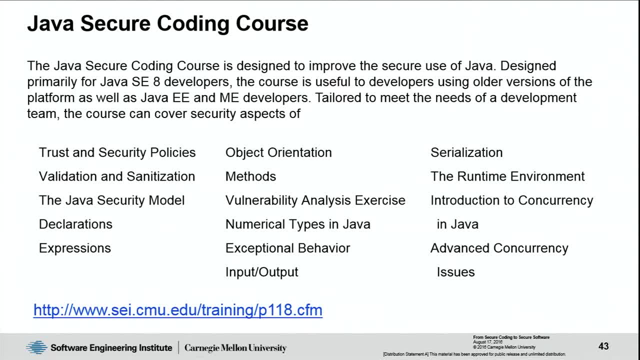 So a lot of people immediately think: well, Java's secure as is. It has memory protection. It has a lot of other protections. Well, as it turns out, there's a lot of different ways that you can misuse Java. Not the same ways as C and C++, but you can get into trouble. 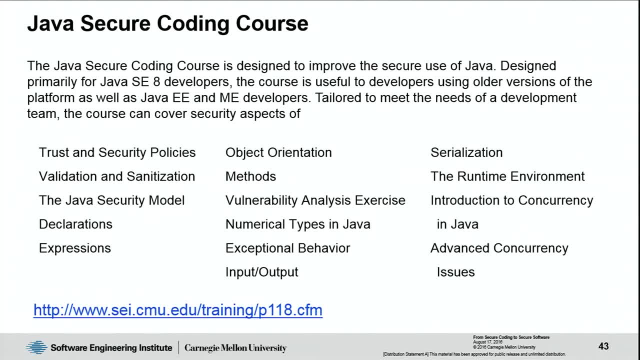 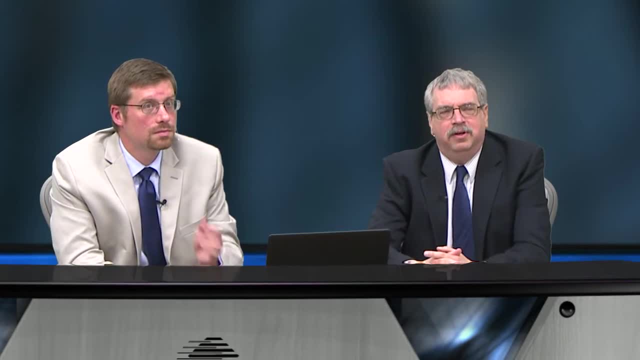 I'll just mention the one in the top right there. Serialization and deserialization has been a very recently come out as a trouble spot with Java and using it correctly, And so there definitely are issues there. Go ahead, Mark. And just to illustrate the comments that people were making before with SQL injection: 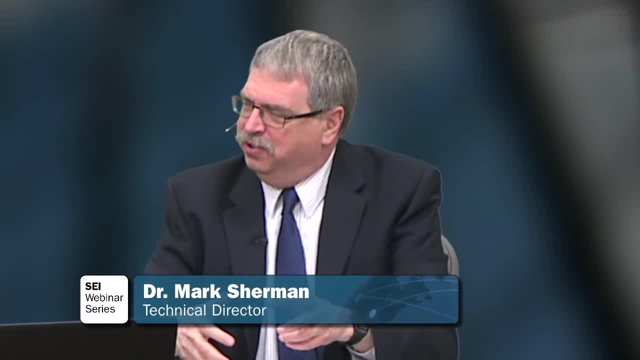 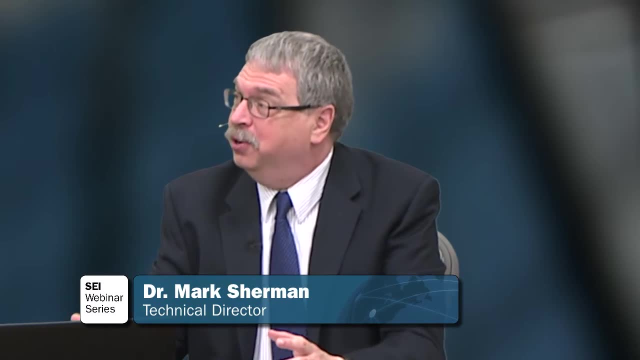 even within Java, you have the same issue, that vulnerability, whenever you open up the capability to execute arbitrary code. In the case of Java, they call it class loaders, But nevertheless it's the same paradigm that we see repeated in languages again and again. 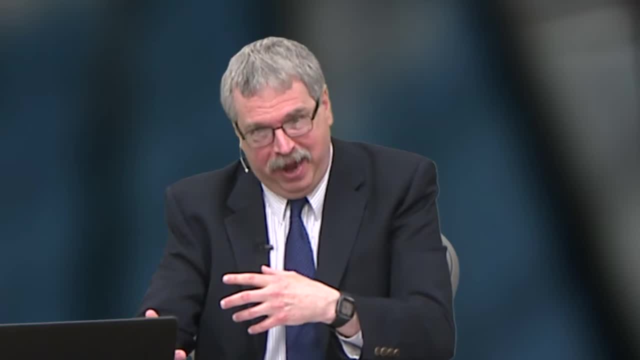 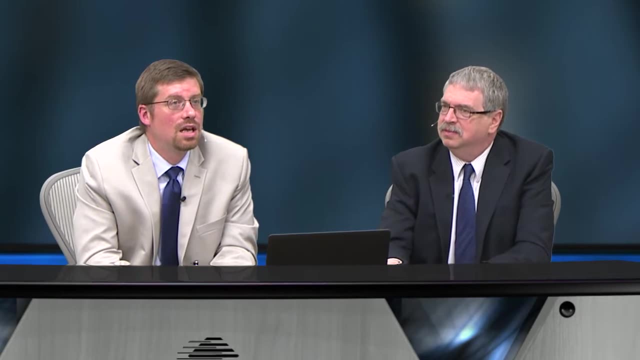 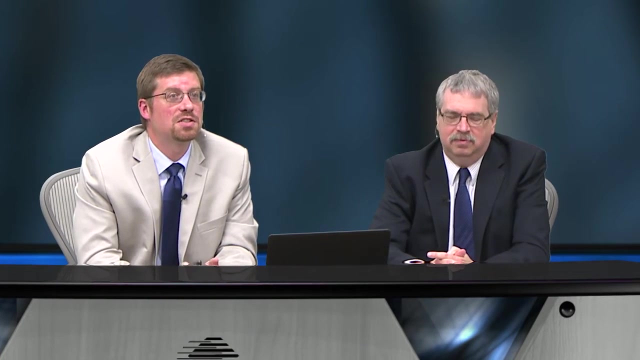 And how you protect against it has the same generic answer: The details depend on the language. Yeah, that's right. Interfacing, using Java to interface with other languages and using the constructs of Java correctly are not always obvious, And so this teaches you how to use those APIs correctly in a secure way. 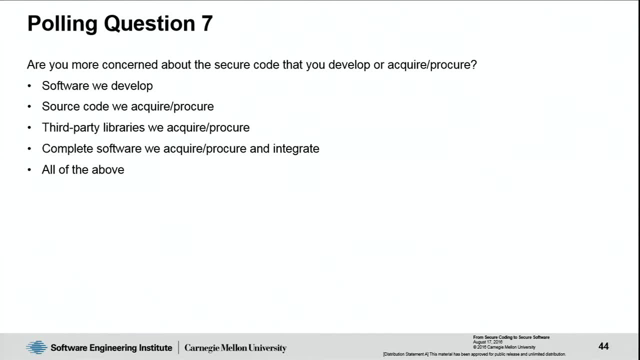 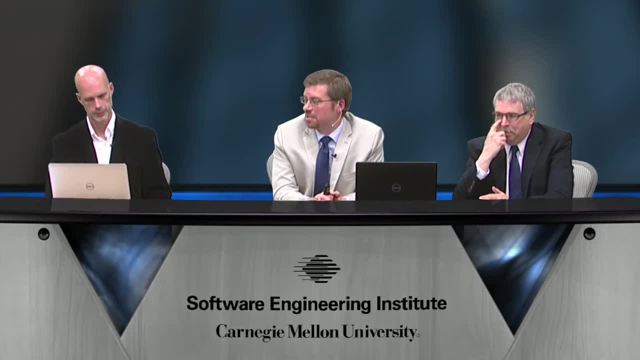 And so that covers most of what I'm going to talk about of developing software. Of course, that doesn't address everybody's concern. Well, nothing does. There's a big area that it doesn't address, And that is that a lot of people acquire software or acquire source code or libraries that have been compiled. 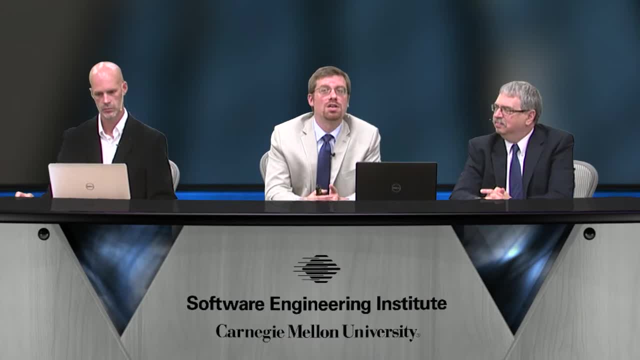 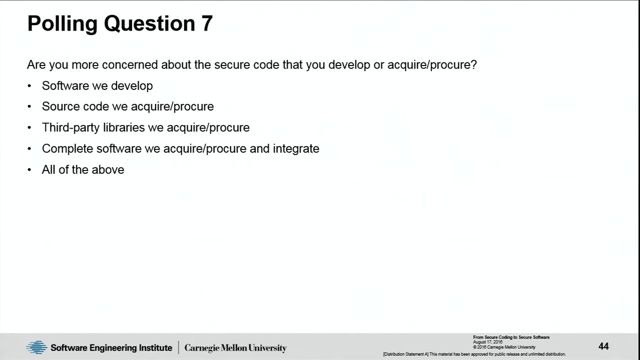 And they're using third-party software, but they're not sure what's in it. And so first I'd like to find out from this polling question what people's proportion of building versus buying, so to speak, even though I know that often it's open source and free. 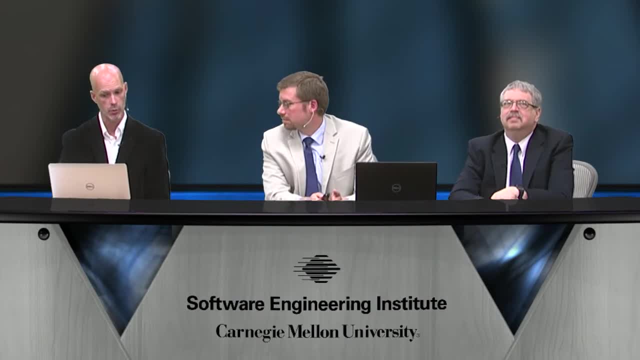 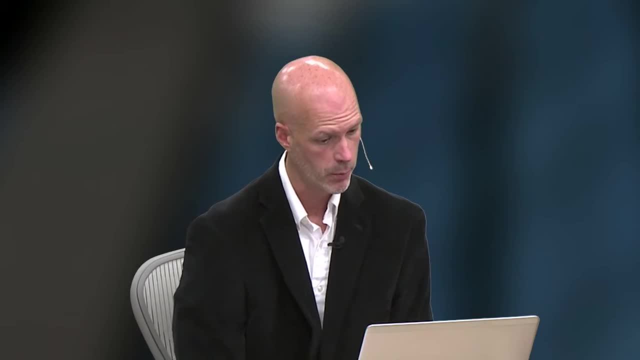 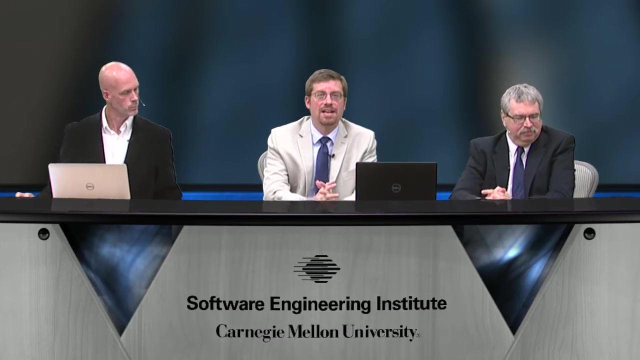 So we've got 34% software. we develop, 3% source code. we acquire procure 10% third-party libraries, 1% complete software. we acquire 52%. all of the above, Okay, So a lot integrating pieces and packages from a lot of different places. 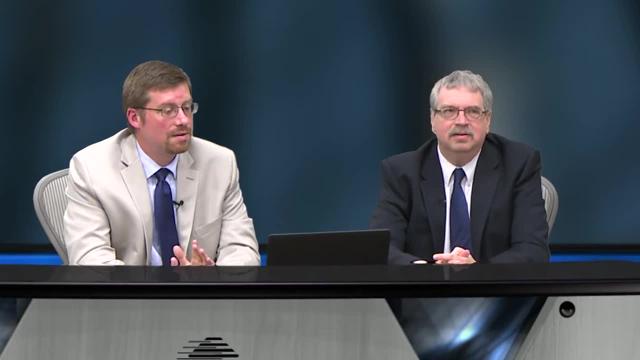 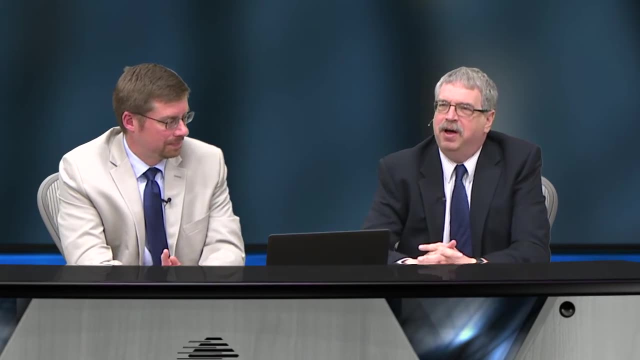 So I was wondering, Mark, could you talk a little bit about acquiring software securely? Sure, And also we'd like to just react to a couple other questions. There was a fair amount of discussion about scale, about the aggregate that we talked about. 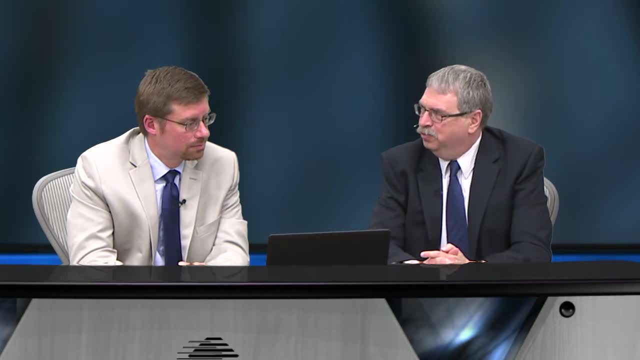 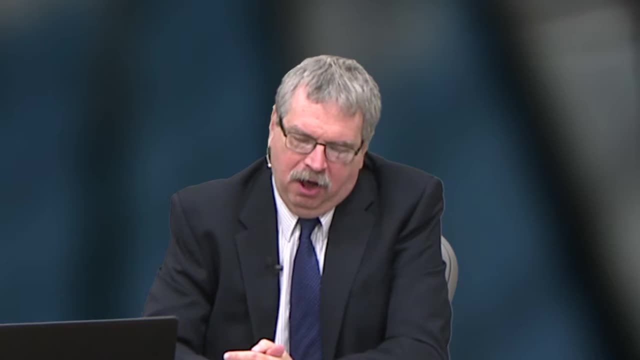 And clearly we've been asked to include information about where to find that in reports and so on, So we'll include that in the website rather than trying to give all those URLs on the fly here. There was also discussion about compiler optimizations and someone used the word undesired. 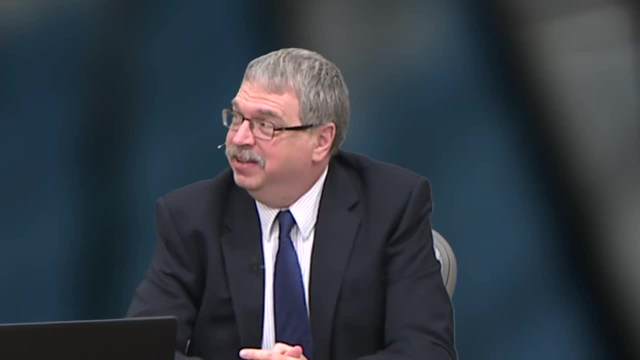 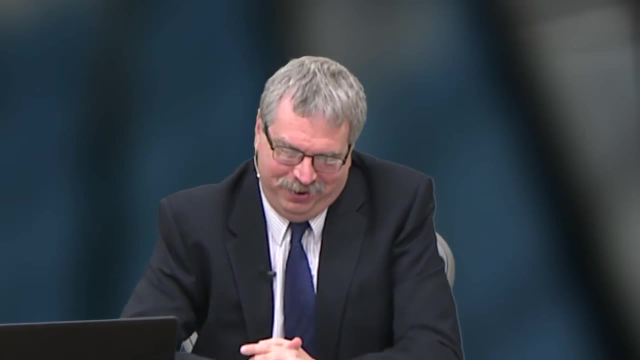 Our technical team actually is really fascinated by that particular topic and they've put together a whole other presentation and seminar which, if we want, by all means let Shay know. But we call it unexpected compiler optimizations because all those optimizations were put there for a reason. 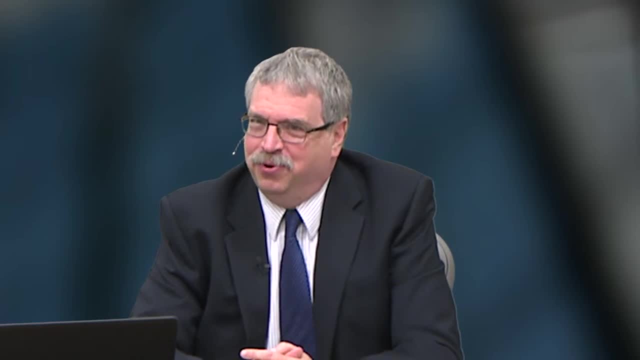 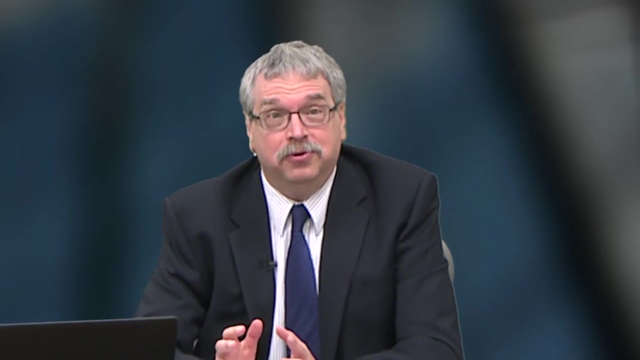 So certainly in many circumstances they were desired. The question is whether you would expect them or not, And the broad-brush comment we'd make is either. one set of problems happens when people really don't understand the language in enough precision. The other circumstance where it runs into problems is in portability. 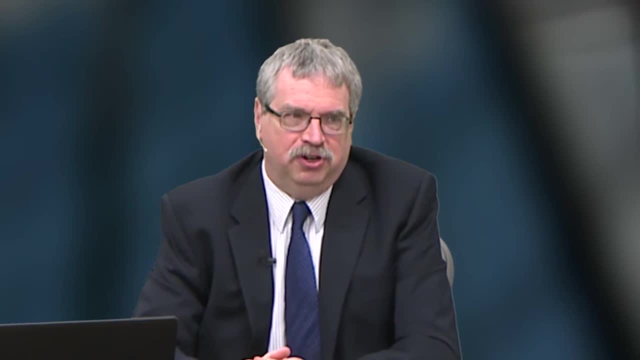 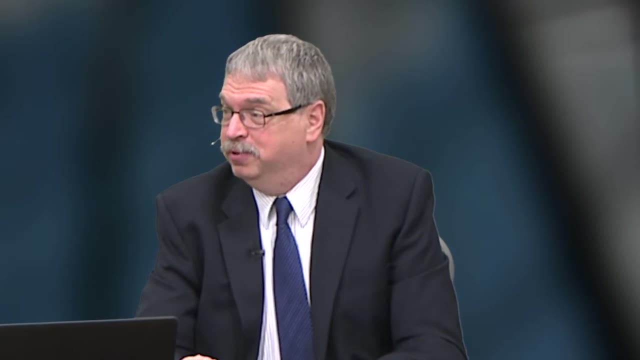 in, where they do understand the language in the correct precision, but they move it from one system to another system, And a common one that we've seen is moving from 16-bit to 32-bit machines and all of a sudden, optimizations which they thought, assumptions and implementations, they thought. 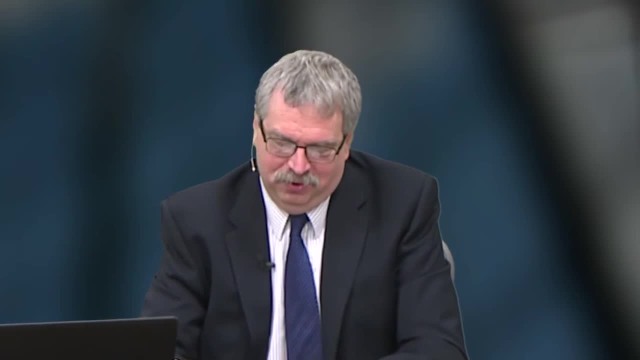 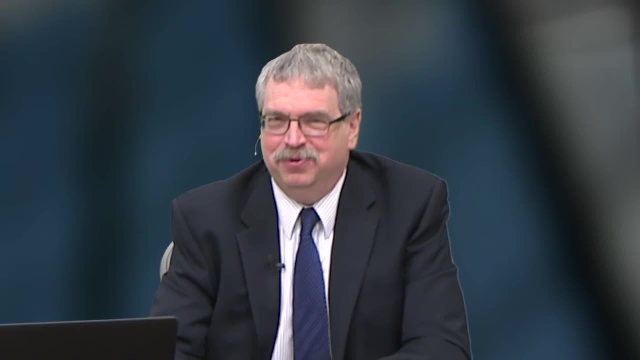 no longer hold and they run into problems. But that's a whole other talk And there's a whole lot more to be said there. We'll defer that to another time if you'd like to hear about it. But one of the topics that we've run into when we talk. 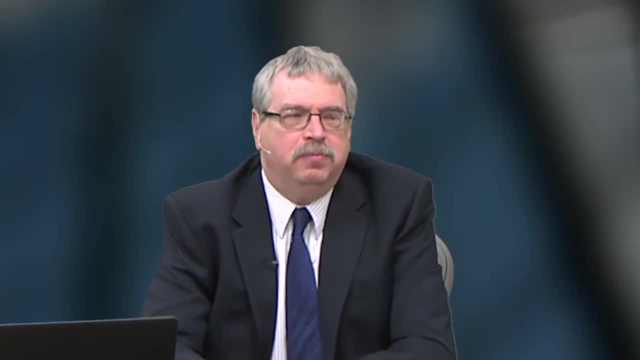 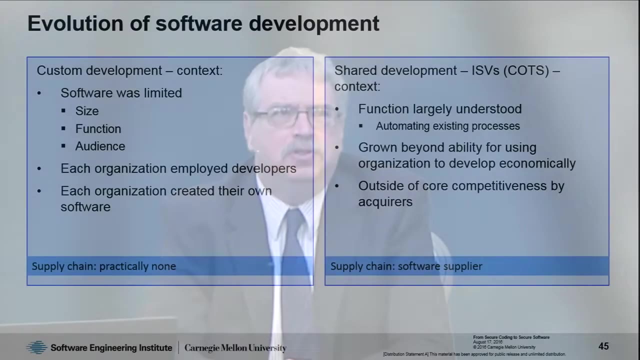 when we talk with development organizations about the problems that they face, part of it is what we discussed here is the code that they are writing, And historically that really was the focus of attention. So when software started being developed- and I'll use my own sister as an example- 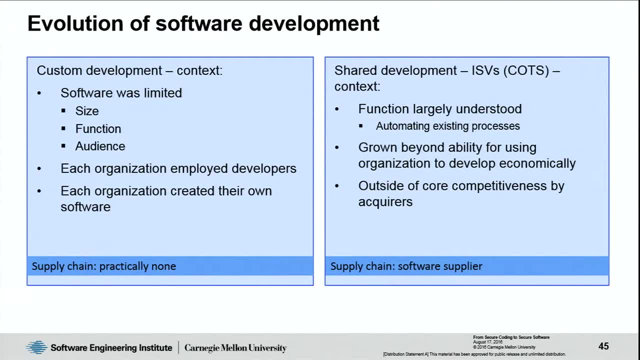 she worked for a large manufacturing company and one of the jobs she had to do was to build an airline reservation system. No, she didn't work for Delta or Unite or whatever. She worked for a company that you know had plants and extrusion lines and so on. 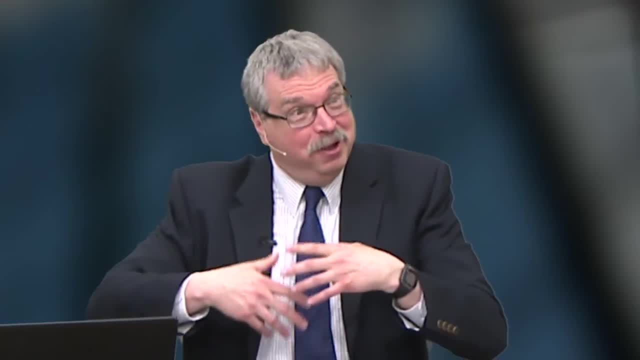 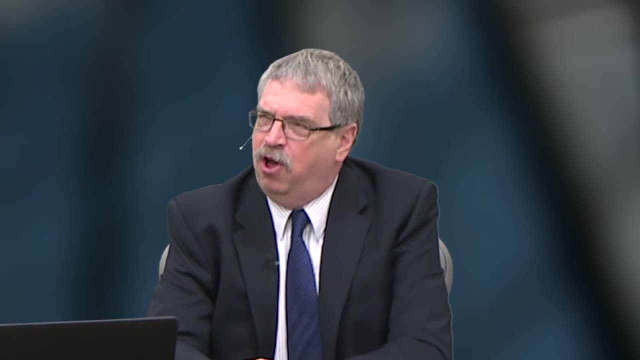 But they had a bunch of corporate jets and they needed to schedule them and so she went and built an airline reservation system from scratch. In that kind of context it was custom development, limited amount of software, limited audience, limited function. And for those purposes, companies like that one basically employed their own developers and they created their own software. They developed everything That turned about to be fairly expensive and quickly. they decided that there were some things which really weren't their core differentiation. 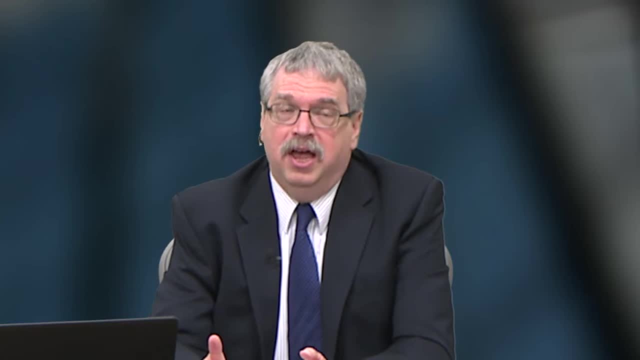 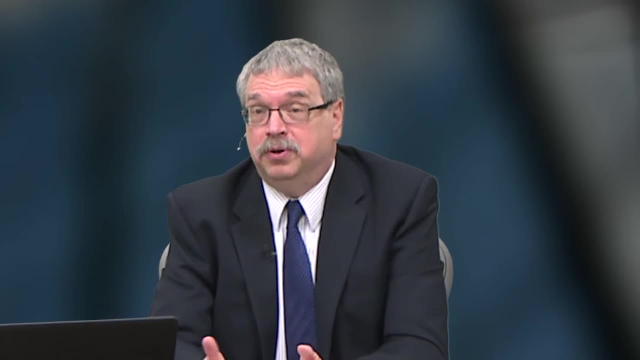 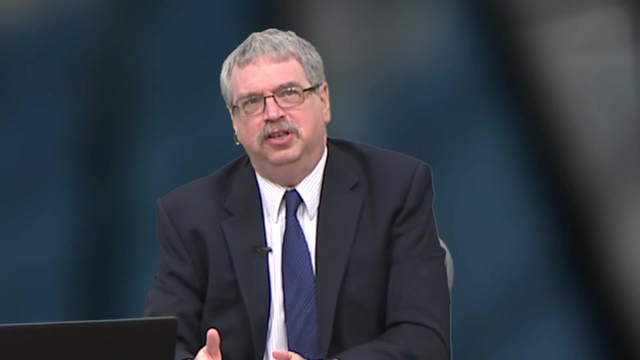 And so the industry of independent software vendors came up and they were automating well-known processes. I don't know about airline reservations being so ubiquitous, but things like general ledger were enterprise resource management, supply chain management, the whole variety of common kinds of functions that needed to be done. 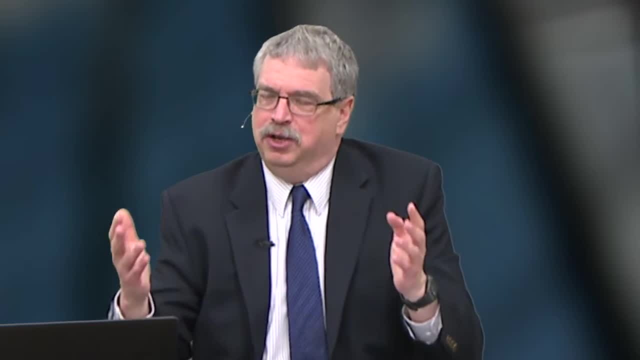 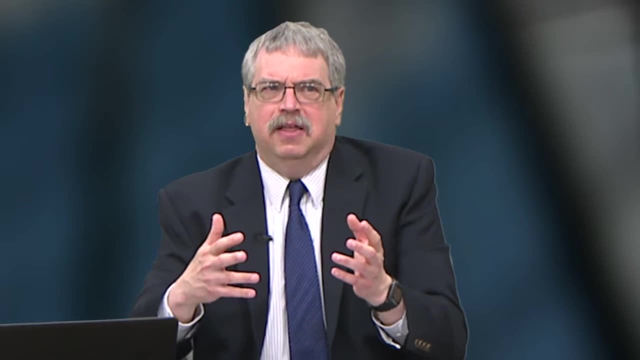 that were not the specialty of any one company, And so you had InforGlobal, SAP, Oracle, a whole variety of infrastructure companies who went and built this, and now you started getting a supply chain, A very small supply chain. It was just the vendor that you dealt with. 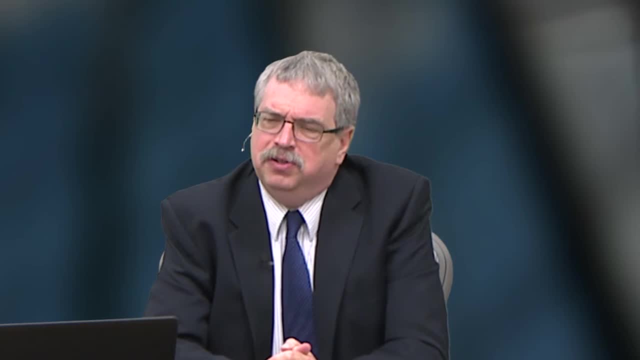 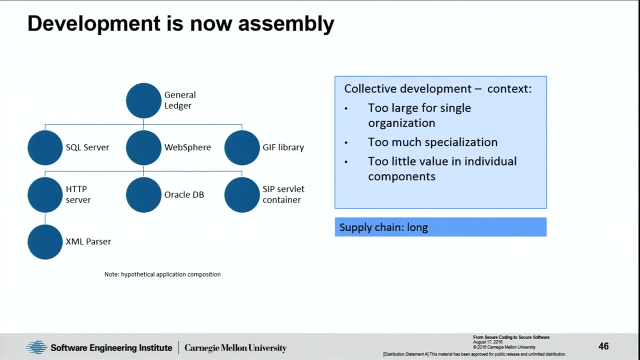 What has evolved over time is that actually there's very little development being done on large programs outside of these independent software vendors. I mean obviously Oracle or Microsoft spend a great deal of their time building programs completely from scratch, But for most places development is assembly. 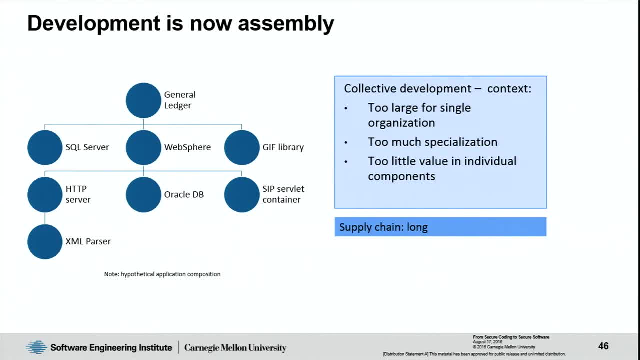 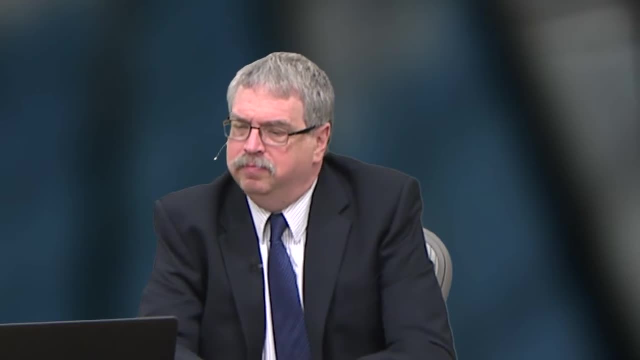 It's simply too large for any individual organization. There's too much specialization in each individual component And, frankly, every little component doesn't have enough value to invest in it, whether it's a SIP container to connect to telephony systems, your own database, your own XML parser, and so on. 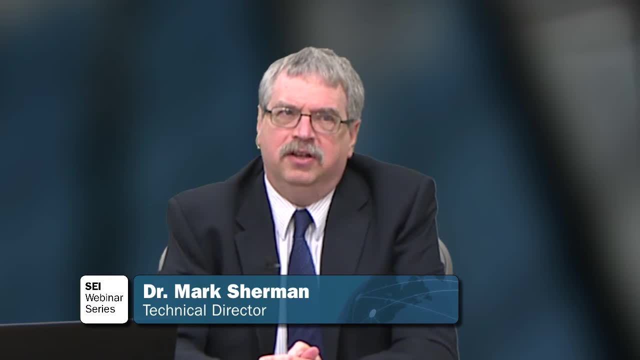 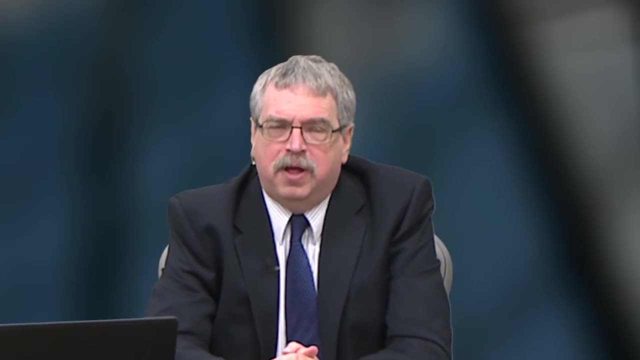 So instead, what we've wound up is having a large supply chain in where you reach out to lots of vendors and they reach out to vendors and they reach out to vendors, But in this supply chain you have a large amount of open source. 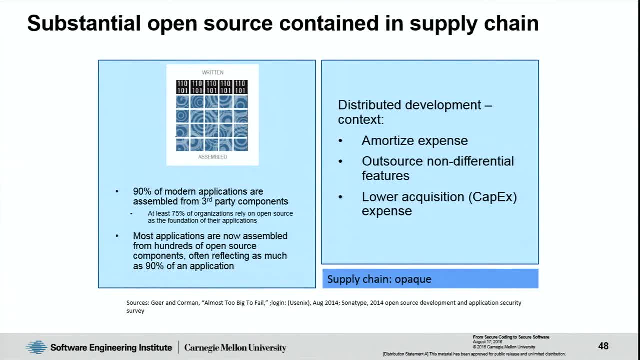 So what's the magnitude of this? Well, when we've done, we rely on third-party surveys. they found that about 90% of applications, in fact, are assembled. They're not constructed. And perhaps as importantly, of those assembled applications, 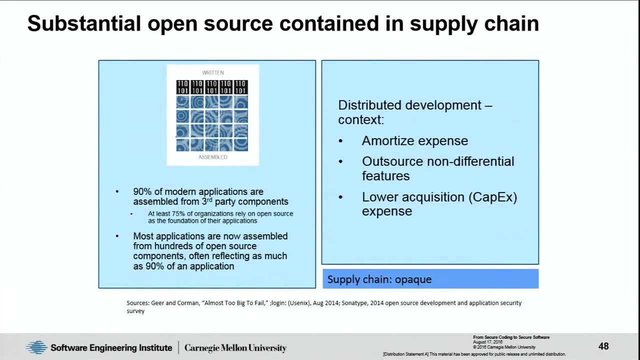 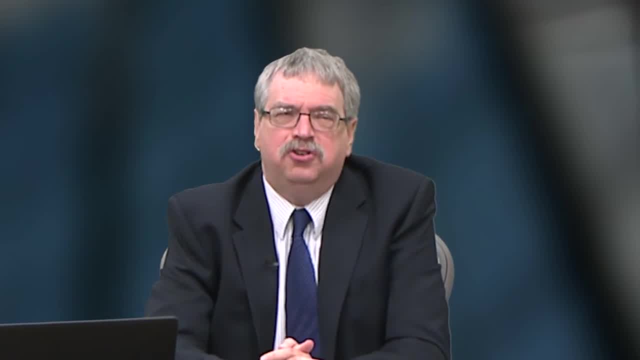 90% of their content comes from the outside, And so now you have a very long supply chain of people getting pieces from other people. It's very long. Just to give you an example, let's say you have an application server that contains an HTTP server that came from another place. 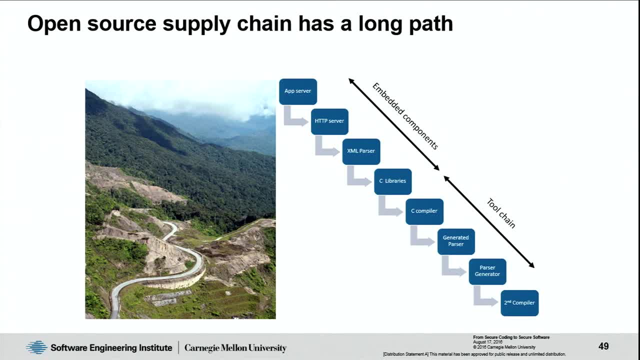 which has an XML parser which came from another place, which came with some C libraries that came from another place, That was generated by a compiler that came from another place, The compiler itself was generated by a parser generator that came from another place, and so on. 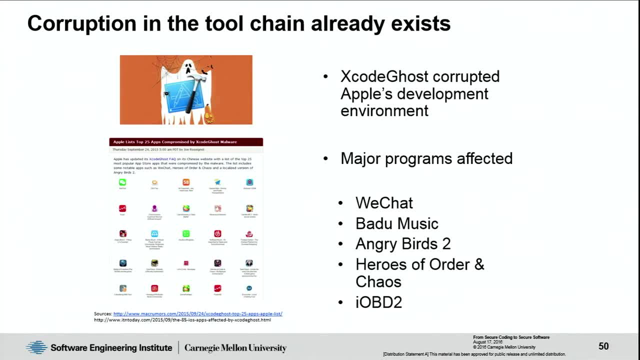 You wind up that there's a huge, long list of dependencies And there are problems. You might think that who's going to really screw around with the compiler? Well, it's happened already. For example, Apple had their development environment attacked. and, as a result, they had applications built with Xcode of being corrupted And open source is not secure. We use a lot of it. People know about shell shock and bash bug just as two common examples. That happened because people were explicitly exploiting them. 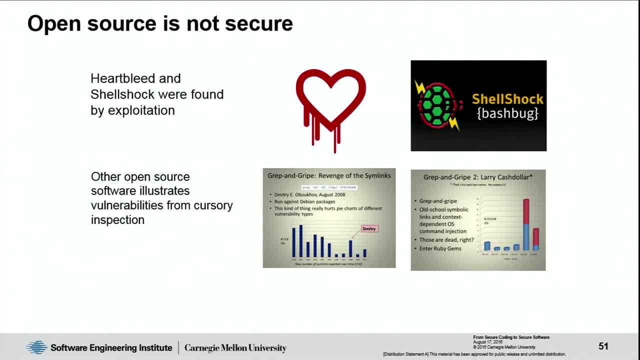 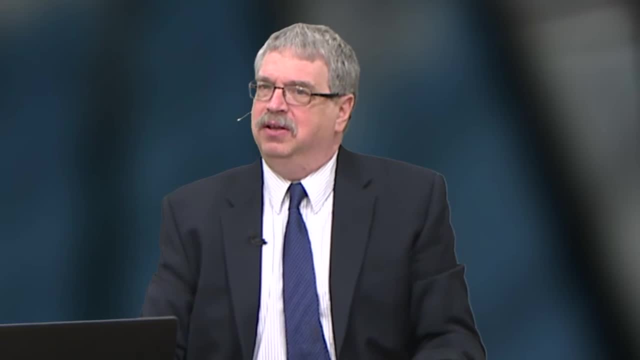 But worse. a study that was presented at Black Hat showed that finding bugs was basically just shooting fish in a barrel, And they were quoting some researchers here which said: we just decided to go look for a particular kind of bug and they found so many that it was upsetting. 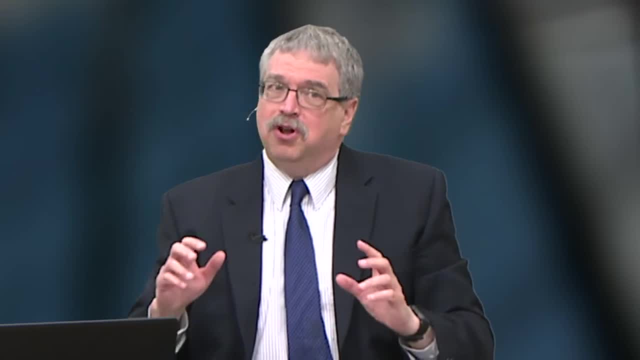 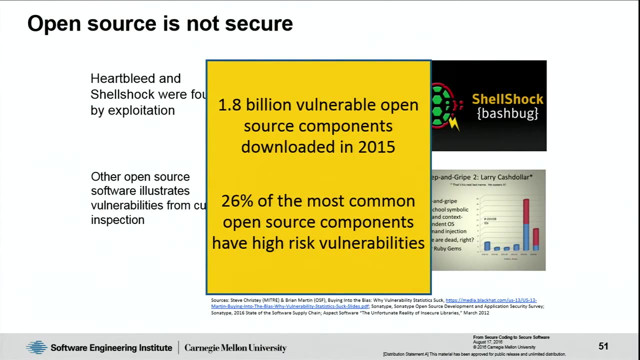 all the statistics that are being used Now to quantify this, rather than just say, well, there's shell shock and whatever. again, there have been studies done. Just in 2015,, close to 2 billion open source components with serious vulnerabilities were downloaded. 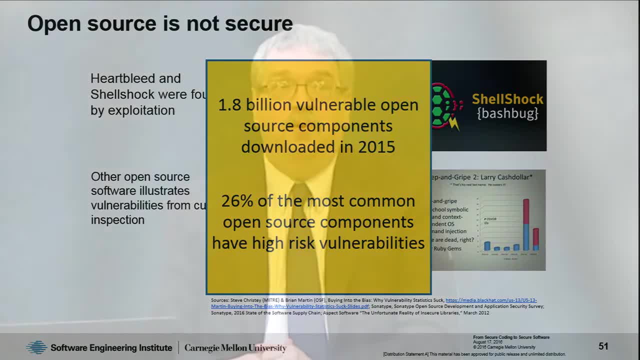 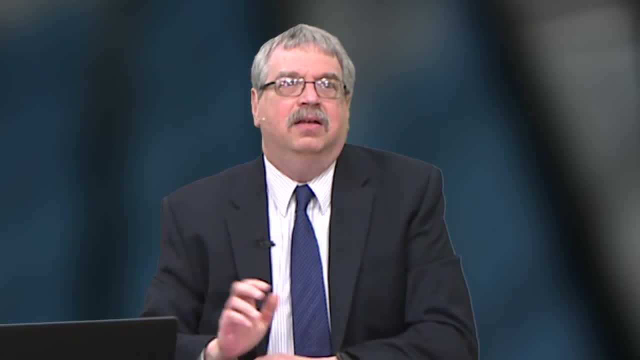 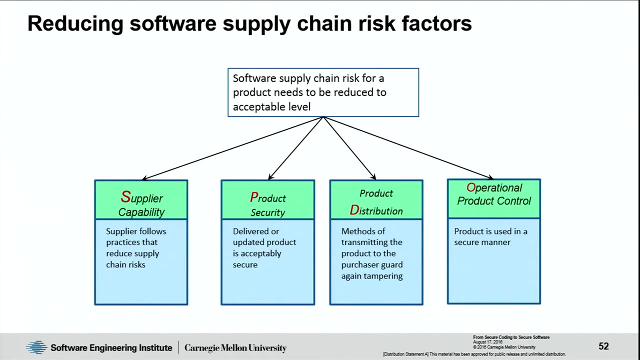 26%- A quarter of the most open source components have high risk vulnerabilities. If you're using Spring, you probably are one of these people. How to do that? How to reduce this? Well, by managing your software supply chain, and the methodology we use is called Speedo. 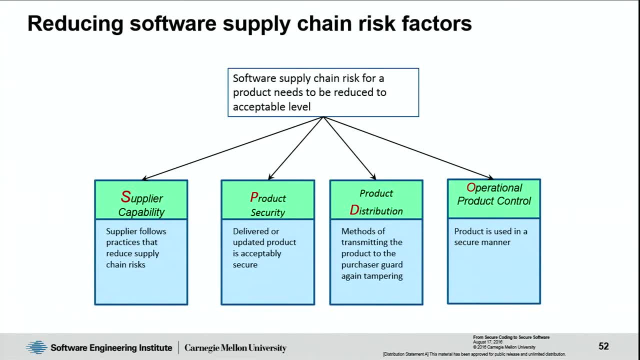 S-P-D-O. Very minimal methodology, if you'd like to remember it that way, Making sure your supplier knows how to do secure coding, that the product was built correctly, that it wasn't modified too much, that it's right in distribution. 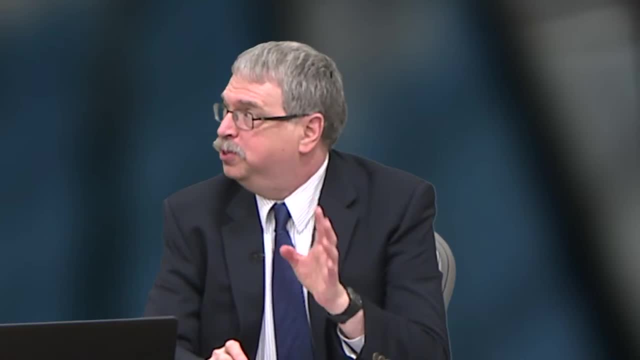 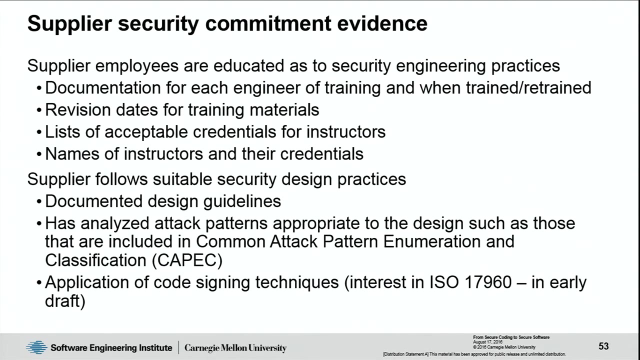 and that it's in the right operational context. Now, for each of these, we have specific recommendations that you can follow for supplier evidence: Do they really know what they're doing? And again, you can look at the details on replay. Similarly, how do we evaluate a product that you're getting? 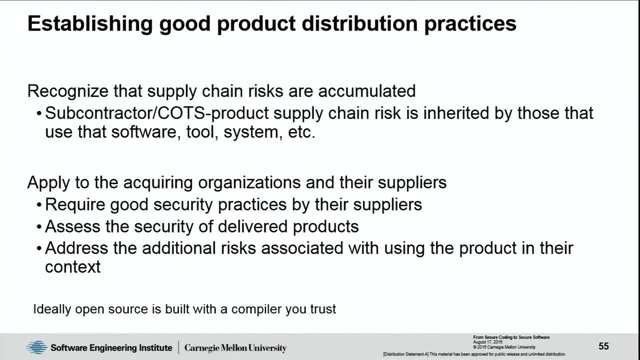 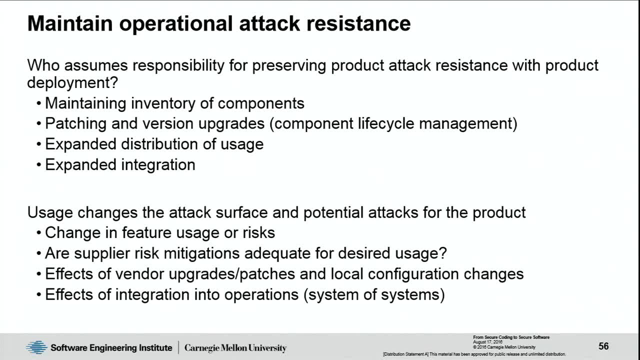 whether it's been properly put together or not. How do you know that it has been distributed in a way that hasn't changed along the way And, perhaps most importantly, that you haven't changed the operational environment? Most of the problems that we see in large systems. 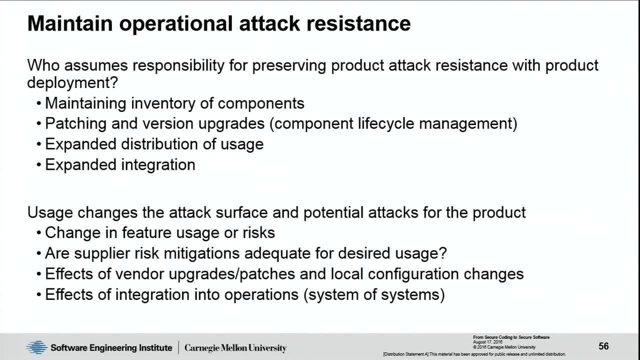 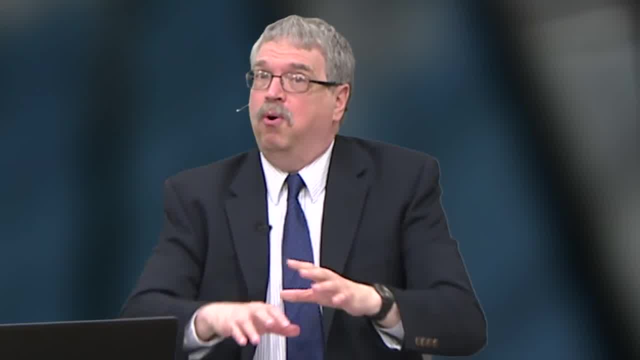 have the consequence that they were built under one set of security assumptions, put into a different environment and they've changed the security assumptions. So we said an awful lot of things you can do And you might say: well, what should I go after? first, 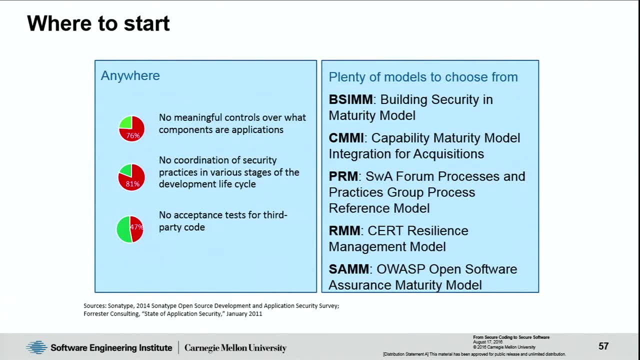 The unfortunate truth is that there is so much to do that you can pretty much start anywhere. On the left, you can see that the large fractions of people who basically have huge security gaps in their development processes- And there are lots of ways to do this- 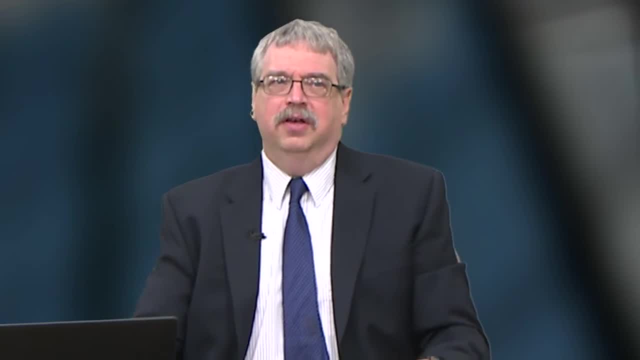 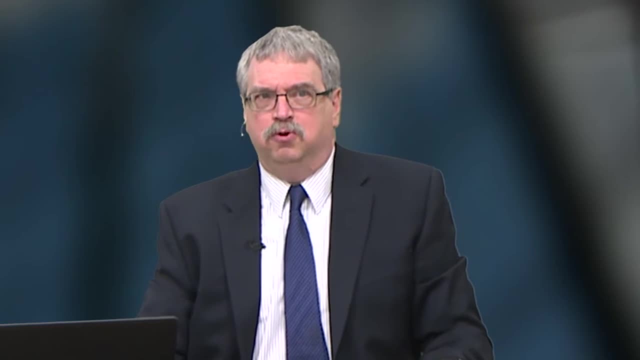 And on the right we list a variety of choices that you can use, depending on if you like us. you can use things like RMM- come from CERT. If you like what Citigrall does, you can use BSIM, But there are many alternatives. 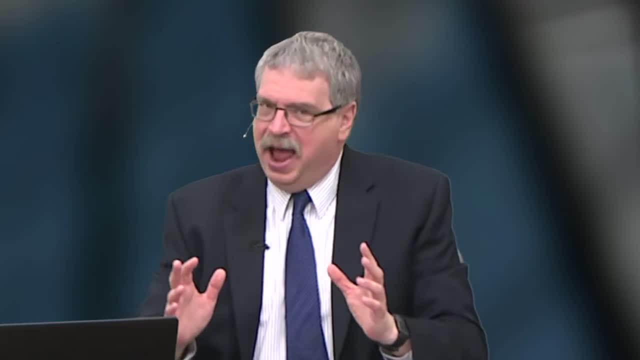 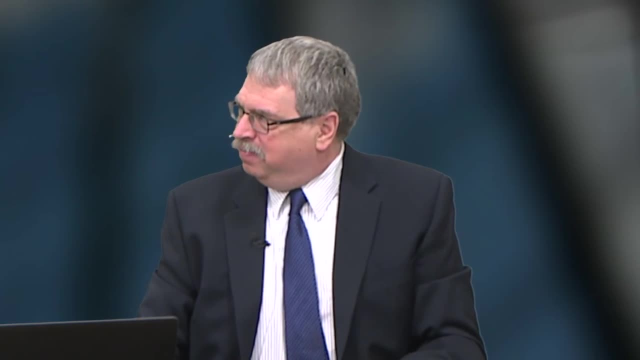 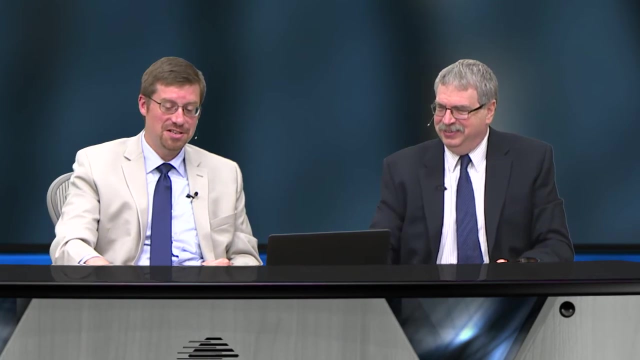 Each one has their pluses or minuses, but there's such a gap that pick one and use it as you would like. With that, I'm going to let Bob close here. Sure Thanks, Mark, And sorry for well. thank you for doing a good job. 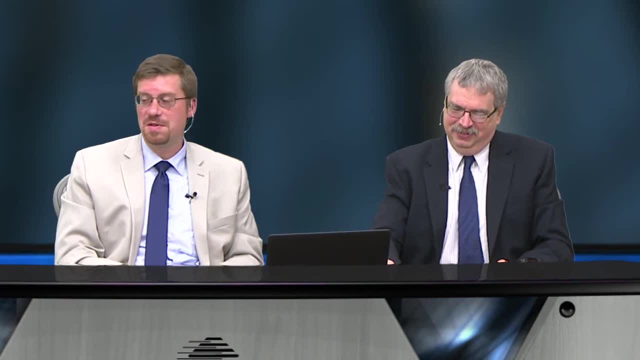 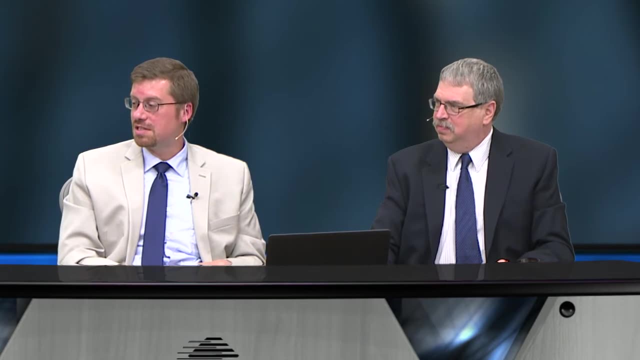 of kind of getting through that. Sorry to the audience for him having to do that. If you have questions, please let us know and we'll be sure to follow up With that. that pretty much closes, except for questions. There's two things I wanted to say really quickly. 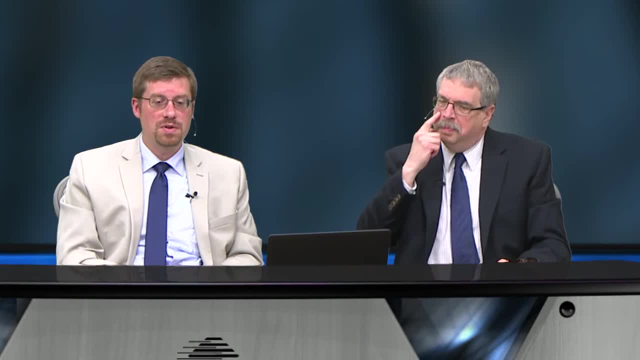 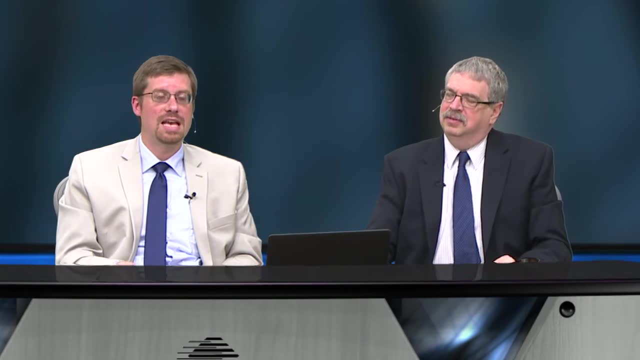 One was that: where are we going with research? Just quickly, we're looking at ways to use machine learning to improve the accuracy of static analysis tools. in particular, Can we use the data of what we found with diagnostics that are either true, positive or false positives? 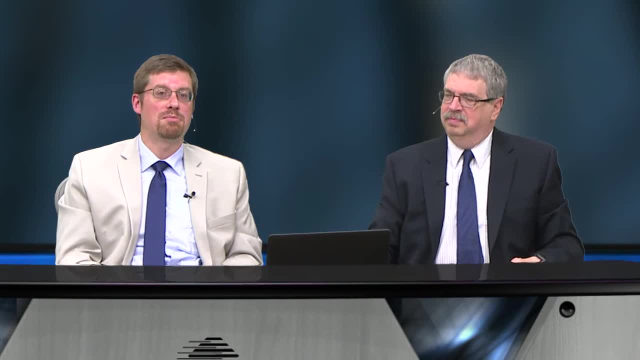 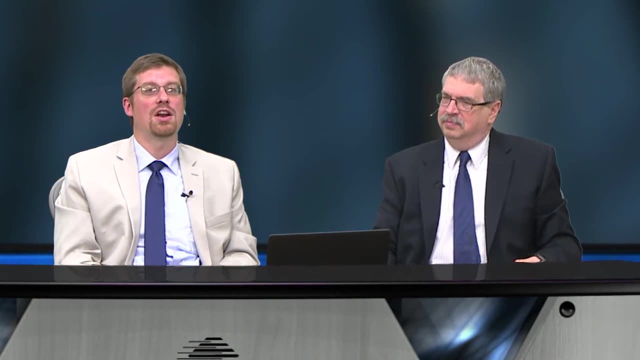 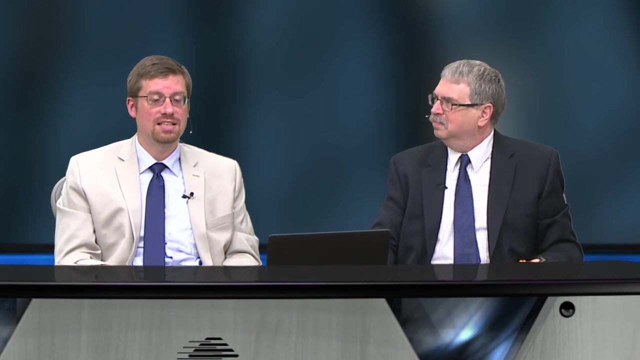 and use other information to improve our prediction of whether or not it's a true positive or false positive, and something to pay attention to, as well as working on automatically correcting code. finding code that you know an analyzer might find is a diagnostic. 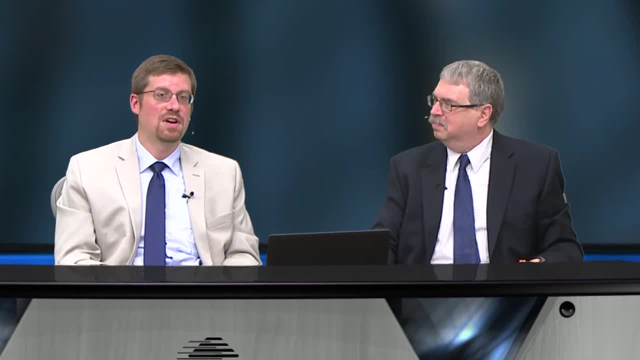 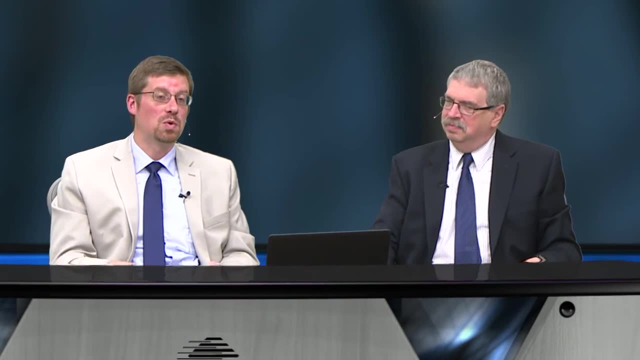 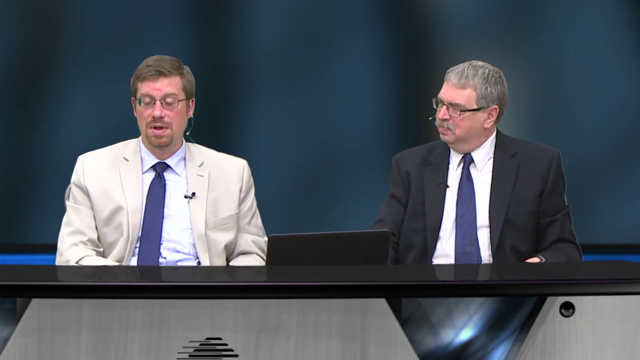 but that we feel we're pretty sure that it is a defect and informing the developer on the spot what could be done to correct the defect. or for code that is out in the wire, just fixing the code with, you know, near perfect or perfect accuracy to not cause any problems. 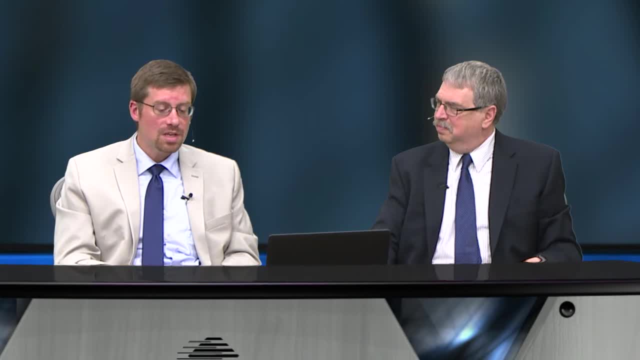 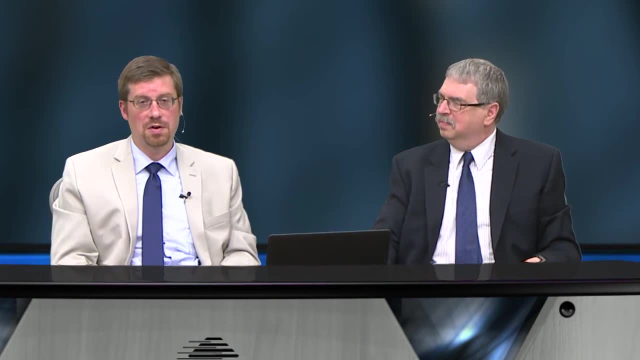 The last thing I wanted to mention was that we do have a secure coding symposium coming up. if you're looking for more information about secure coding, both from the SEI and from the community, On September 8th we'll be in Arlington, Virginia. 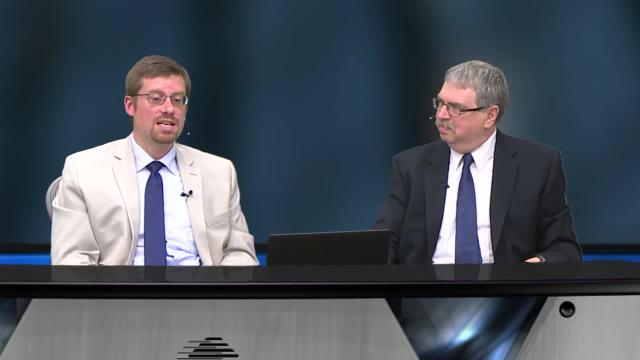 at the secure coding symposium, Largely the day. it's a one-day event. It will be a few keynotes and several panel discussions and then a tutorial. The panels, the keynotes will be outside, the outputs will be outside speakers. 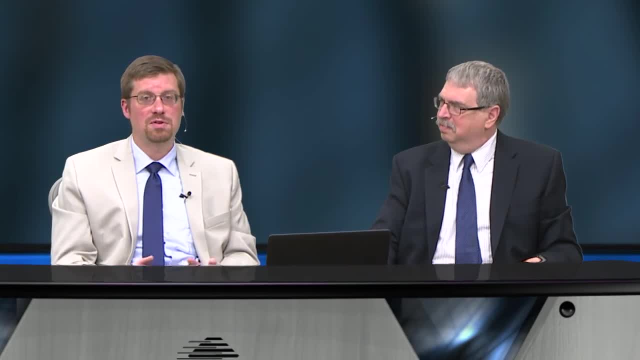 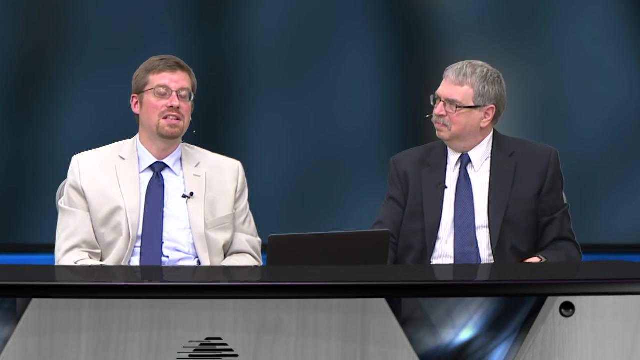 The panels will be a mix of SEI and outside speakers from government and industry, And we'll end with a tutorial And the registration page is already available and I believe it's in your resources area. There's a general agenda listed as well, and we're going to be updating that within the next couple days. 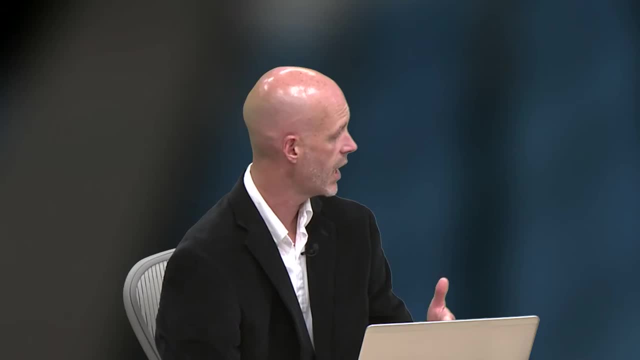 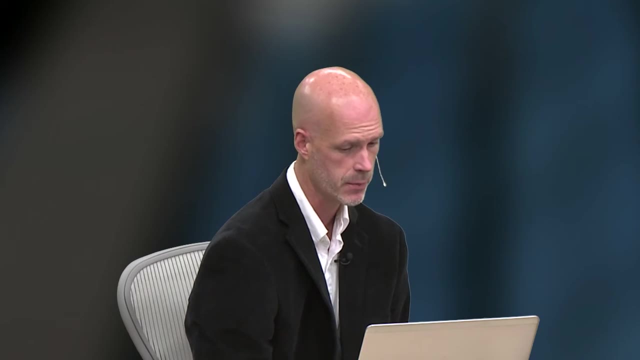 with the names of the speakers and the presenters. And I'll just add: there's no cost to attend that. but space is limited and a lot of space is already taken up. That is correct. If you have interest, click on the link in the resource tab. 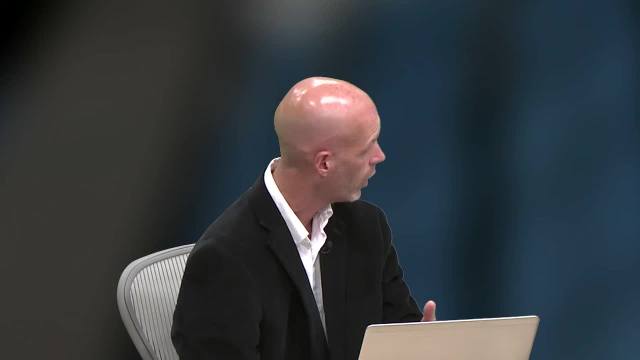 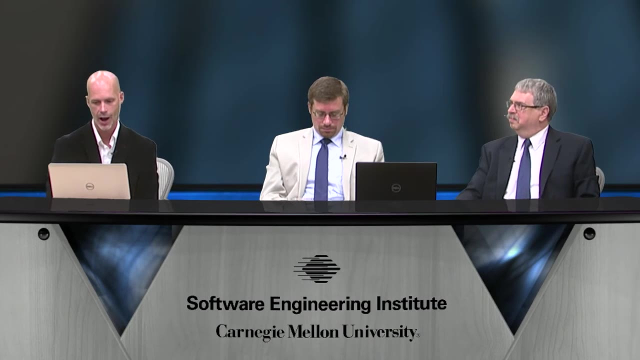 So we know it is 2.30, so if you have to go, we understand. But I'd like to just get one question before we wrap up, And that's from Brian asking: would you agree that turning up compiler warnings to a high level, eg W4,? 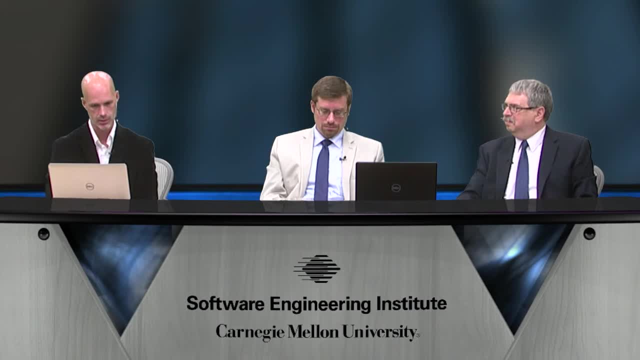 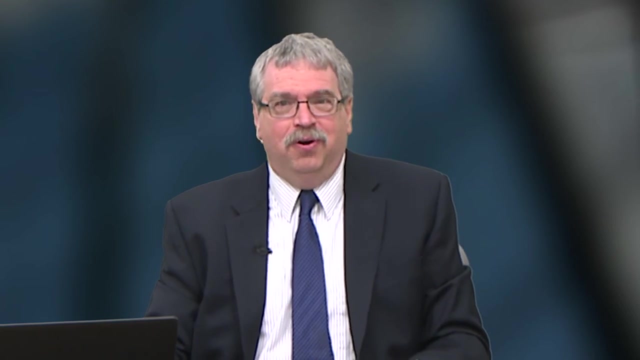 should be a priority to secure a legacy code base. It depends who you ask. This goes back to the false positive comment that it will definitely increase the number of diagnostics that get generated, and the question becomes: at what point do your developers start ignoring all the diagnostics? 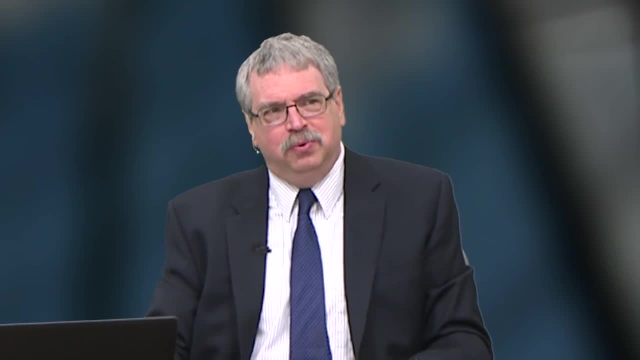 We've gotten stories from people like place development organizations, like Google, who tell us that if they put out any false diagnostics, the developers revolt and they can't put them out at all. Other places are far more rigid and say: you've got to address every single diagnostic.